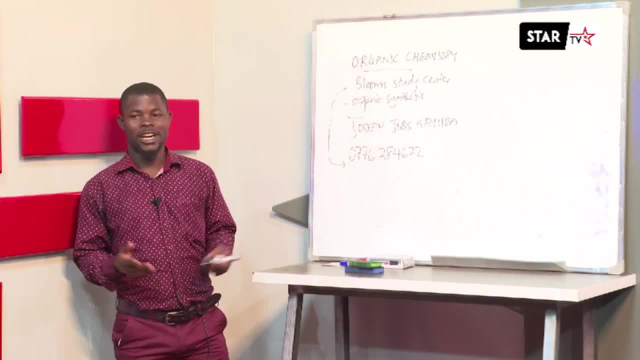 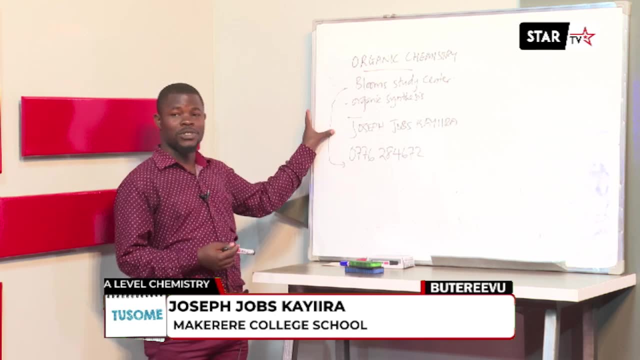 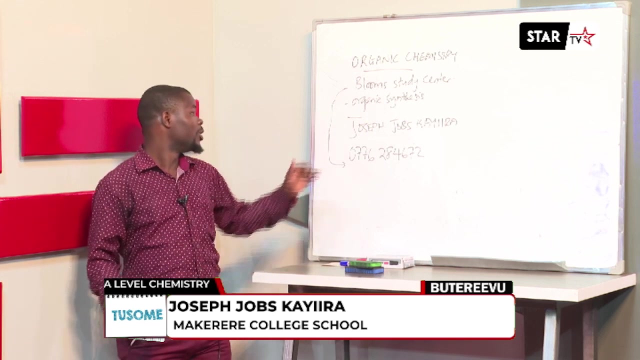 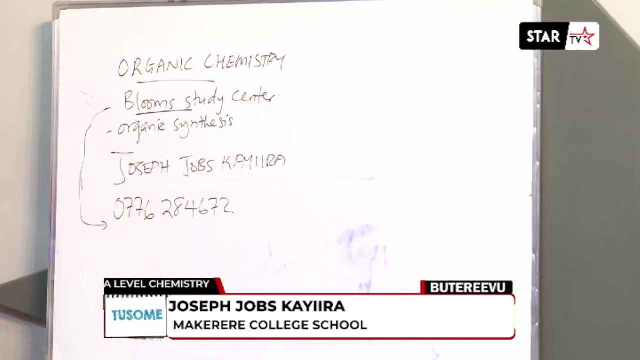 Yes, you're welcome. dear viewers, We are back here to our presentation. I'm Joseph Jobs-Kaira and I'm here for Organic Chemistry. I'll be taking you through organic synthetics. It is Bloom Study Center and UBC Star TV bringing you this good program. 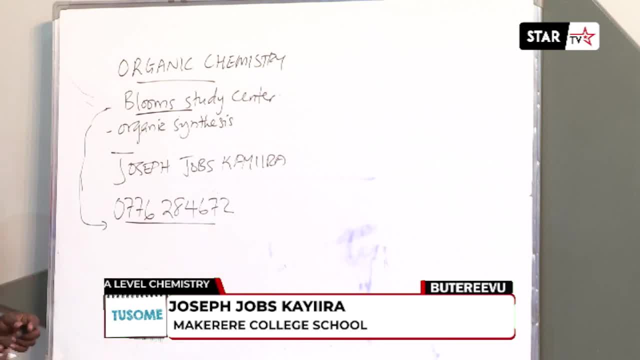 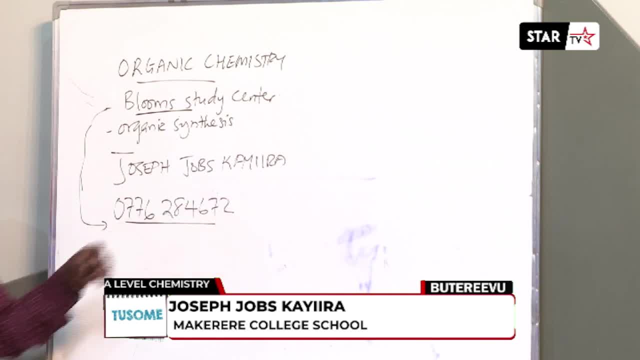 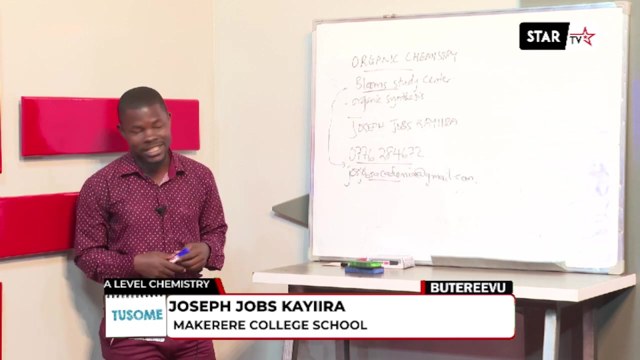 Personally. you may contact me at Joe's Jobs Academia at gmailcom. Now we are here for our simplest branch of chemistry that most of the students- are already students- enjoy. But before I proceed, remember, dear viewers, that COVID-19 kills. I've already 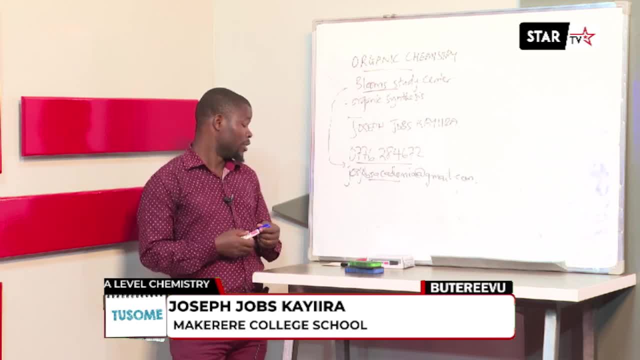 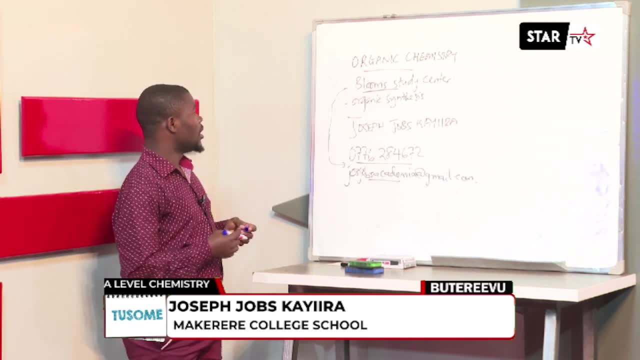 got my two doses and I'm well to go. Please go to the nearby vaccination center and get vaccinated. I'll be using this board and also our PowerPoint presentation for this lesson. Let's have the first slide and then we'll be well to go. 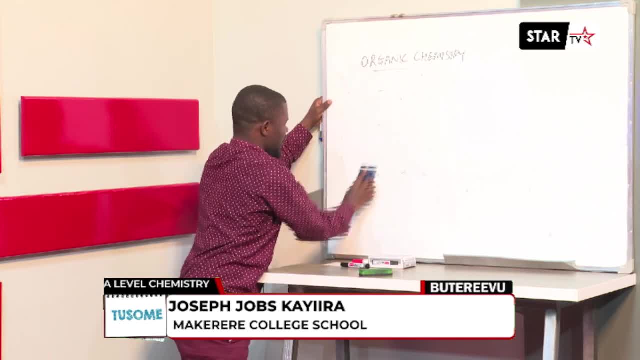 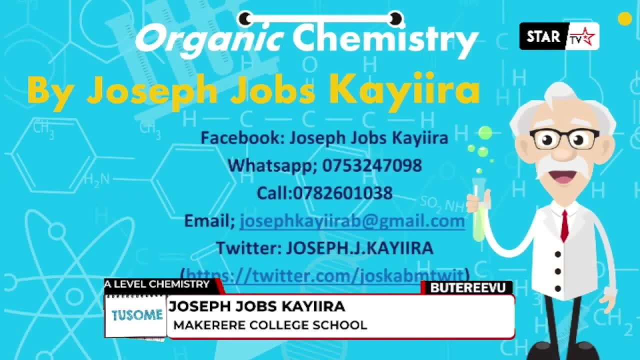 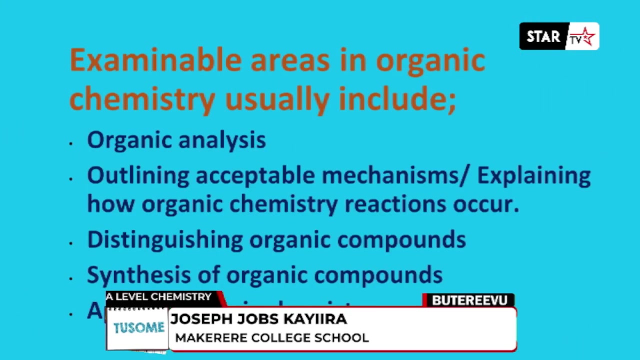 When you look at your TV screen, you see that slide showing you organic chemistry. You see that slide showing you organic chemistry. Sorry for that interruption. My contacts are there. Let's proceed to the next slide. In our next slide we are showing you our examinable areas in organic chemistry. 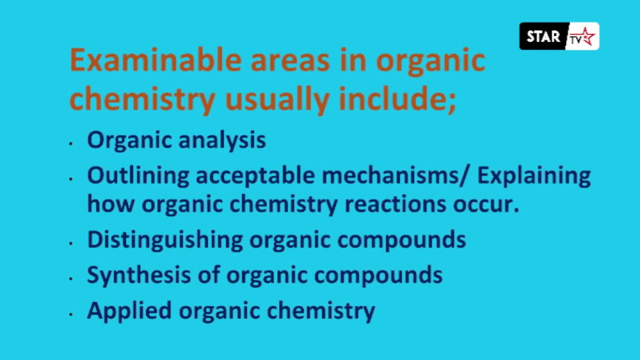 We are showing you our program, our examinable areas in organic chemistry. We are looking at organic analysis, how to outline mechanisms distinguishing organic compounds, synthesis of organic compounds and applied chemistry. But I'll be looking at mainly that fourth section that you're seeing on your screen. 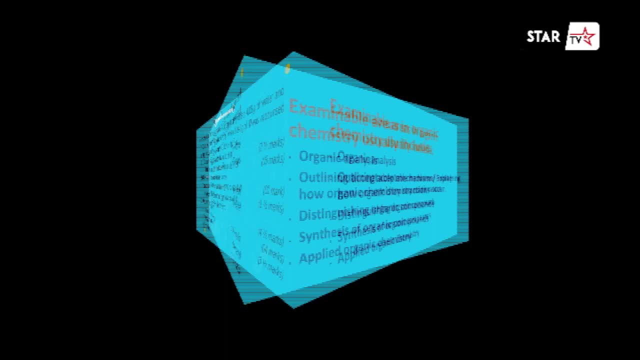 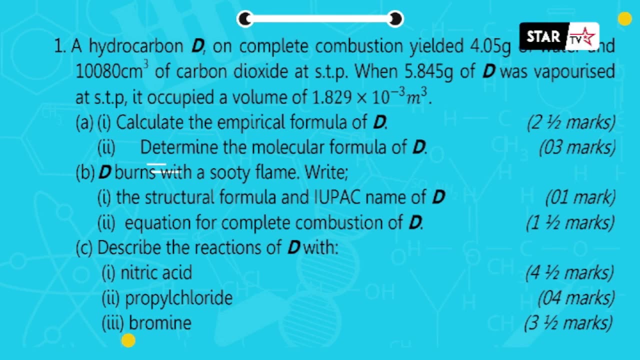 the synthesis of organic compounds. Our next slide, That question you see on your screen, is a question that is an example of what we deal with in organic analysis, But it's not our aim today. We shall look at that in our next session. Next slide: That is a question about mechanisms. 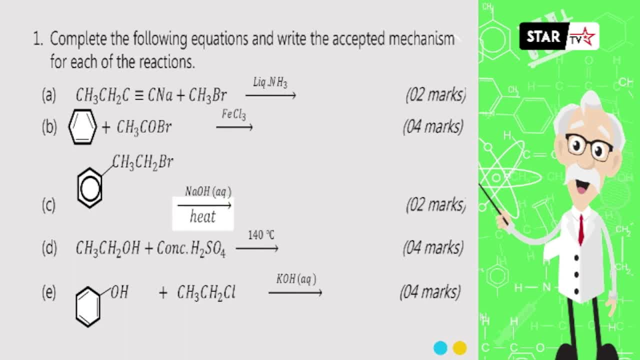 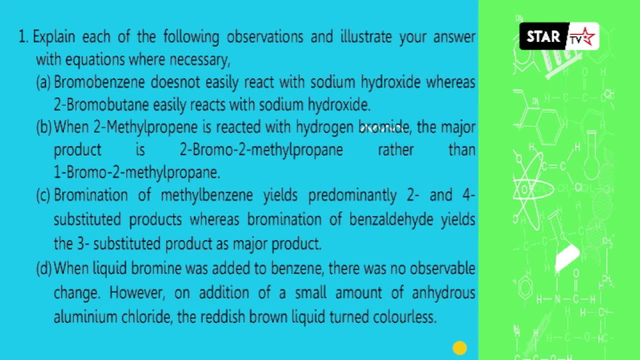 Complete the equation and then outline a mechanism That will also be for another time, Then next slide. That is a question. that is a general question that involves explanation of observations and how to illustrate your answer with equations where necessary. Such questions examiners are very much interested in them these days. 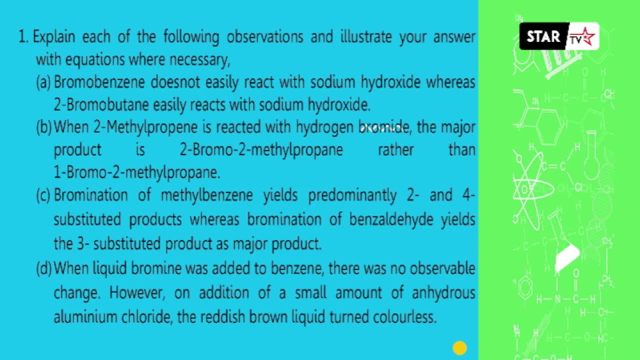 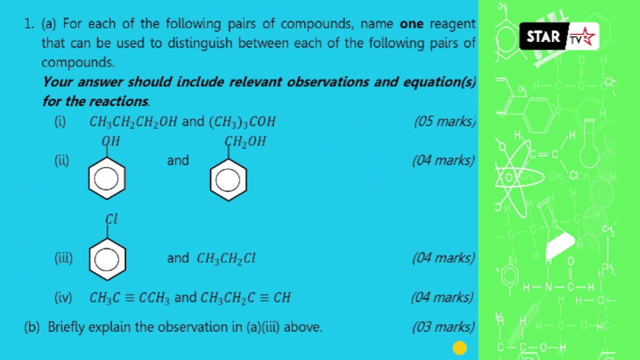 So when you look and approach such a question you should always be very careful. Next slide that question. there is also a good question where you are asked to identify a reagent that can distinguish compounds. examiners are very much interested these days in observations. 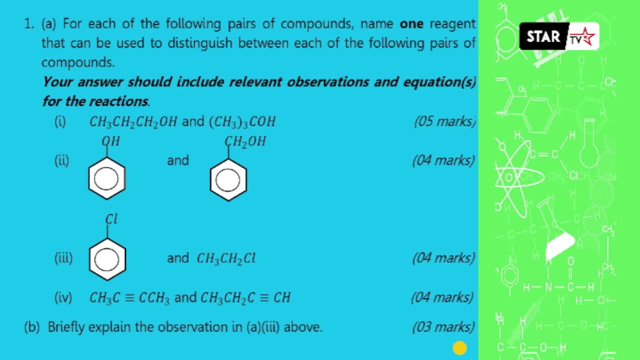 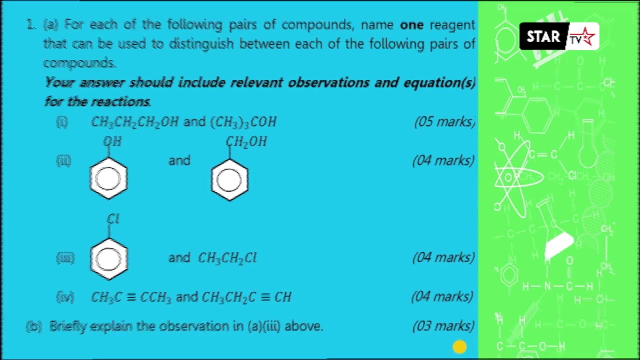 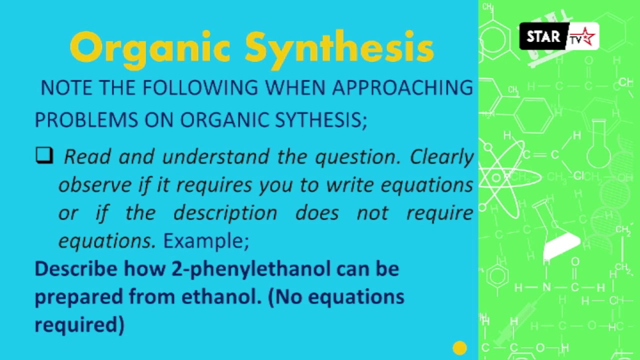 and equations for the reactions at the end of the after you've given the observations, you've stated the reagent, you should also be well conversant. without right, balanced equations for the reactions, we proceed now. our aim today is that organic synthesis you're seeing there and what should you note? 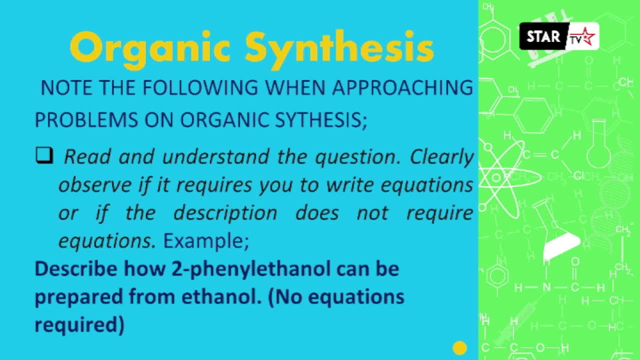 during organic synthesis. during organic synthesis. dear viewers, I want you to note the following. the first one is that read and understand the question. observe if it requires you to write equations or if the description does not require equations. we have our first question there. it says: describe how. 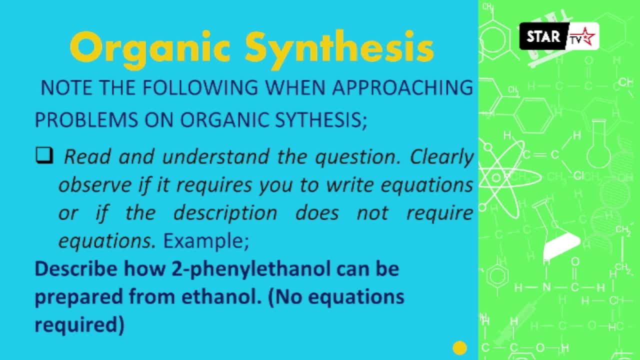 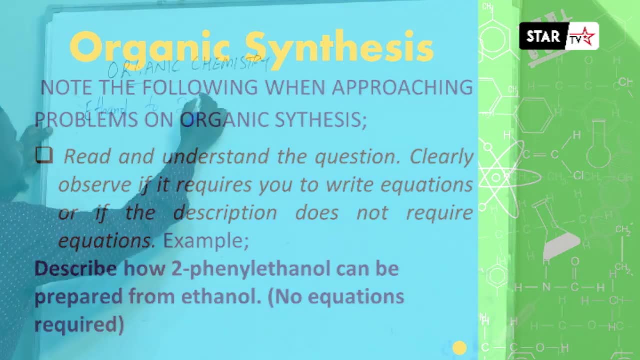 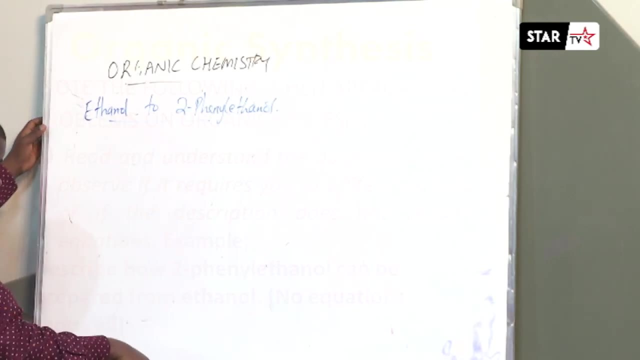 two phenyl ethanol can be prepared from ethanol. in other words, we are converting ethanol to two phenyl ethanol. the question is very clear. no equations are required. you're told not to include equations in your answer. so what do you do? try to do some side work. 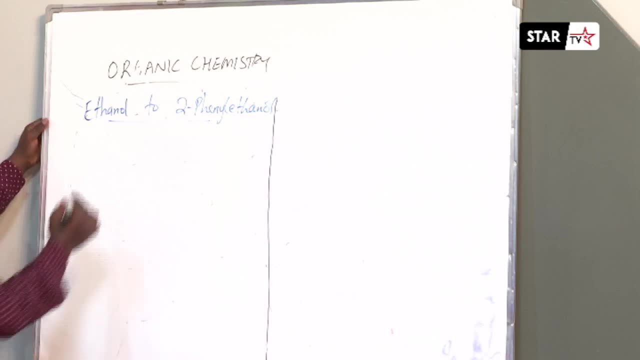 you cannot approach this question directly. this question was set in last year's paper two and most of the students misfired. they had to go on and write equations and they lost 20 marks. they were working out of 18 for paper two. what do you do? 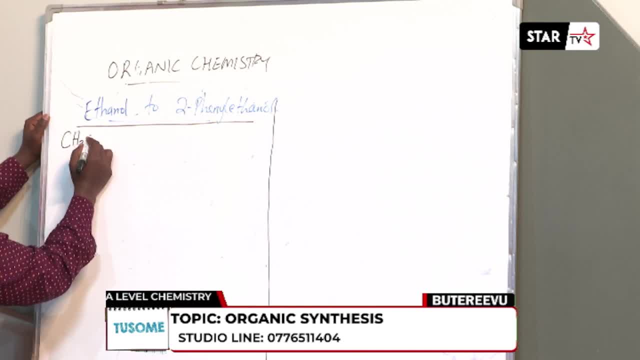 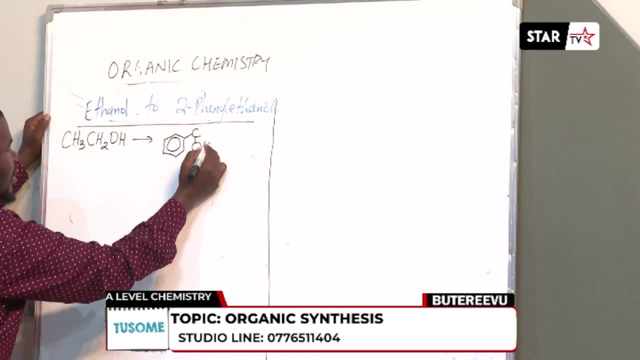 write the formula of the compound you want to convert to the other. this is ethanol. you want to convert it to two phenyl ethanol. you want to convert it to two phenyl ethanol. so you should, very much you should, be aware of the nomenclature of these compounds. 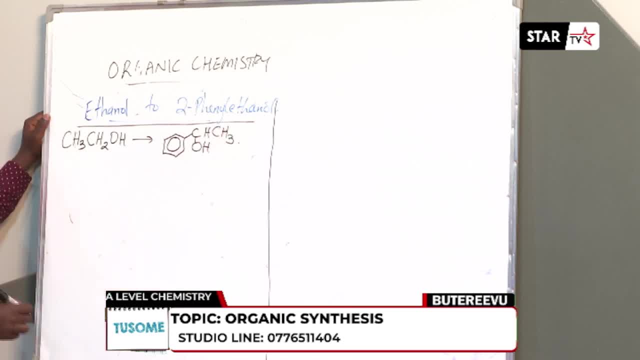 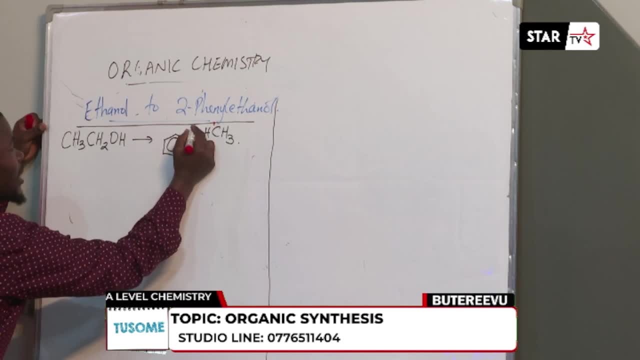 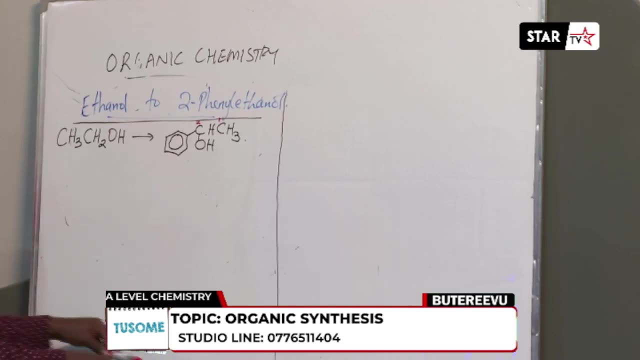 so this compound here is what you call two phenyl ethanol. this is carbon number one and this is our carbon number two. this is your carbon one, that's your carbon two. that's why we call it two phenyl ethanol. okay, um, I'm sorry, I have to make a correction here. 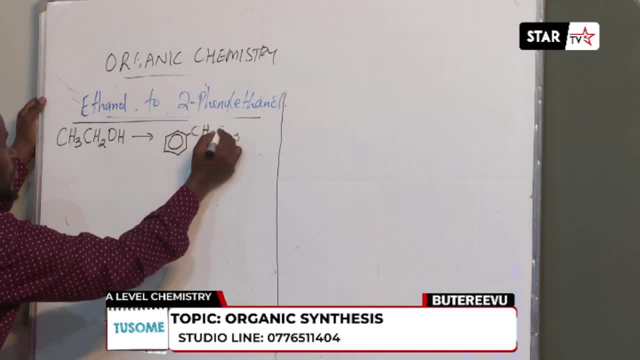 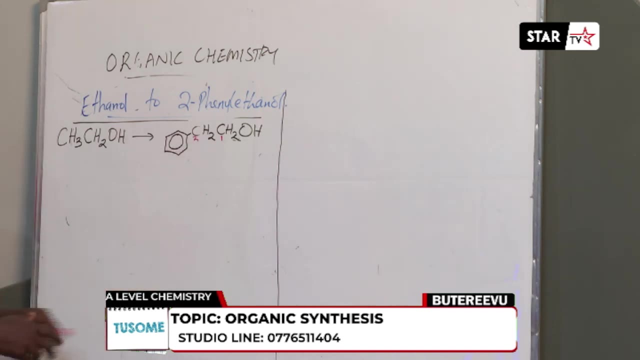 for two, phenyl ethanol. this should be ch2, ch2. oh, this would be your carbon number one. the carbon that has the OH group is carbon number one, and then the carbon that has the phenyl group becomes carbon number two. you count the carbon atoms depending on. 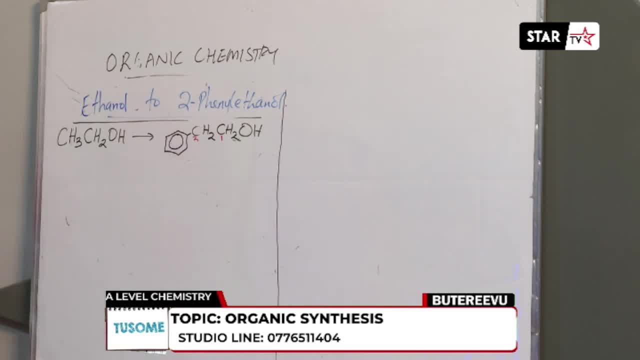 the hydroxyl group. so what do you do? what you should you do is very simple. First of all, try to do the synthesis using equations as side work. So this one will first of all be converted to a benzene ring. and to get the benzene ring, you must of course get ethanol, you must get ethylene first. How do you convert ethanol to ethylene? You proceed through ethene by first of all dehydrating the ethanol at 180 degrees Celsius. This gives you ethene. Then add bromine in the presence of carbon tetrachloride. This gives you CH2Br. 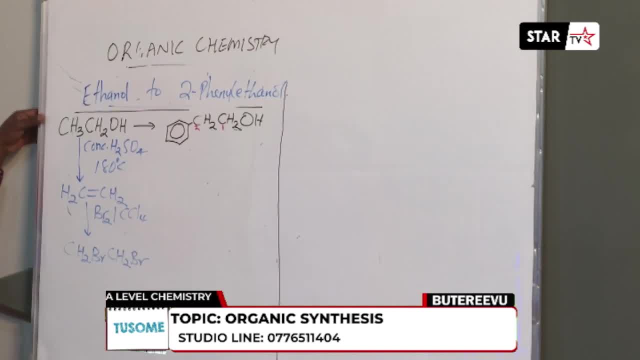 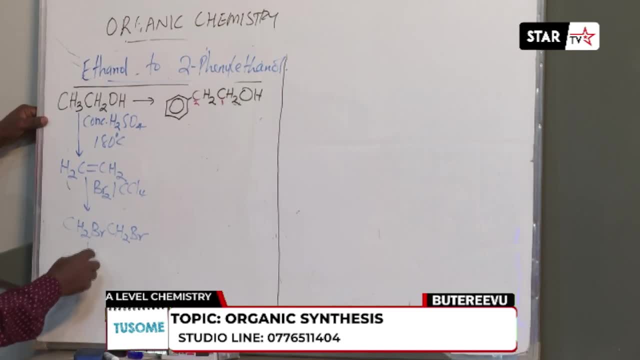 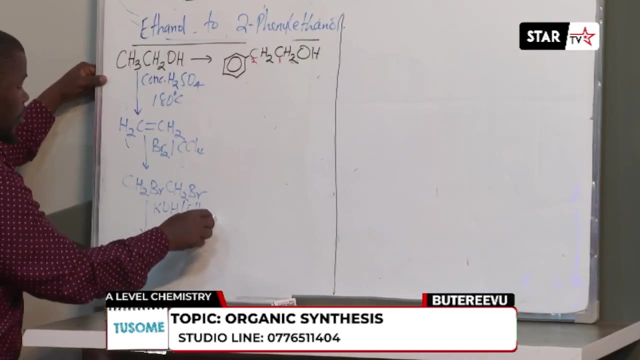 CH2Br. I hope our viewers from the West Entire High School you are very much following. Now this one here can be converted to ethanol by using a benzene ring, And this one here can be converted to ethylene by using potassium hydroxide. 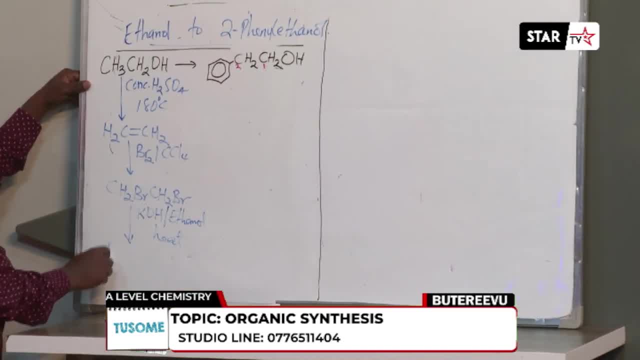 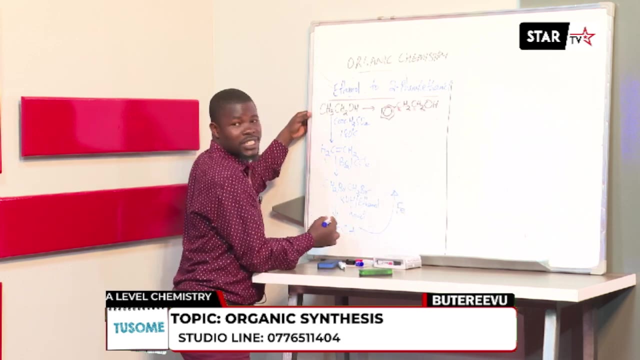 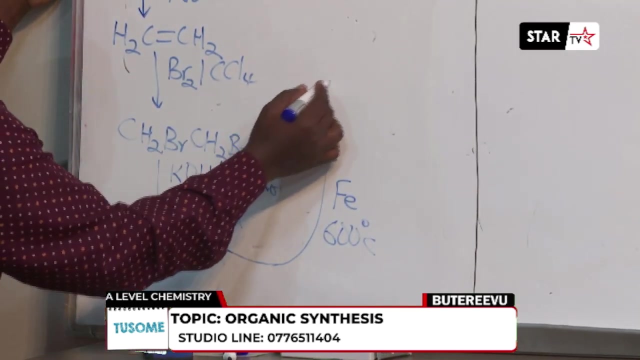 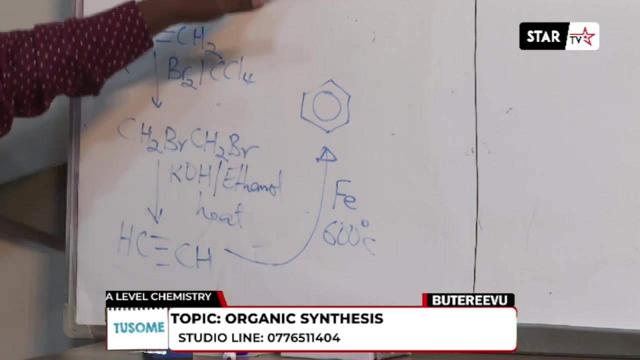 ethanol and then heat. This will give you ethylene. That is, your ethylene. Now ethylene can be converted to benzene using iron tubes or copper tubes and you heat, at a temperature of about 600 degrees Celsius, the benzene, and now they are well to go. How do you get from benzene to this? 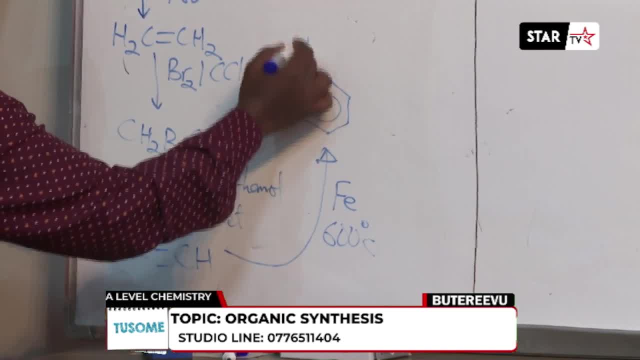 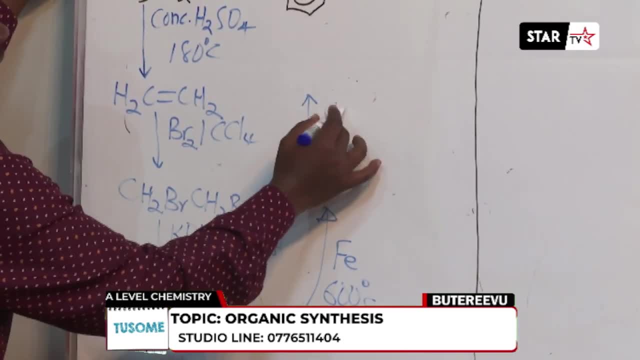 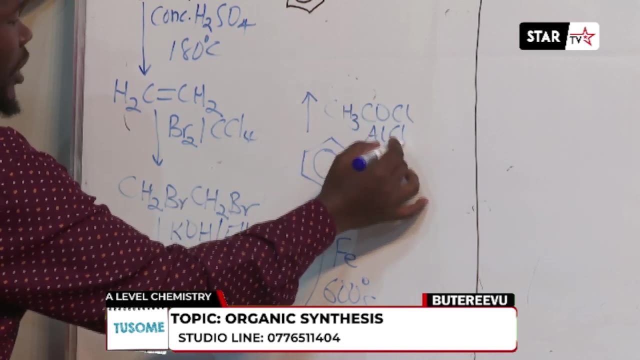 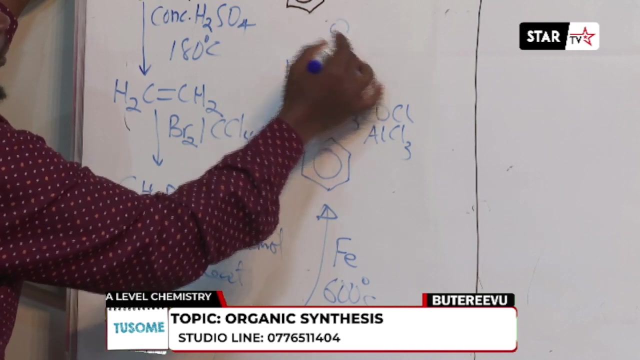 compound. To get to that compound you must get, you must do acylation, Friedhoff-Raffut acylation. So to do that I add that reagent in the presence of aluminium chloride. That gives me phenylethanone. Now I want to convert. 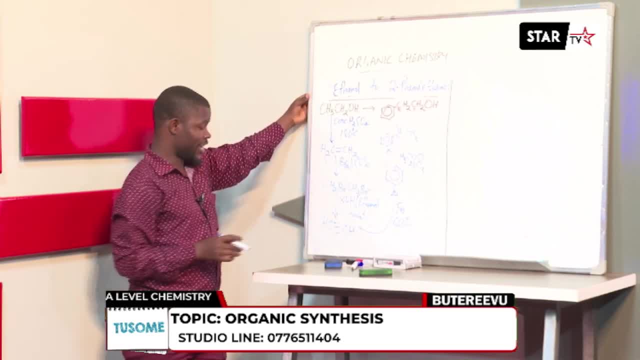 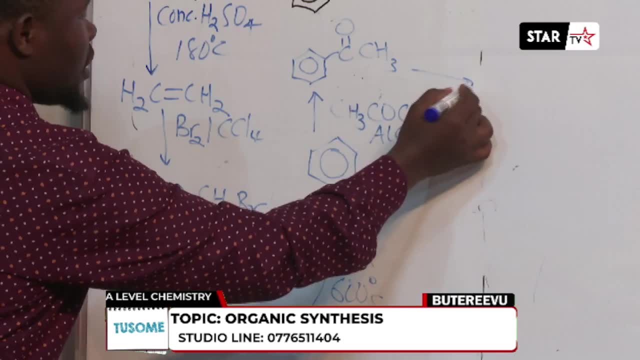 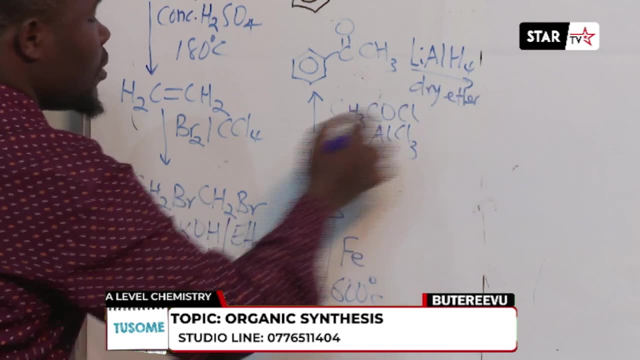 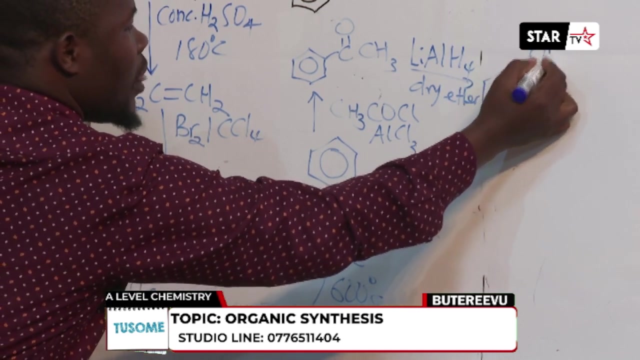 phenylethanone to that compound. I still have a journey to travel, So what do I do? I can now reduce this using lithium, aluminium tetrahydride in presence of dry ether, So it gives me this compound here, A secondary alcohol which I now want to. 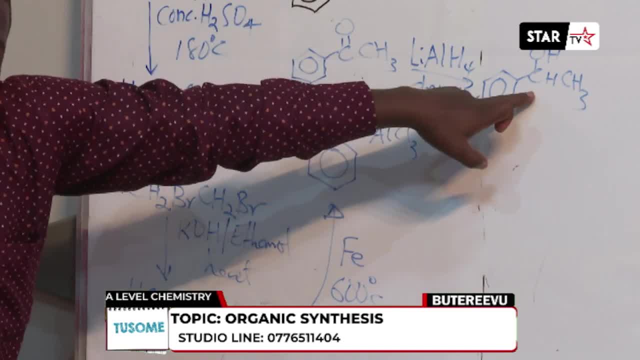 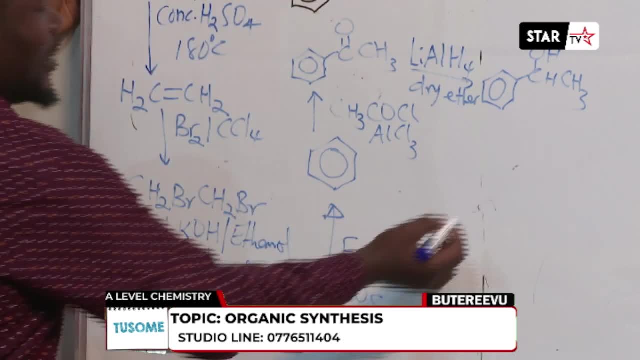 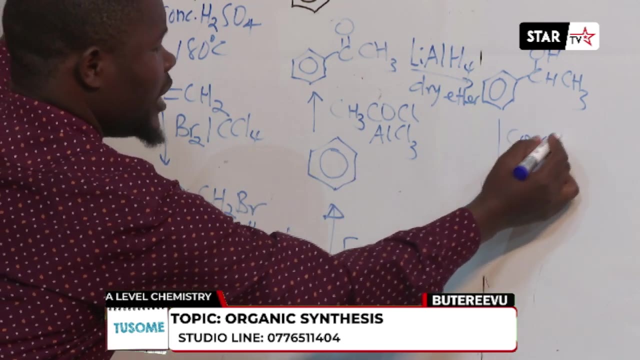 convert to a primary alcohol. This one is one phenyl ethanol- One phenyl ethanol. This is two phenyl ethanol. So what do I do to this? Finally, I can dehydrate using corn sulfuric acid- Atroxyl sulfuric acid. 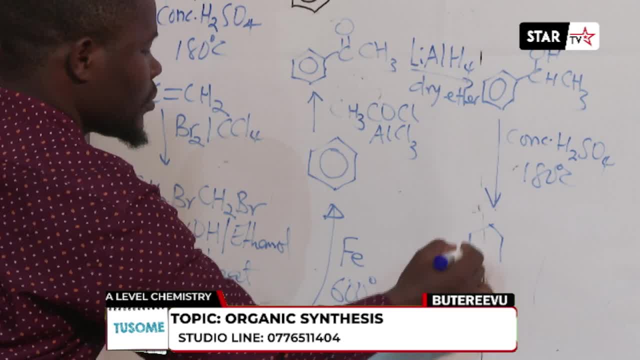 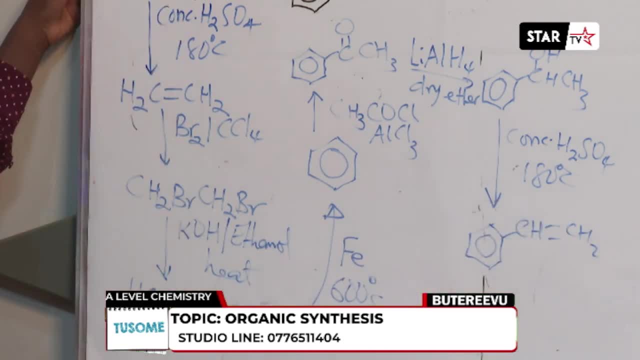 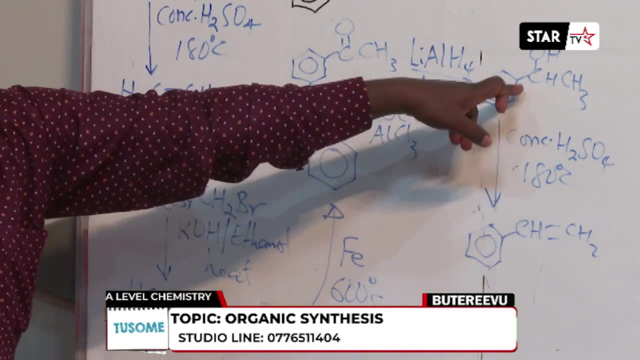 Atroxyl sulfuric acid At 180 degrees Celsius to give me phenyl ethane. To give me phenyl ethane. Now, some students would add acidified water here. When you add acidified water, you're coming back to two phenyl ethanol, which we are not aiming at. So how do you? 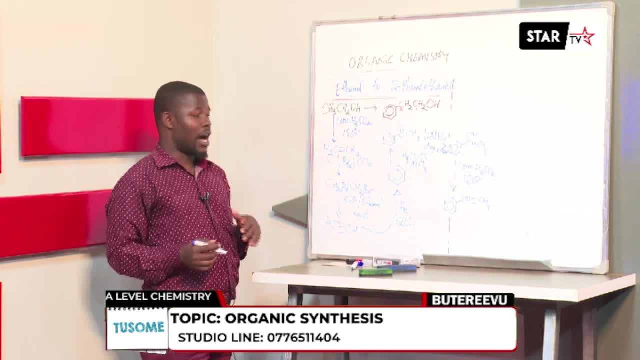 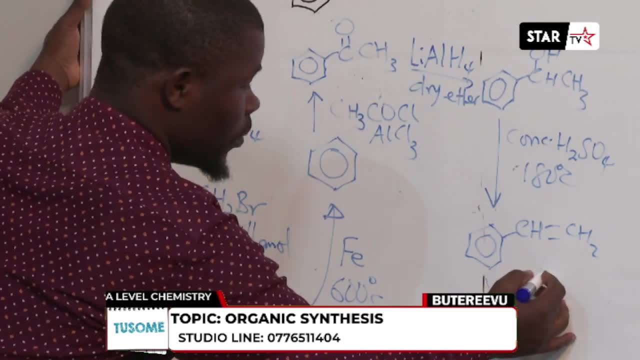 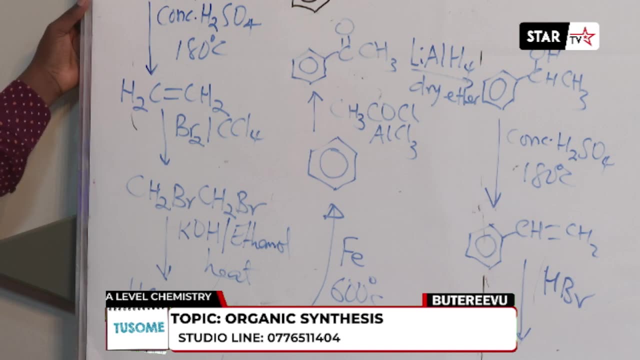 avoid that You can use Makonikoff's rule and look at the other side of the it, which is antimakonikoff. So when you use Makonikoff's rule and you add hydrogen bromide here, it is the carbon atom that has excess hydrogen atoms that will get the hydrogen. 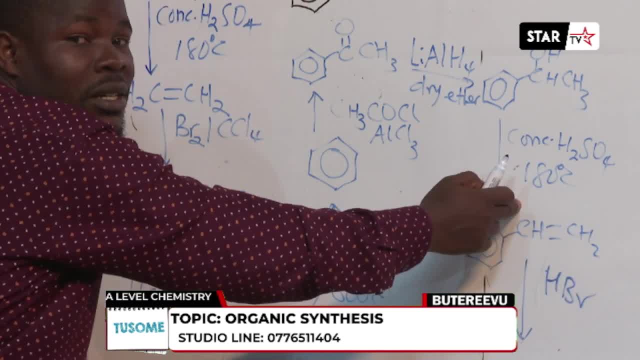 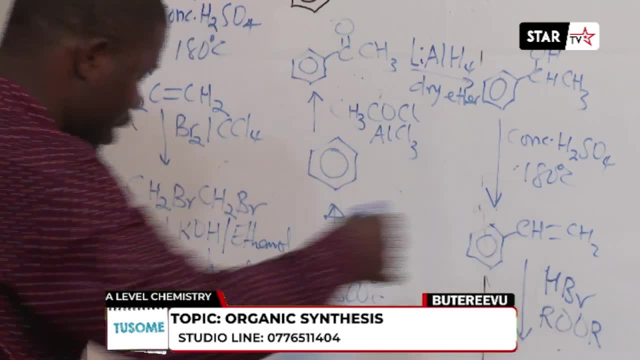 This hydrogen will come here and then the bromine comes here, So that will not help us. How do you avoid it? Let's use hydrogen peroxide, hydrogen bromide, in presence of an organic peroxide and proceed via the antimakonikoff's rule. 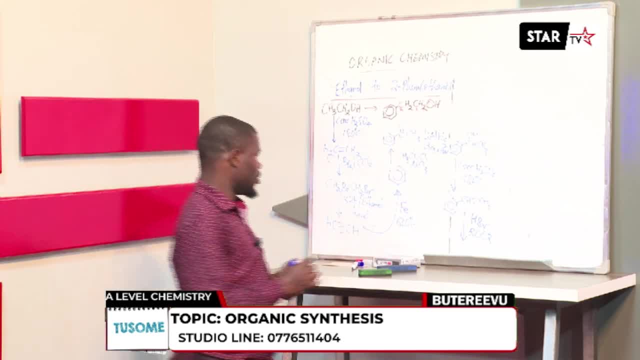 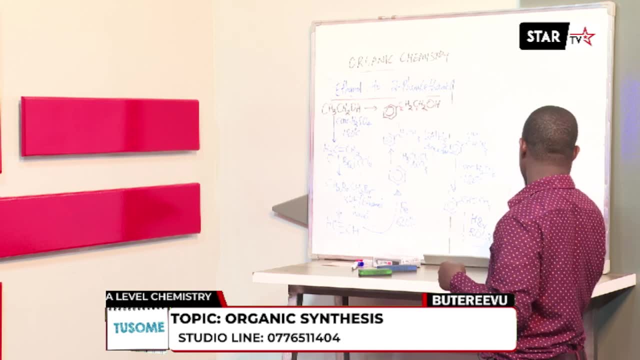 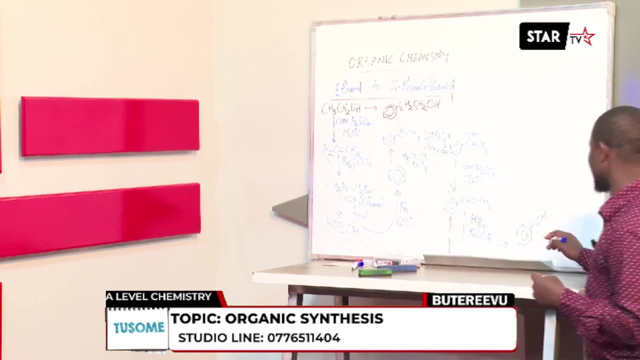 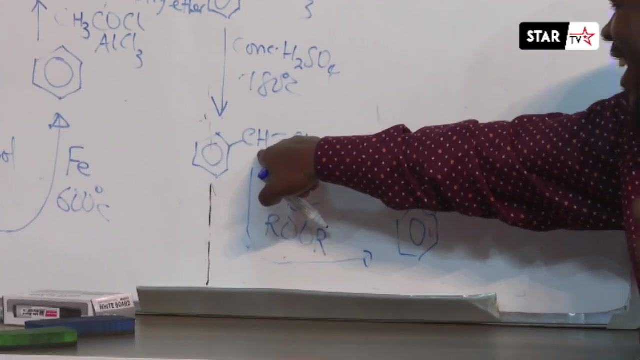 Now, when you do that, you're going to get this compound here. You're going to get the compound CH. You're going to get this compound here. The hydrogen is going to come here to the carbon that has less hydrogens, and the bromine will come here. 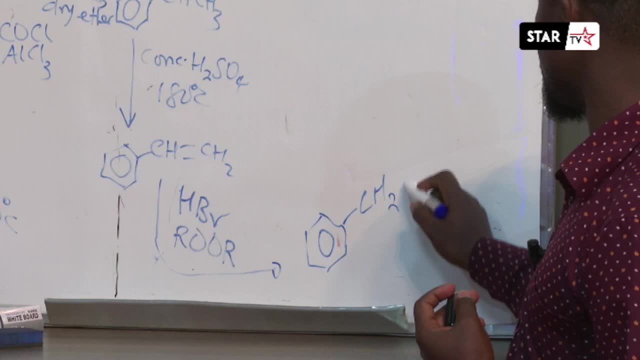 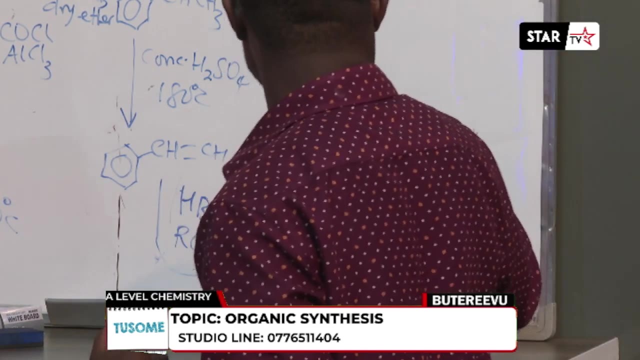 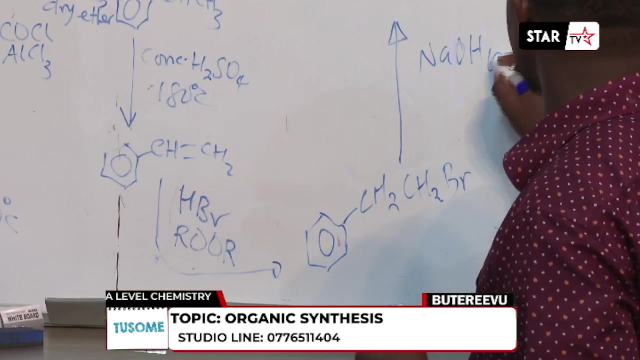 That's antimakonikoff. So now you'll have CH2, then CH2Br. From this point you can go direct to your final product by using sodium hydroxide. The sodium hydroxide should be aqueous. It should be aqueous. 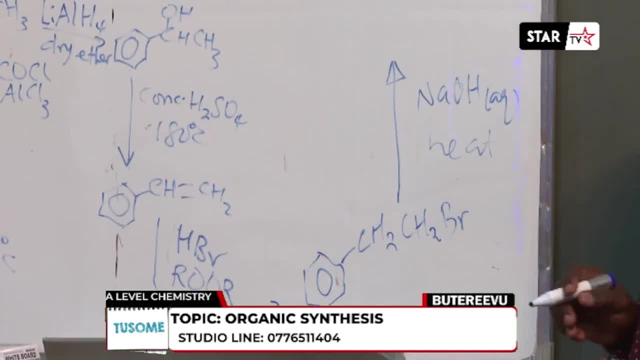 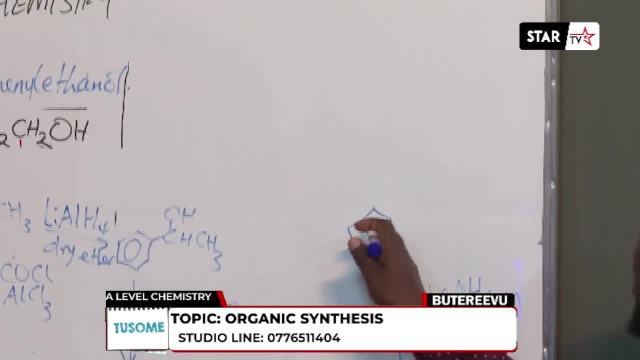 and then you should heat. When you heat, you'll finally come up with your final product, which is 2-phenyl-3-hydroxide. And then the blue is the ethanol, If you didn't know the IUPAC name of that compound. 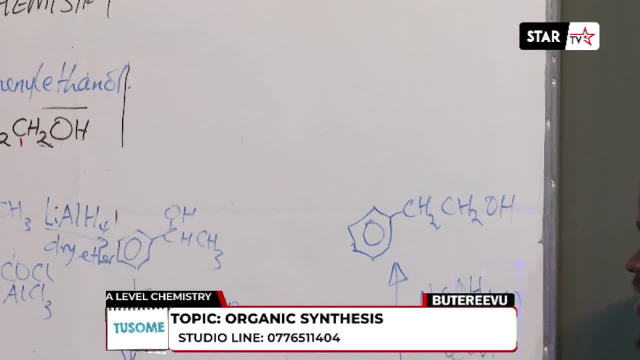 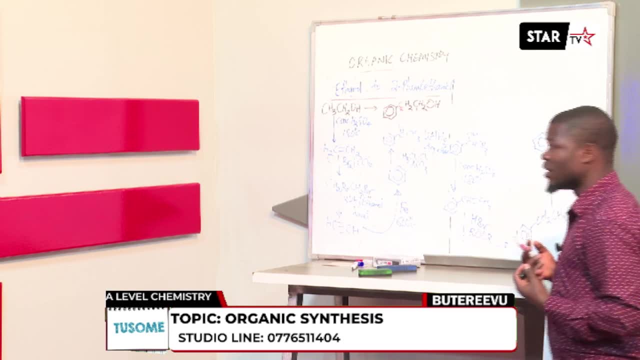 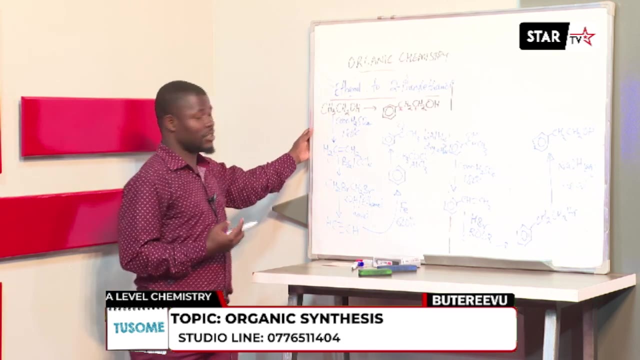 you could not get it. It's a bit lengthy synthesis and now we want to see how do you convert this to words. How do you make these words? So, to make these words, you come here and try to write. You have your books, you're now writing. How do you convert ethanol to? 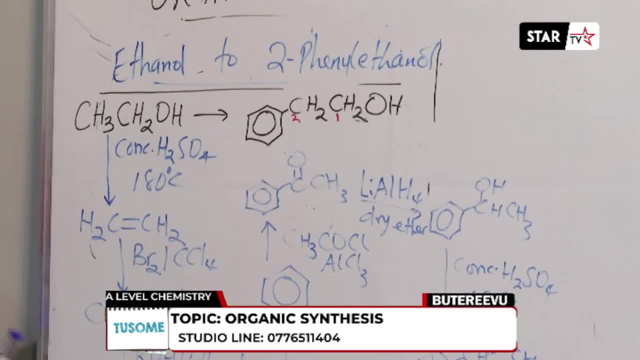 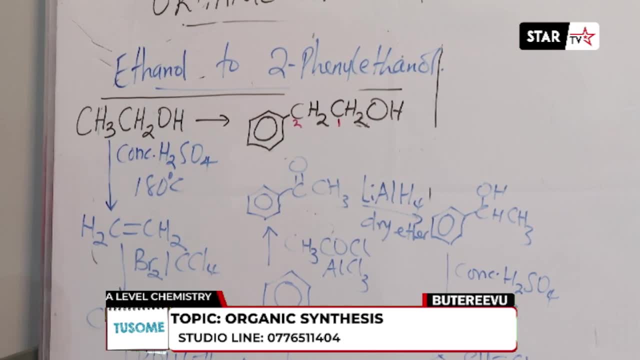 phenyl ethanol is side work. remember, in our slide they told us no equations were required. so, dear viewers, especially those from the north, what will you say? you'll come and say that ethanol is heated at 180 degrees celsius with concentrated sulfuric acid, actually, with excess concentrated sulfuric. 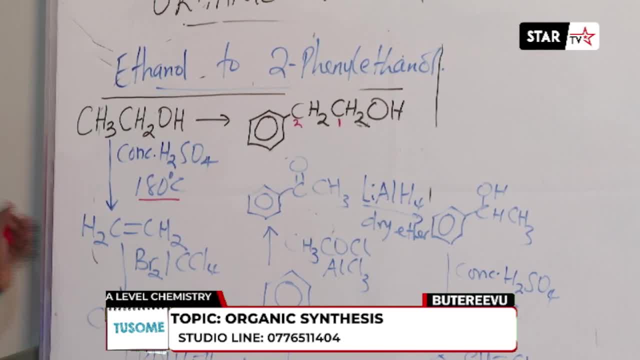 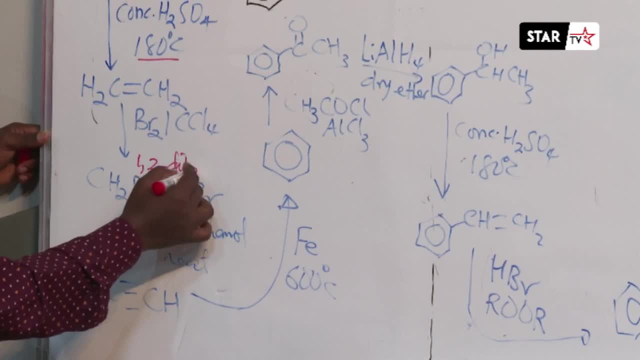 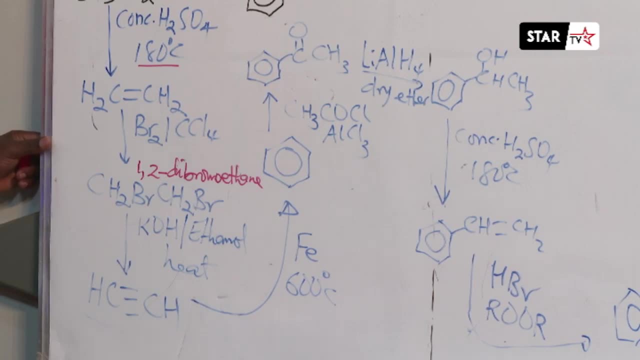 acid to form ethene. ethene is reacted with the bromine importance of carbon tetrachloride to form one, two hyphen dibromo ethane. so if you don't know the names of these compounds, you cannot do this. then the one two, dibromoethane is reacted with alcoholic potassium hydroxide. 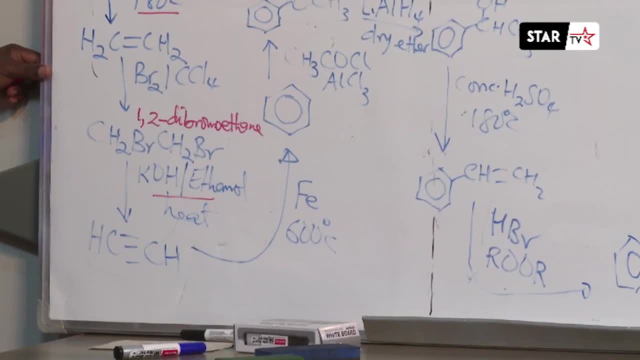 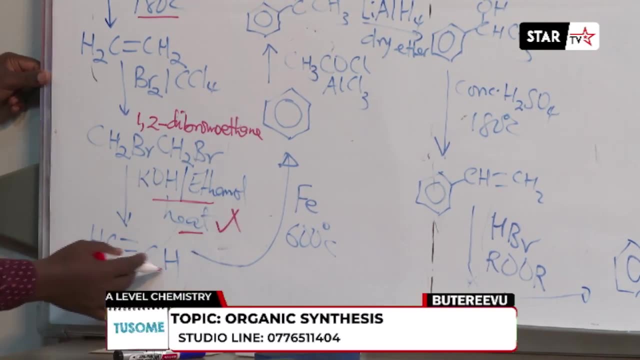 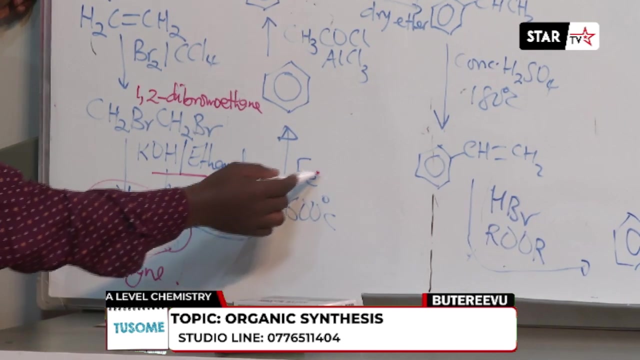 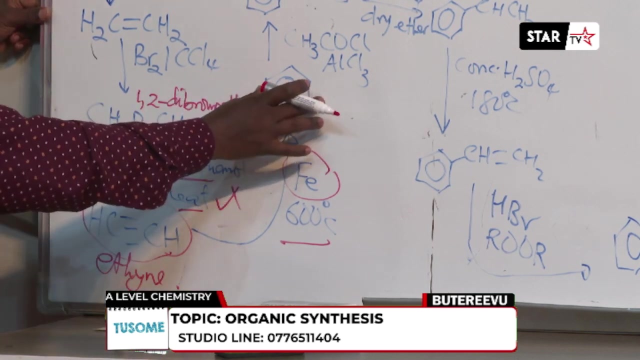 solution. that word solution should be seen in the words. so it is reacted with alcoholic potassium hydroxide solution on heating to form ethane. this is ethane. the ethane is heated in the presence of iron tubes at a temperature of 600 degrees celsius to get benzene, which is then reacted with ethanol chloride. 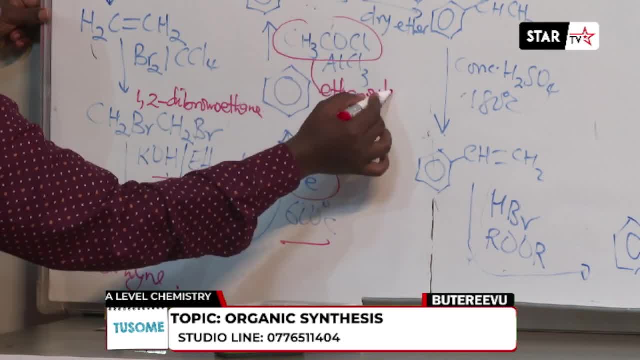 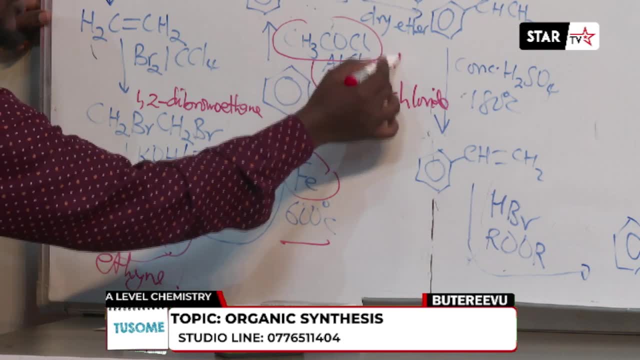 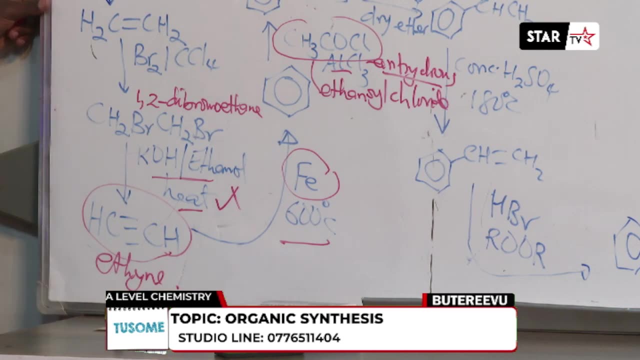 you see, if you don't know these names, then you are not good to go. it's reacted with ethanol chloride in the presence of aluminium chloride, which is anhydrous in the presence of anhydrous lithium, aluminium chloride catalyst to form this compound. what is its name? because you're writing. 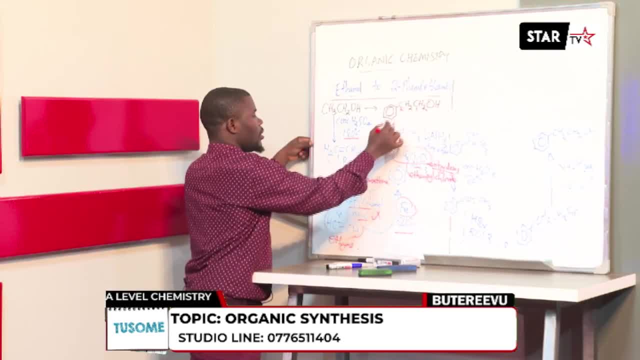 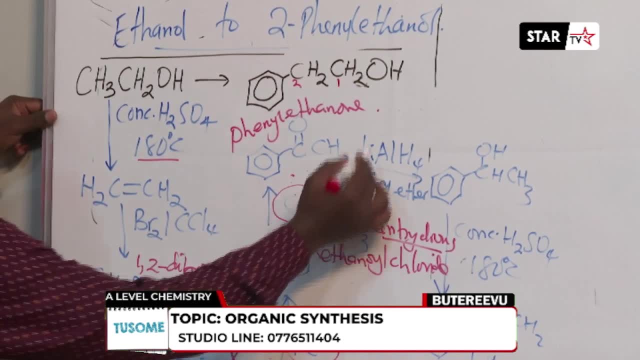 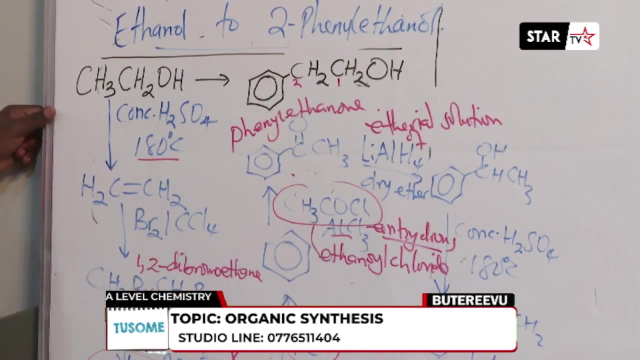 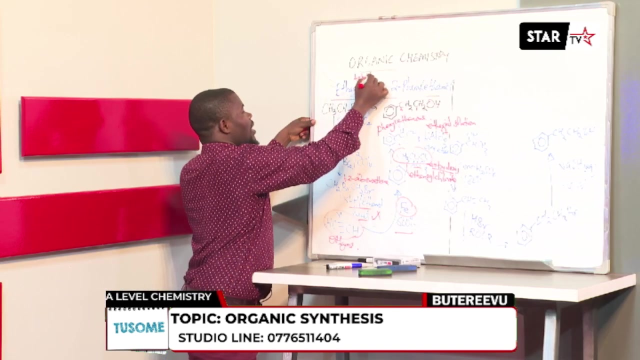 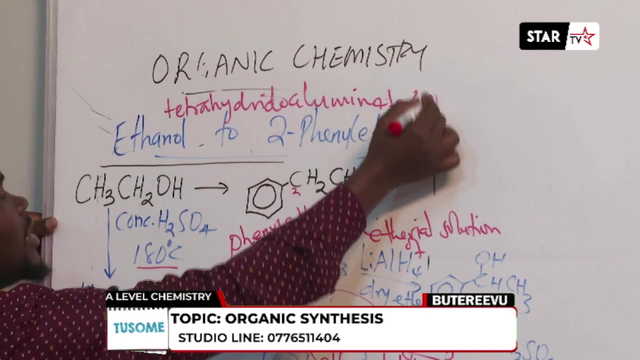 words. this is phenyl ethanol, a ketone. the phenyl ethanol is then reacted with an ethereal solution- or people call this lithium aluminium tetrahydride- i don't prefer that name- an ethereal solution of hydridoaluminate three. that's the name of that solution, tetrahydridoaluminate three. don't put dots here. 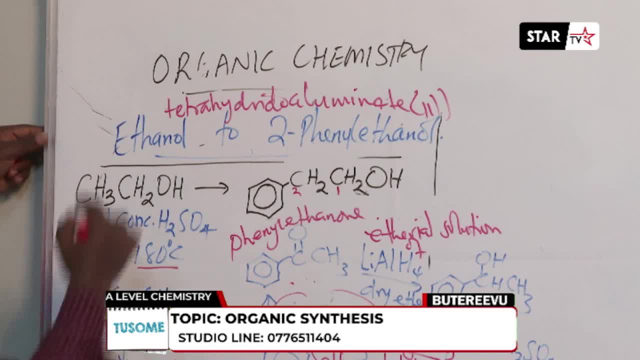 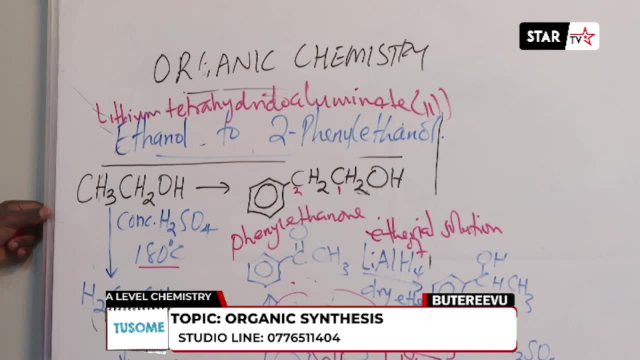 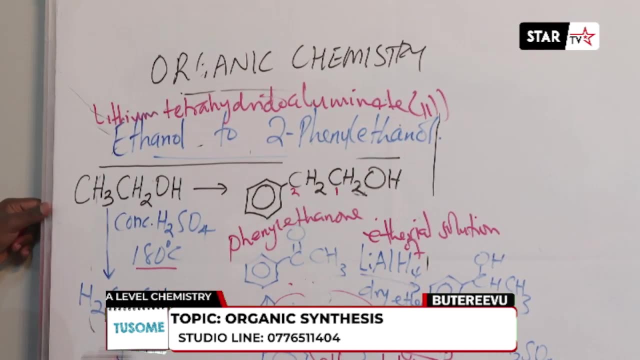 an ethereal solution of lithium. it's called the lithium tetrahydridoaluminate three. all you can say is heated with lithium tetrahydridoaluminate three solution in presence of ether. so the two in the form of a calcium acid and a sodium acid. this is the element of lithium. 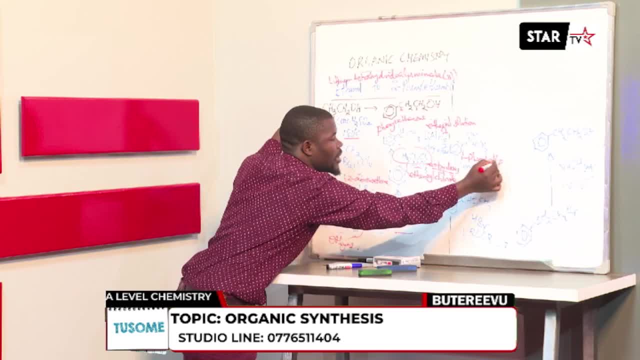 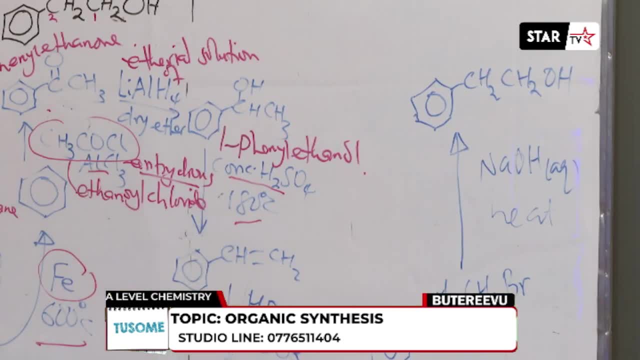 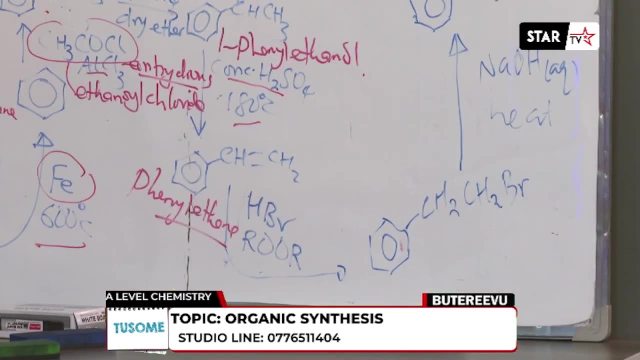 섽, and it is, then it is. then it will react with a dry ether to form two phenyl. this is one phenyl ethanol, one phenyl ethanol, which is then reacted with concentrated sulfuric acid at 180 degrees celsius to form phenyl ethene. 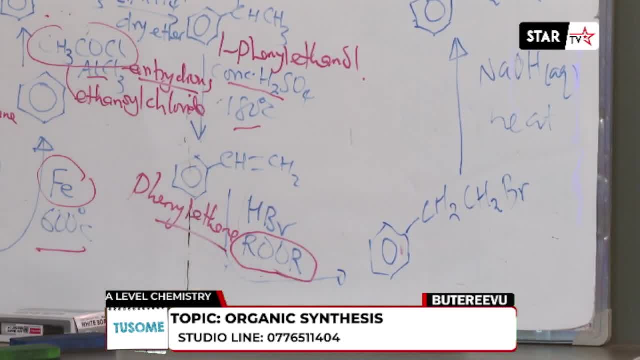 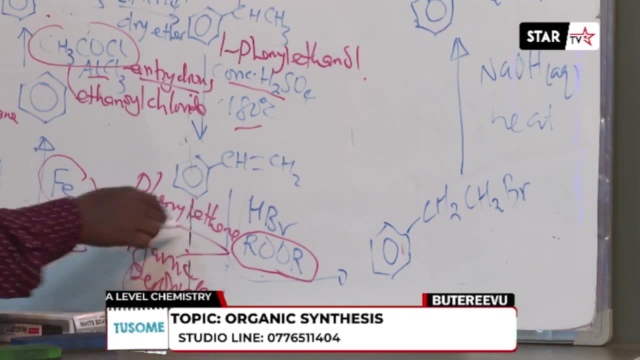 phenylethene is then reacted with the dry hydrogen bromide in the presence of phenylethene is then reacted with the dry hydrogen bromide in the presence of an organic peroxide. this should be not any peroxide, it should be an organic peroxide. if you know the example, you can give an example of dibenzoyl peroxide or. 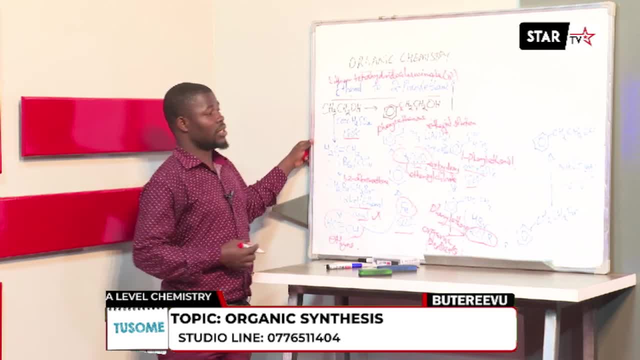 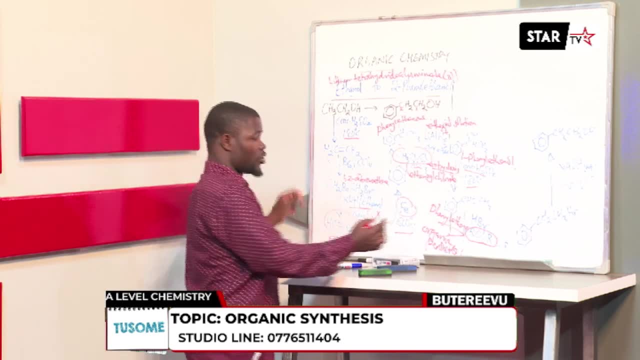 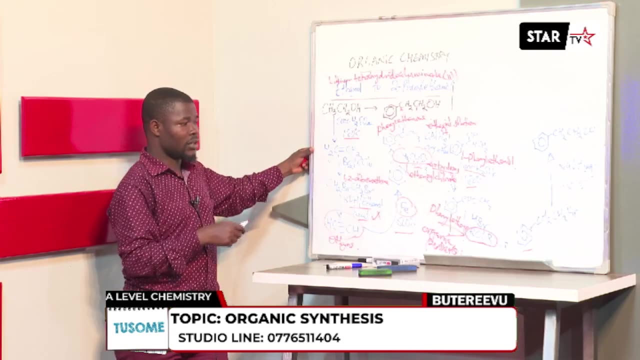 benzene. yeah, you can use dibenzoyl peroxide or any other peroxide that's organic, so this one yields. you should know the name of this compound here. that compound is called two phenyl, one bromo ethane. you can use that name or you can. 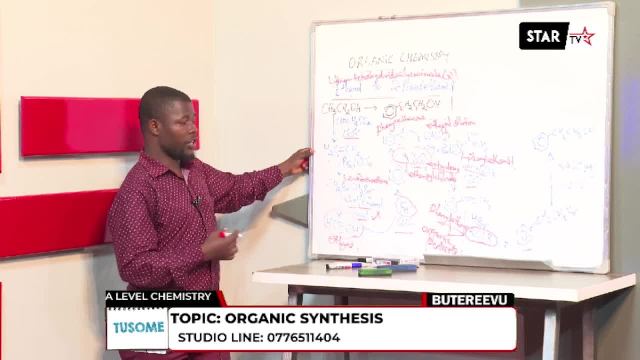 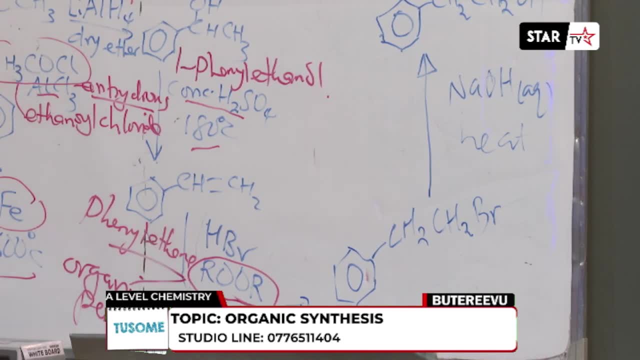 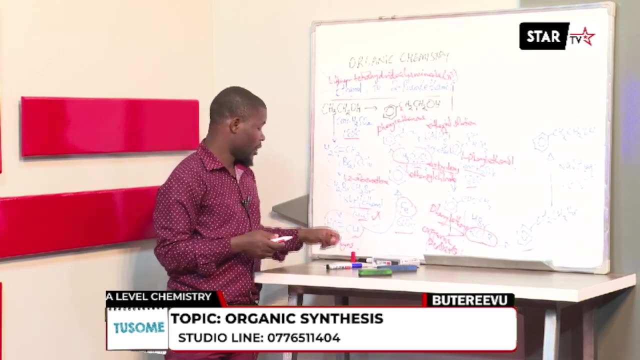 call it one bromo phenyl ethane. then you heat it with sodium hydroxide- this solution to form two phenyl ethanol. that's the approach we use when we are writing mechanisms in words. okay, you can see more of this in the following slides. 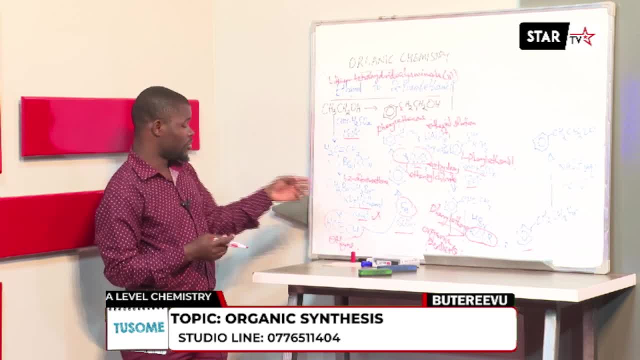 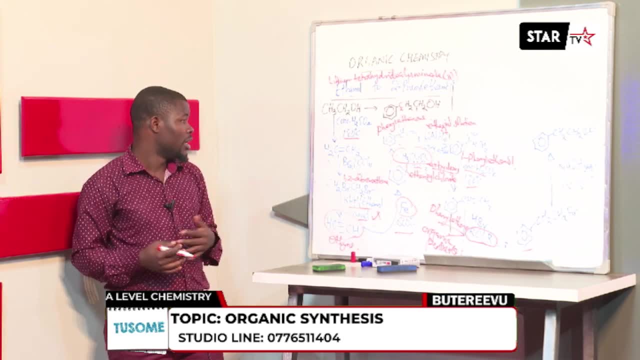 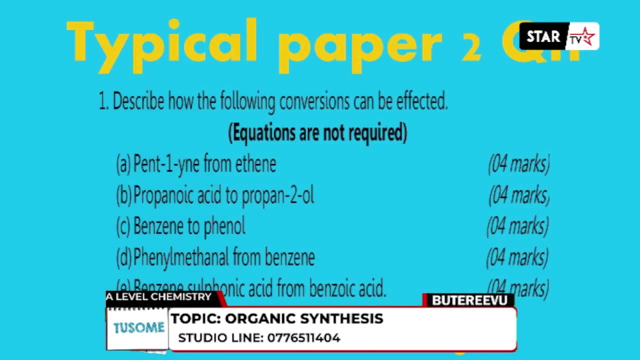 in one of my books demystifying organic chemistry. we also have other books demystifying physical chemistry and demystifying inorganic chemistry. if this is well understood, let's proceed to the next slide and see our next approach. that is a typical paper two question that was set last year and most of the 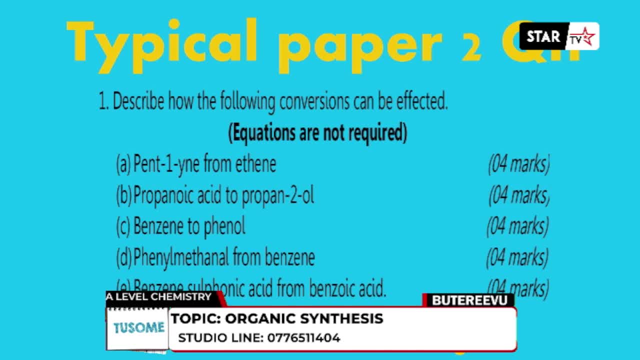 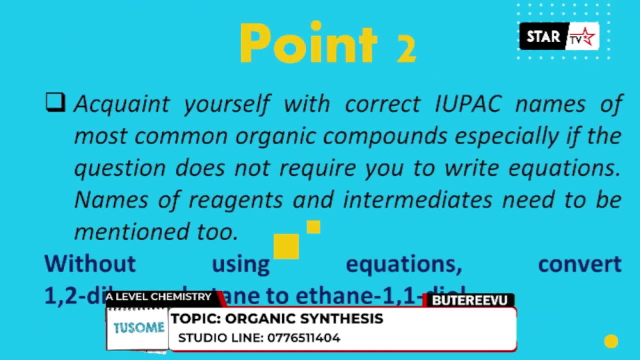 students failed it. I'm showing you how a question can be set and it carries 20 marks. just slide. yes, dear viewers, that's our second point. when you're doing organically synthesis, it also a point that you should do not. chemistry is fun. chemistry is not a mystery. I 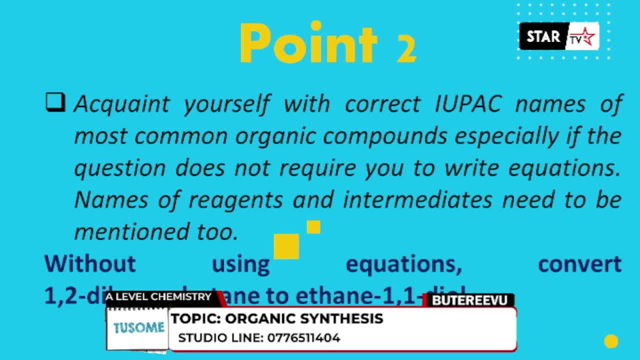 don't know why students take chemistry to be a mystery. most students fear it. you pass in town. you tell us capacity that you're teaching chemistry- they run away from me. you pass in town. you tell us the person that you're teaching chemistry- they run away from you. 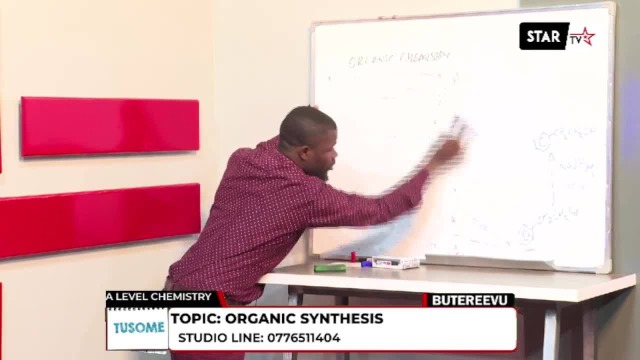 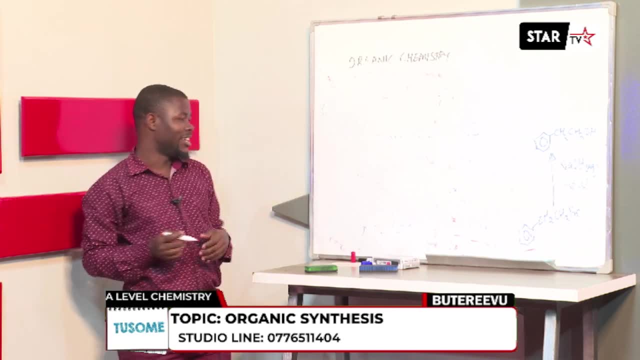 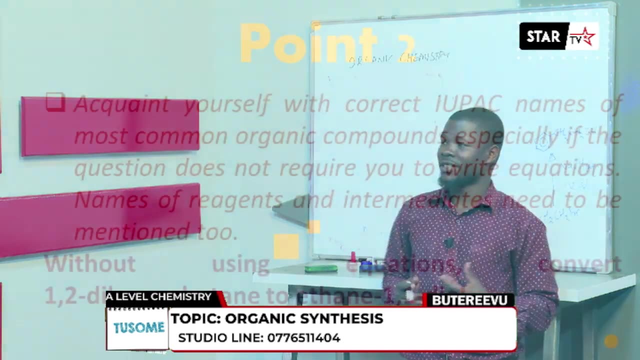 they ran away from me. you, They think you are a terrorist. Chemistry is not terrorism. Chemistry is a very enjoyable subject. Now, when you look at your screen, you're seeing the second point, which says you should acquaint yourself with the correct IUPAC names of most organic compounds, especially if the question 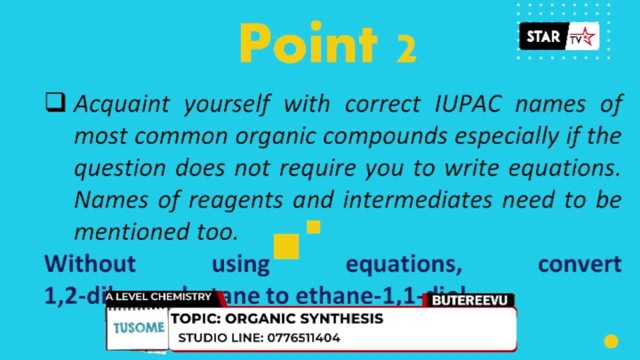 does not require you to write equations. Names of reagents and intermediates need to be mentioned too. You can see an example there Without using equations: convert 1,2-dibromobutane to ethane- 1,1-diol. Convert 1,2-dibromobutane- 1,2-dibromobutane. is this compound here? 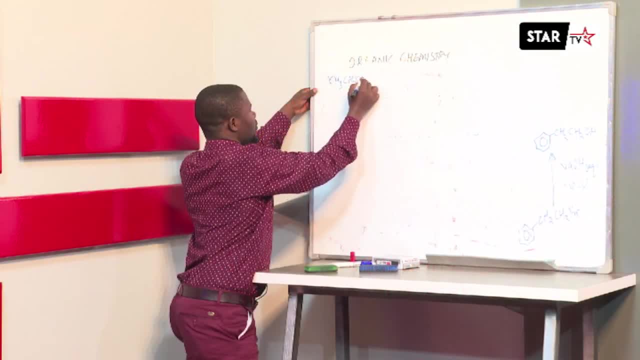 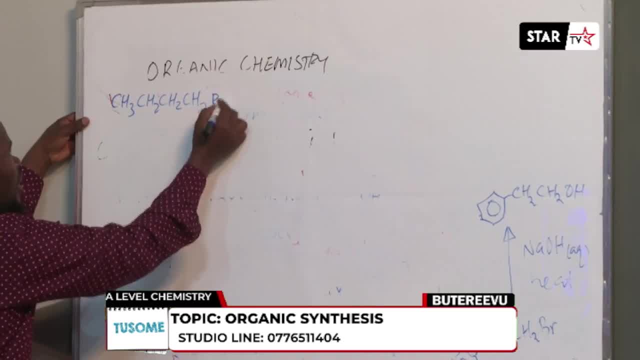 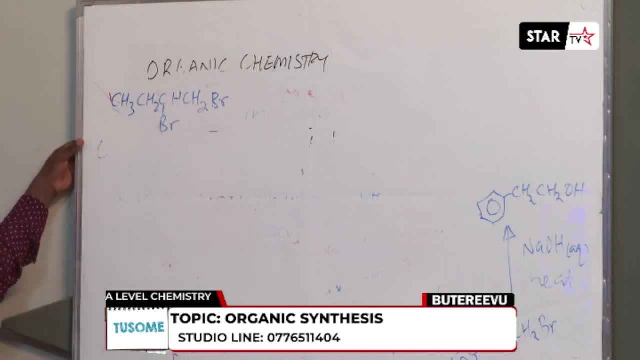 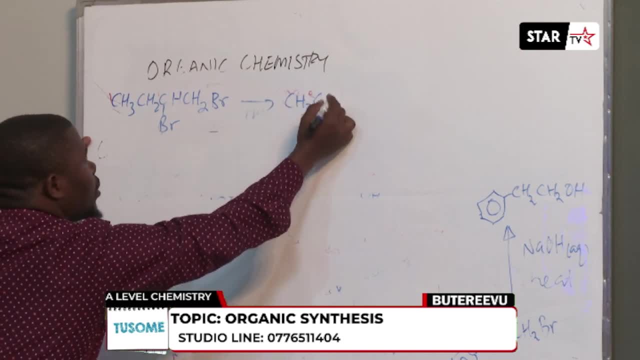 So that is our 1,2-dibromobutane. We want to convert the 1,2-dibromobutane to ethane 1,1-diol, That is, ethane 1,1-diol. 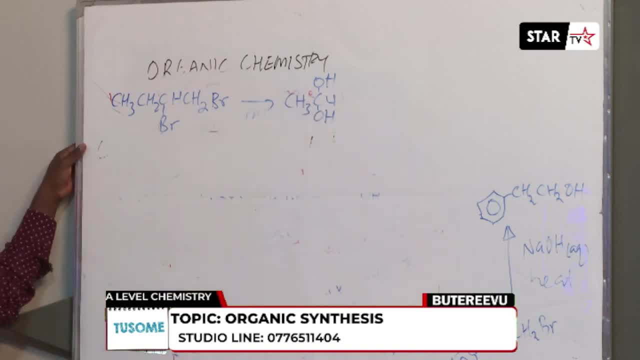 On the same carbon atom, we have two hydroxyl groups, So that is ethane 1,1-diol. When you look at the number of carbon atoms in these compounds, this is 1,2,3,4, and these are. 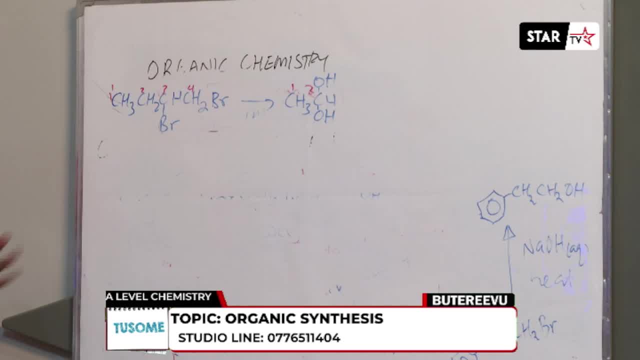 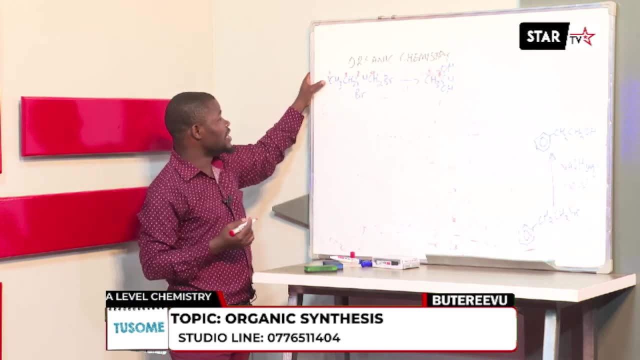 two, meaning some will have to break a given chain that will give us two carbon atoms. How are you going to do that? You must of all make sure this is converted into analkyne, because that's the first step that will. 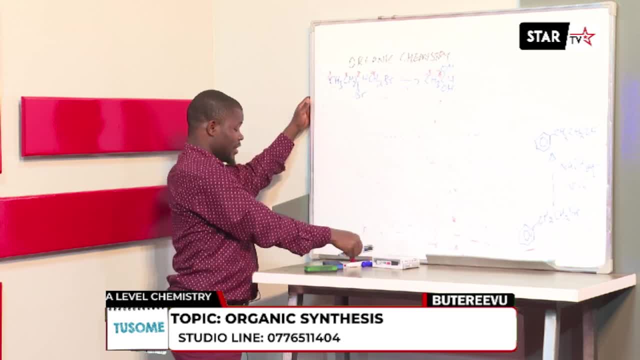 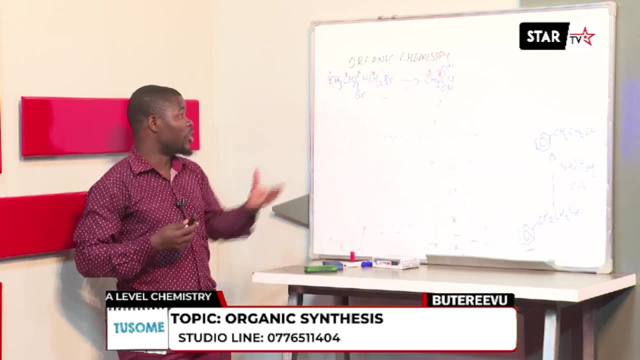 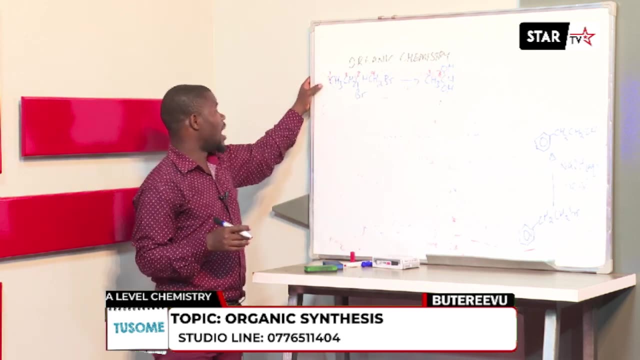 that will ease your work. When you convert it to analkyne, then proceed by converting it to analkyne and then ozonolize. Break the chain by ozonolisis. Okay, And remember please, whenever you're doing ozonolisis, you should use symmetrical alkynes, So not to waste time. 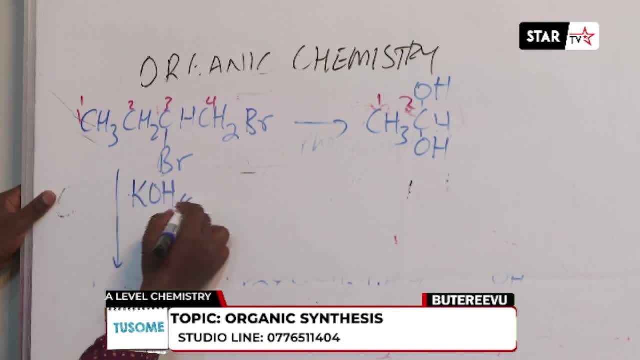 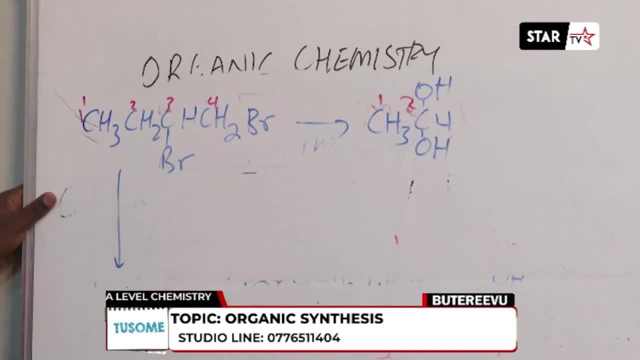 I'll say I'm going to use potassium hydroxide. Potassium hydroxide- I think people always also use this. They call it alcoholic, Alcoholic, potassium hydroxide And then heat. That's the same as what I've done in the previous description, where I said: 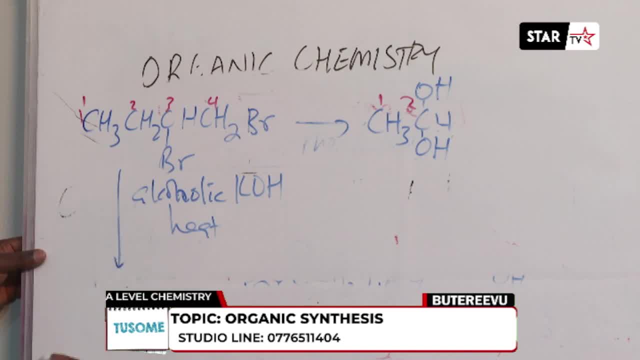 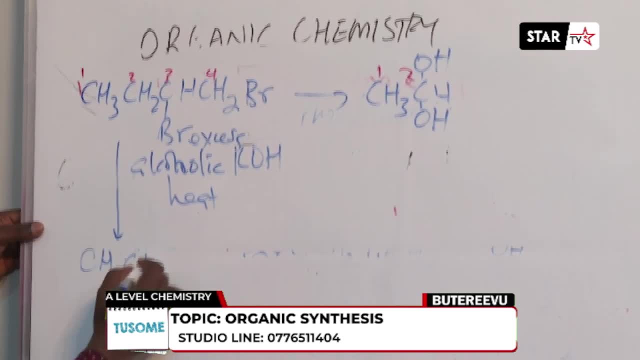 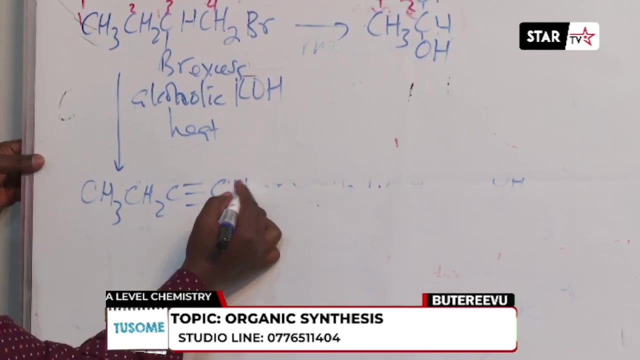 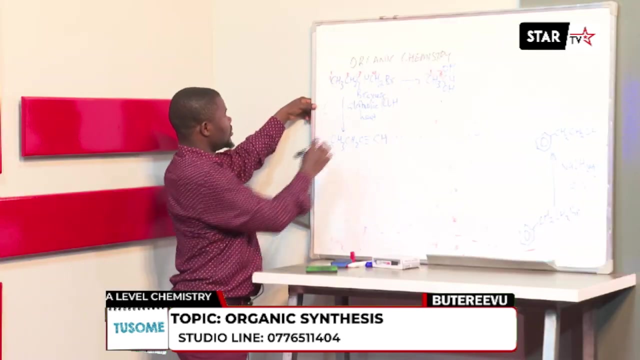 potassium hydroxide stroke ethane. It's the same thing. When you heat this, you're going to use- other people prefer putting the word excess. When you heat this, you're going to get analkyne. That is analkyne, which analkyne is called butyители one-ion. The analkyne is this one here. 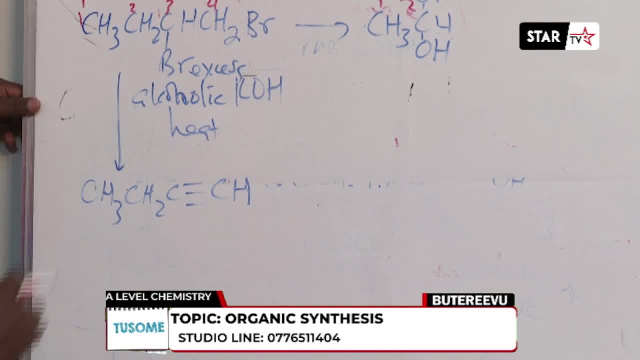 This analkyne here should be converted to analkyne. How do you convert it to an alkene? Use hydrogen in the presence of Lindler catalyst. So hydrogen in the presence of Lindler's catalyst don't hit People don't know Lindler's catalyst. It's the same as 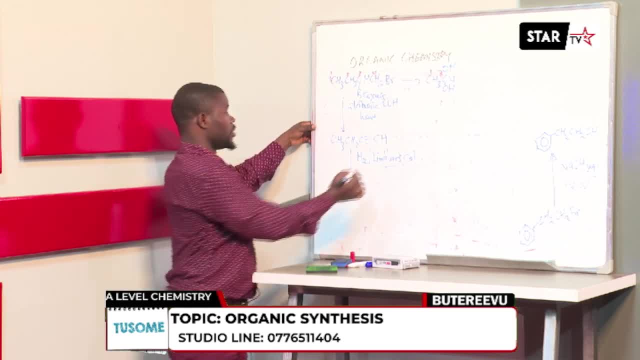 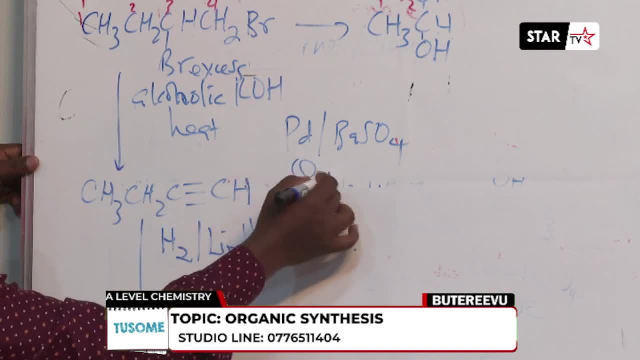 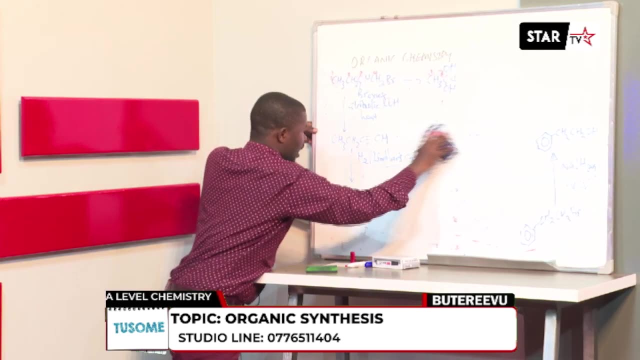 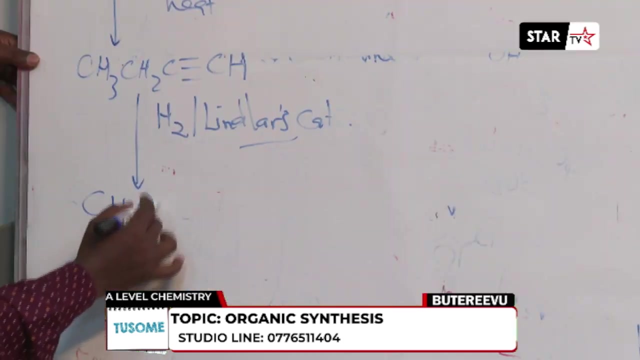 palladium, Palladium supported on barium sulfate. Barium sulfate gives the support to palladium and the whole catalyst is poisoned by quinoline, But those details may not be relevant for now. So when you use hydrogen plants of Lindler's catalyst you'll get an alkene. 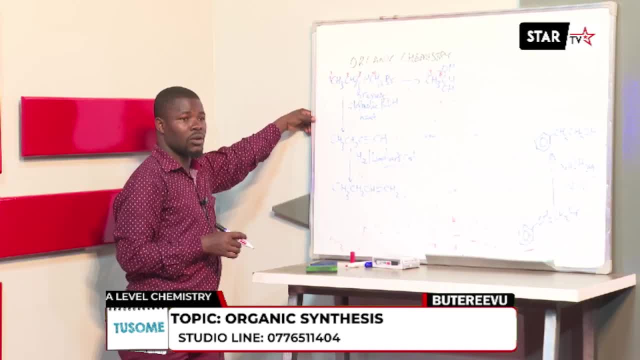 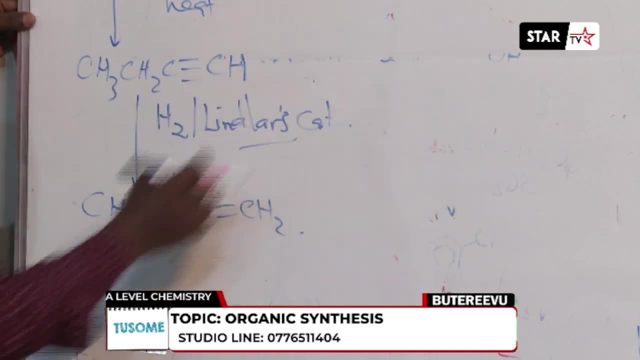 Which alkene we call but-1-ene. That's the alkene you will get Now. this alkene here is to be ozonolized. But if you are to ozonolize this alkene, you'll get two aldehydes. 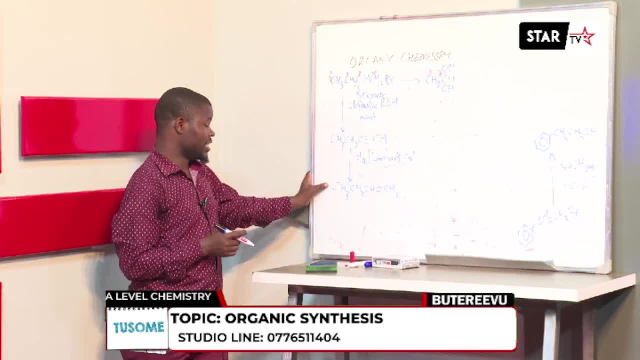 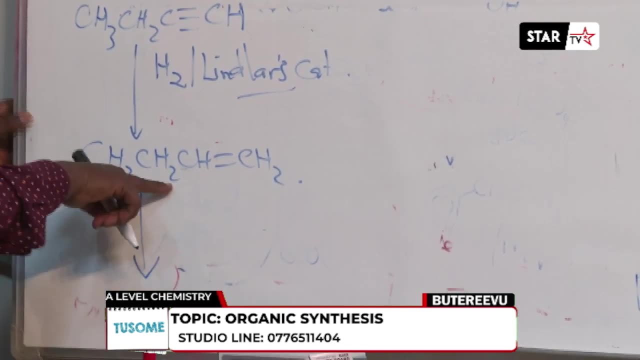 Which two aldehydes are both present in almost the same concentration in the solution. So how are you going to avoid that? Make sure you get a symmetrical alkene out of this. And how do you get a symmetrical alkene out of this? Most people here will do ozonolysis. 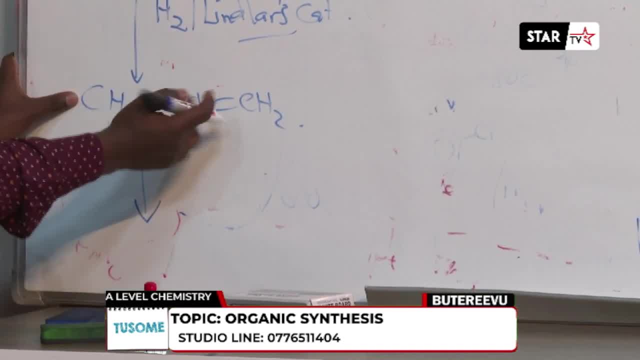 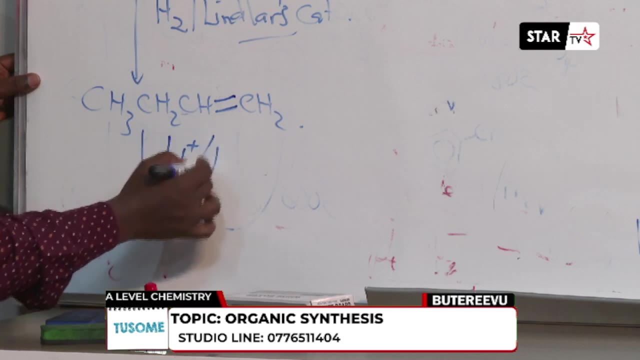 directly And then get. Actually, if you do the ozonolysis, there is cleavage. at this point, You're going to get two aldehydes which will not give you the ozonolize. So you're you the desired product. so, to avoid that, what are you going to do? you're going to use acidified water. 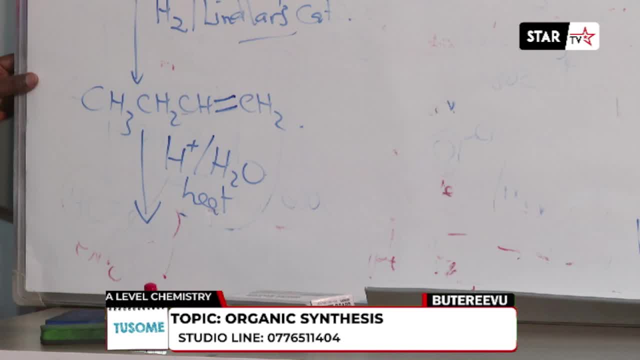 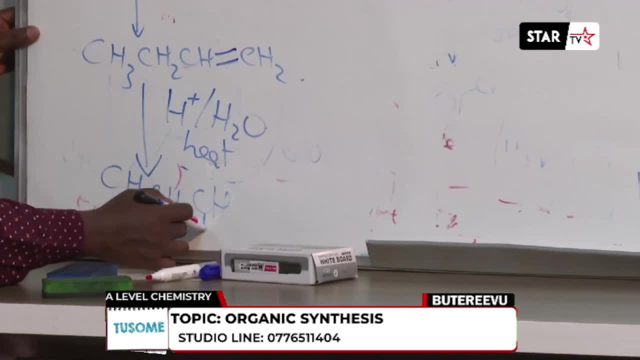 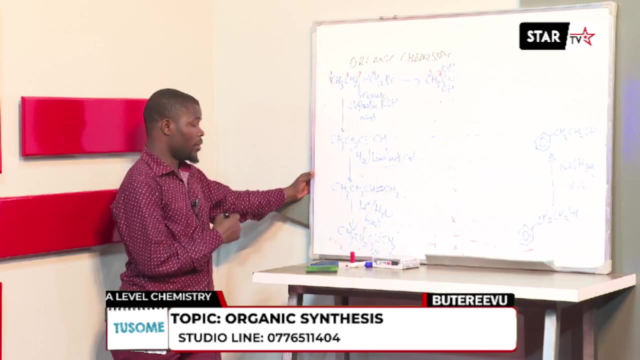 and heat or warm. when you do that, you're going to get an alcohol. the alcohol you get in this case is not a primary alcohol, it is a secondary alcohol that is butan to all. after getting butan to all, we still have a way to go. you're going to. 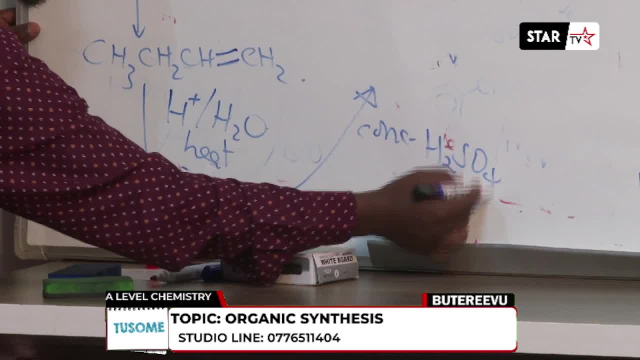 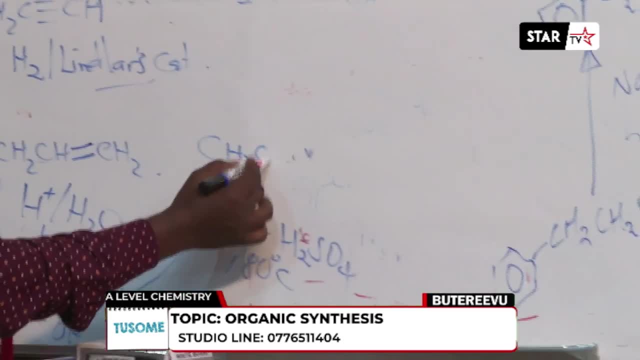 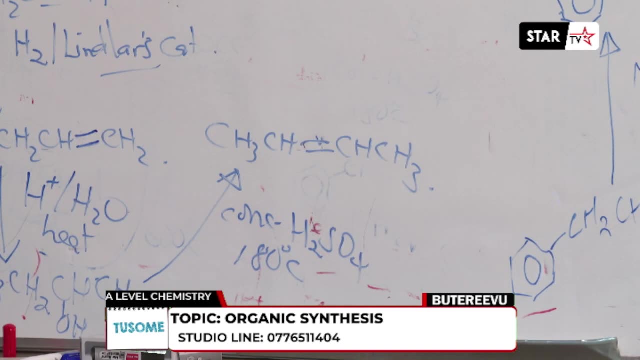 dehydrate using quark sulfuric acid at 180 degrees celcius. so when you dehydrate, you're going to get ch3 ch, ch, ch3. yes, there is a student i'm seeing there, i'm seeing you getting perplexed. you're going to get ch3 ch, ch, ch3. and you're going to get ch3 ch, ch, ch3. 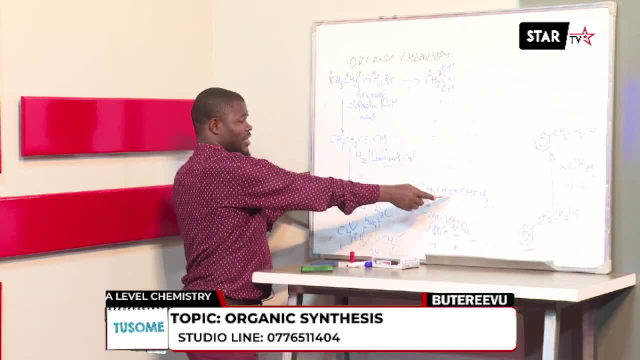 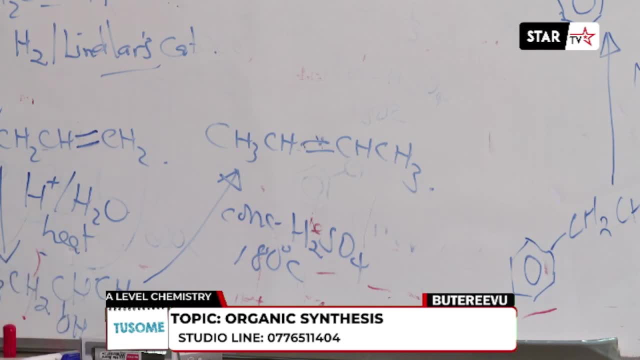 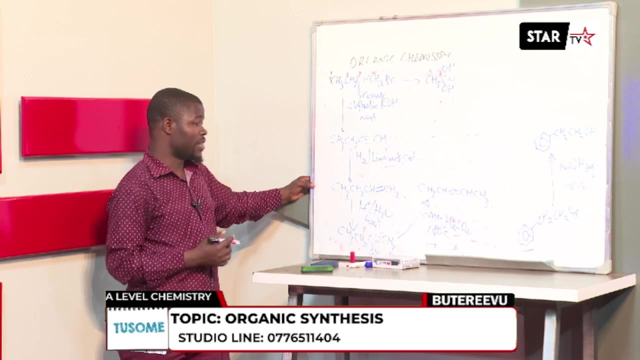 you're wondering how i dehydrate this and then i get the double bond between these carbon atoms and not these ones. when you put the double bond here, that means the carbocation you used to get that alkene was the most unstable carbocation. i think you remember that mechanism that involves 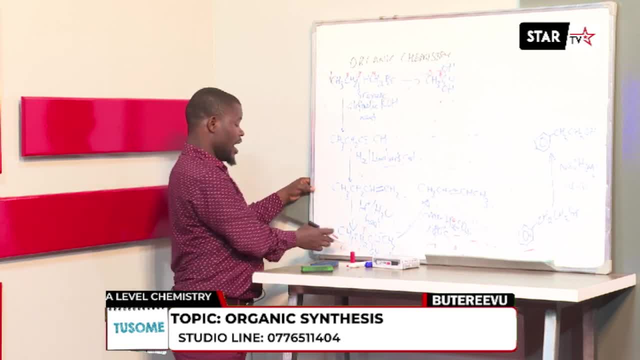 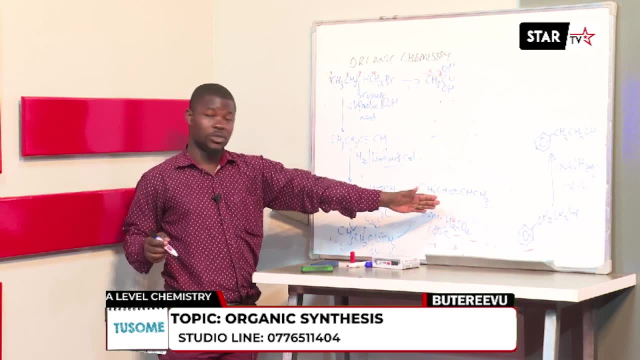 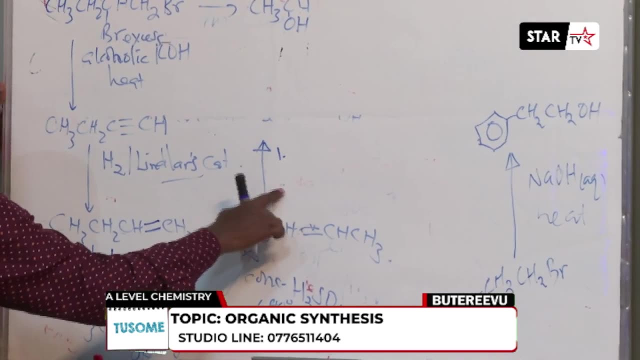 a hydride shift. so when you dehydrate any alcohol that has four carbon atoms you get a symmetrical key. should always note that you get a symmetrical key. should always note that. then here we can do our zoonosis also. analysis is done in two steps. you should show step one and step two. 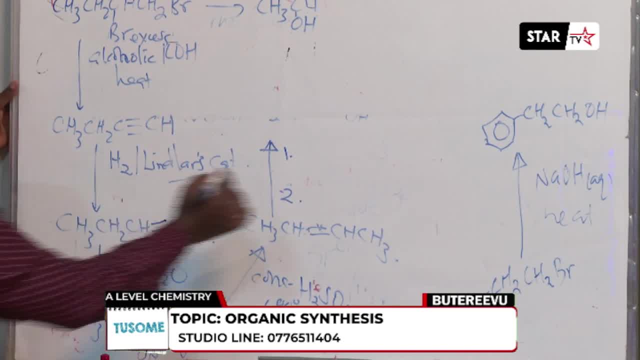 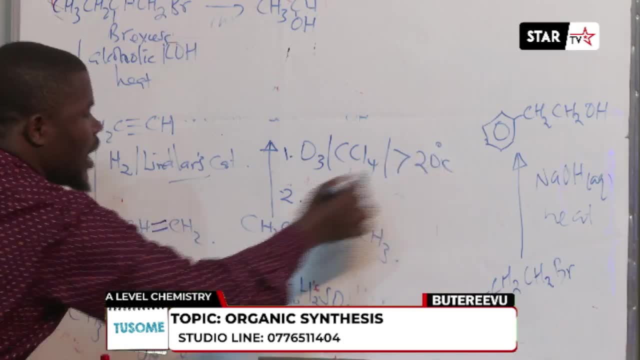 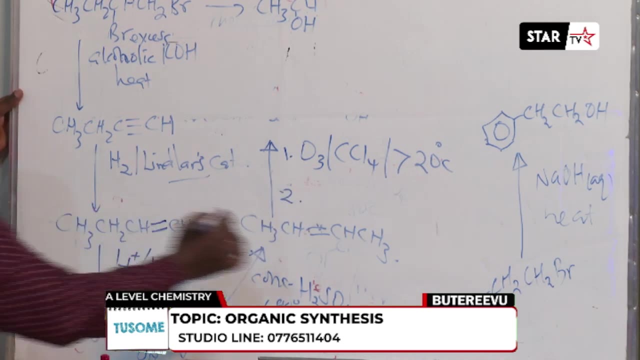 what is step one is on the ozone. in ozone analysis, step one: use ozone presence of carbon tetrachloride at a temperature of greater than 20 degrees celcius. then the second case: after zoonosis, you'd hydrolyze in the presence of zinc and ethanoic acid. I've seen people using zinc and ethanoic acid alone. 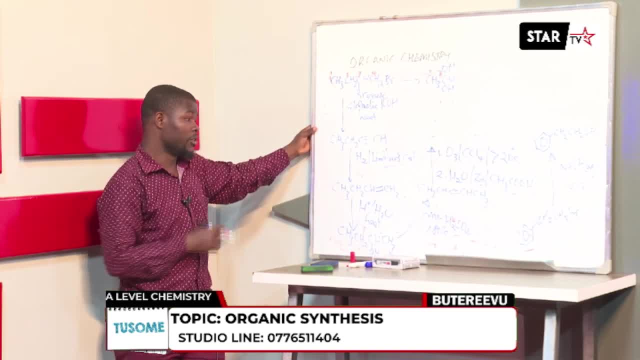 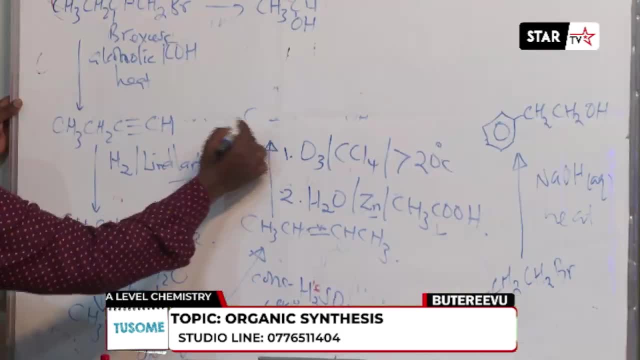 but haven't seen that in any literature. So water is very important because this is hydrolysis. Now, when you do that, you're going to get an aldehyde. You get two molecules of this aldehyde because there's cleavage at that point. 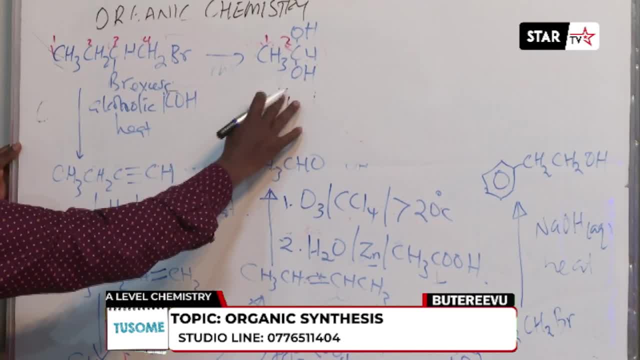 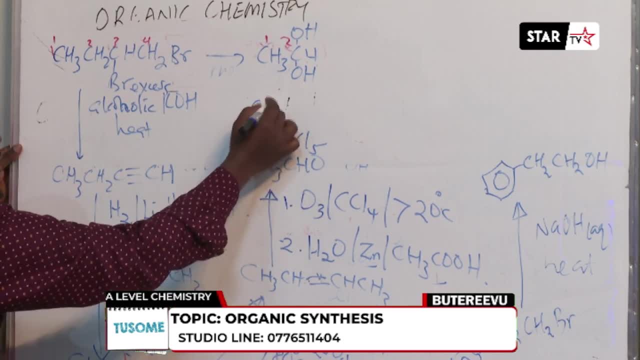 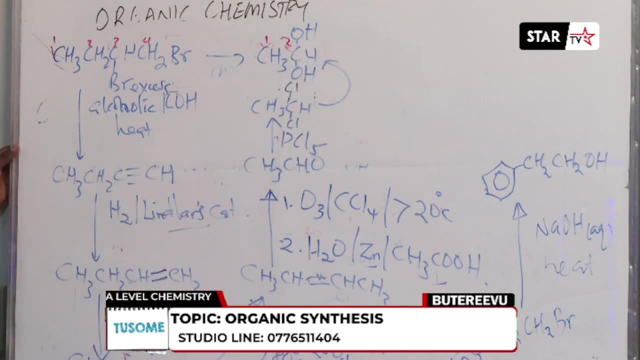 and finally, you can convert the aldehyde to the diol by first of all using phosphorous pentachloride. That gives you this product here, And then, at that point, you can do our last step that we did in the previous reaction, by using 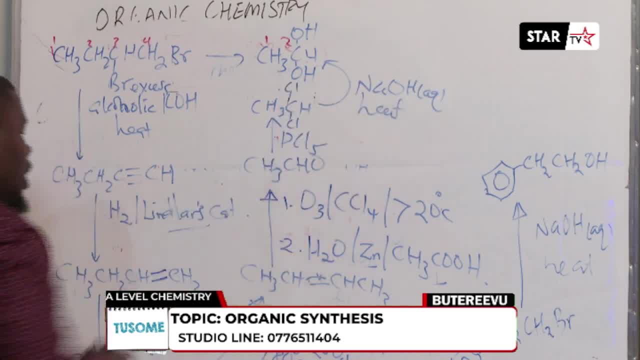 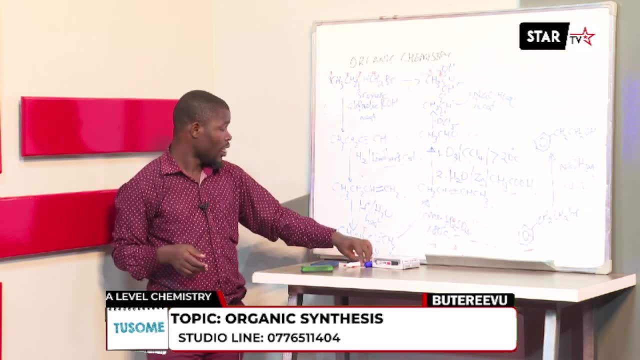 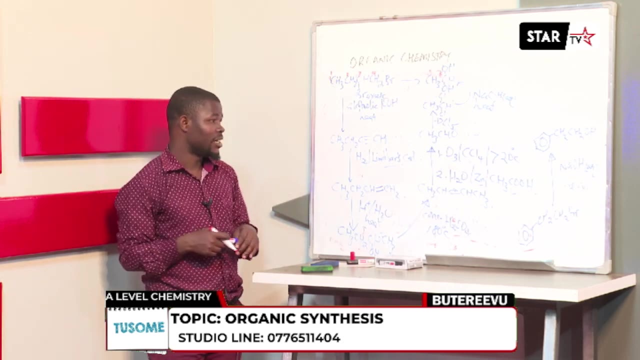 aqueous sodium hydroxide. Don't forget to hit dear students. I hope you're following and you're enjoying this lecture. Thank you very much. Now, our question said: we are not using equations, We are using words, So you can get your books. 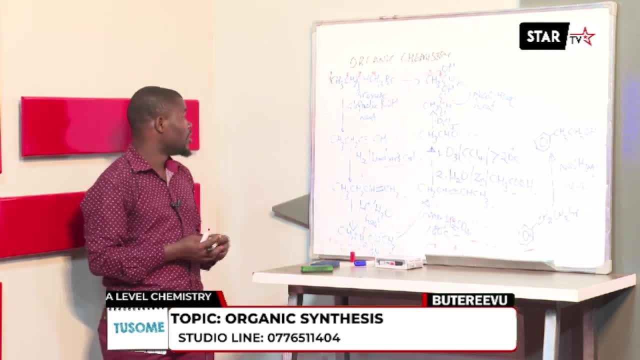 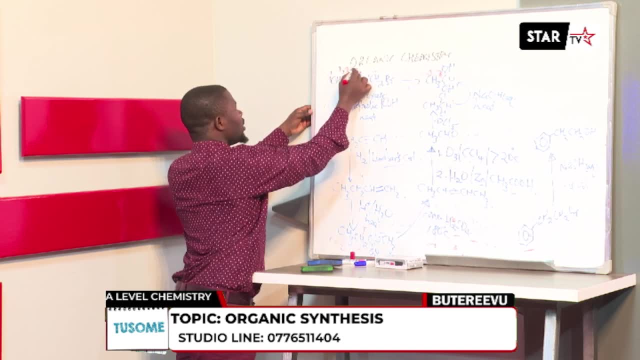 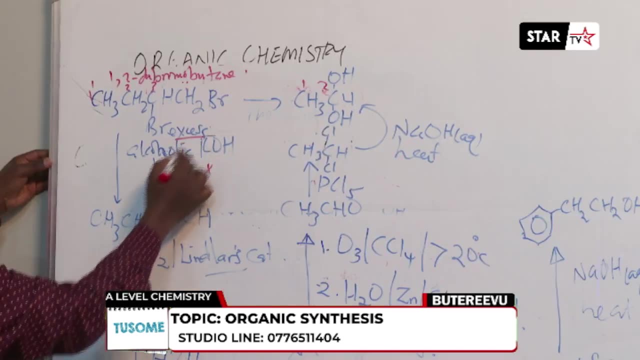 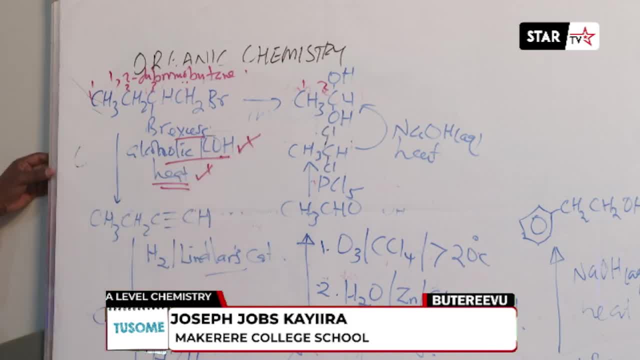 All right. So at this point let me give you a little bit of a breakdown. So you are using 1,2-dibromobutane here, which is an extract of calcium hydroxide. If you call 1,2-dibromobutane, 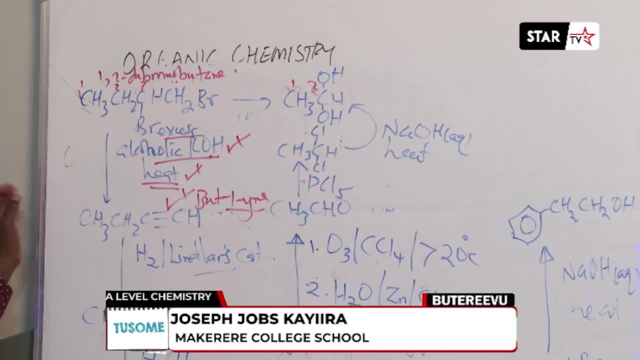 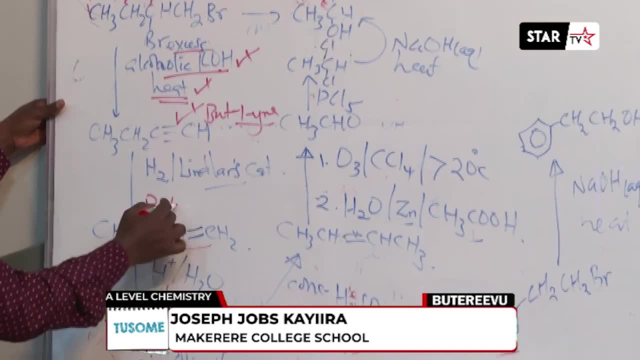 you have 1,2-dibromobutane in the form of a curablestrom, So this is a solution called 1,2-dibromobutane here. It's a solution of potassium hydroxide which will form a 1- Hessian. 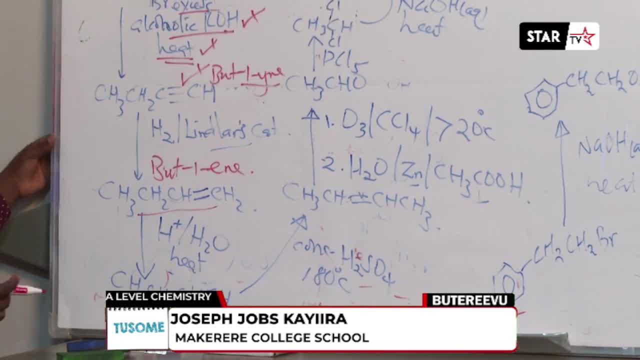 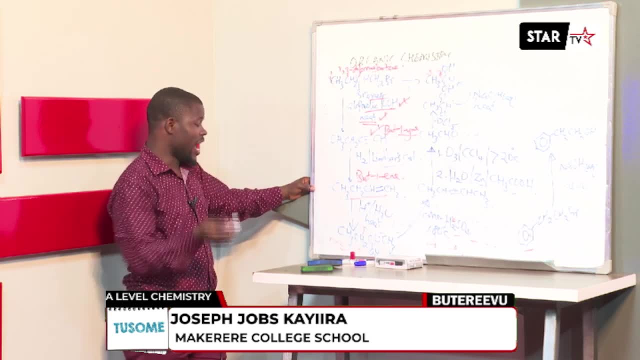 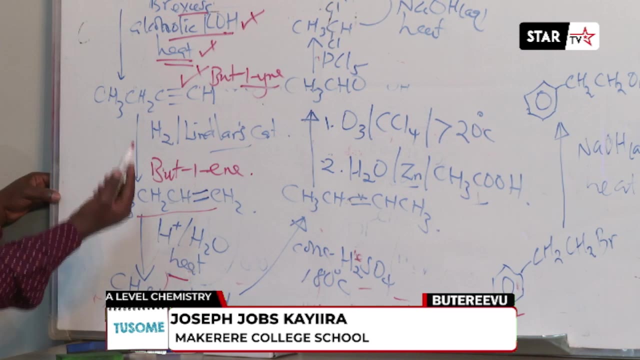 index. So let's then compare it with hydrogen. We have to find that 2,2-dibromobutane in this solution. It leads to B1. Yes, B1. Yeah, So it is our solution. with water on heating to form butan-2-ol. Or you can simply say: the but-1-in is. 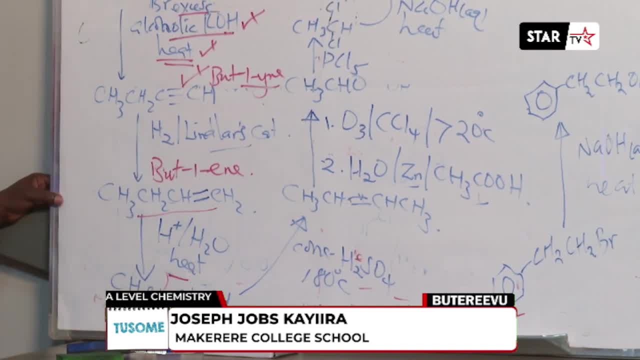 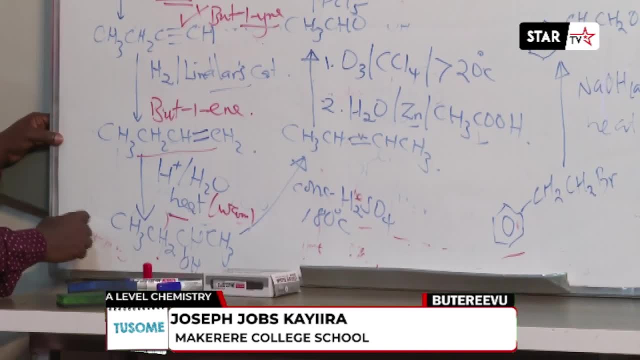 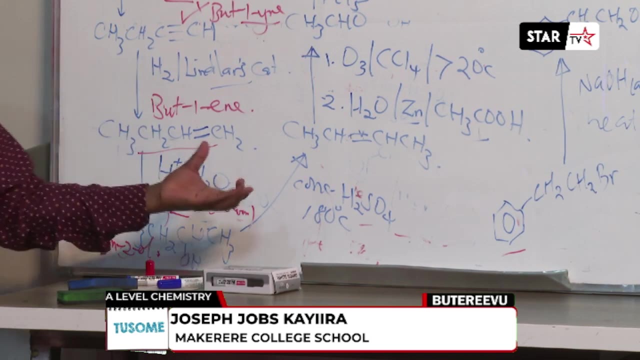 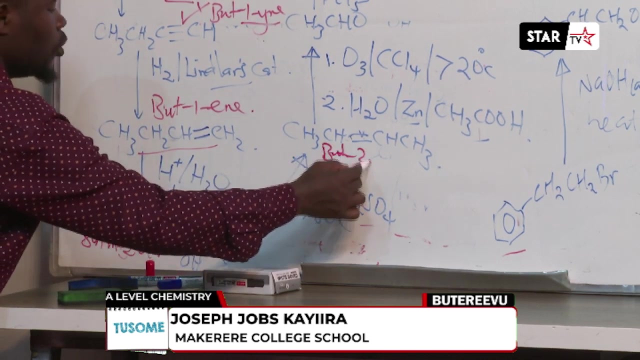 reacted with acidified water on heating or warming. n of the two is acceptable to form butan-2-ol, which is then heated or dehydrated using concentrated sulphuric acid at 180 degrees Celsius to form butan-2-in. You're writing words. Now here is where most 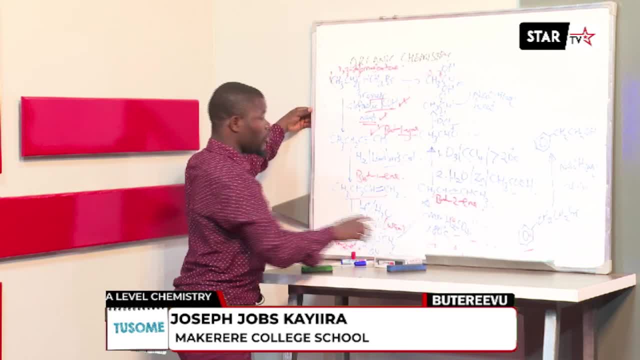 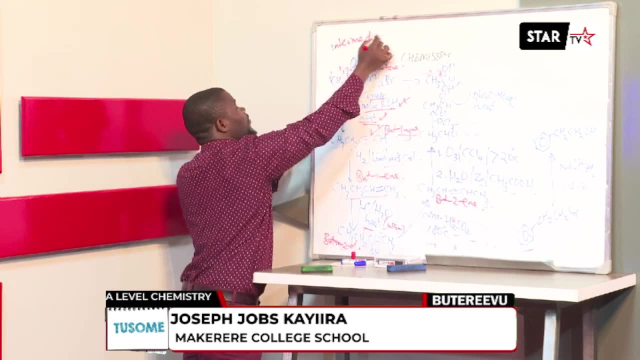 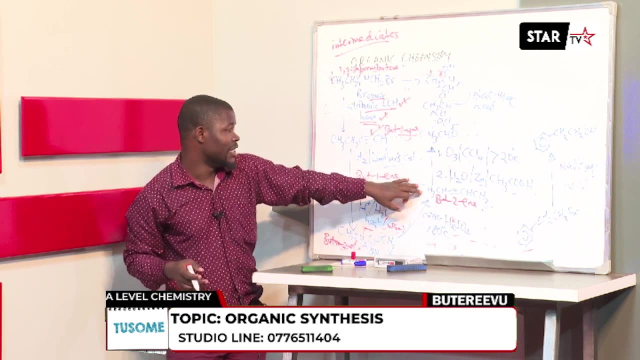 students messed up last year at this point. There was a question that involved ozonolisis as one of the steps, And I've told you, always name all intermediates involved. Always name all intermediates involved. So what do you say? Butan-2-in is first of all reacted with ozone. It's 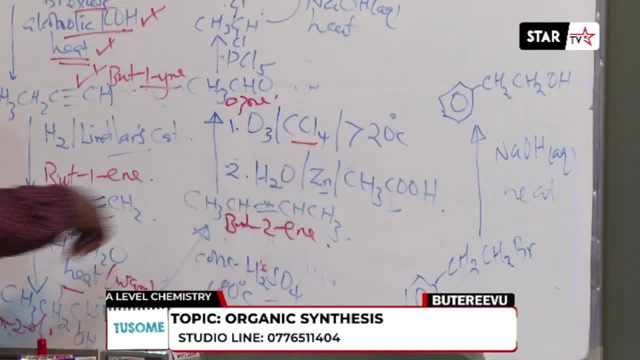 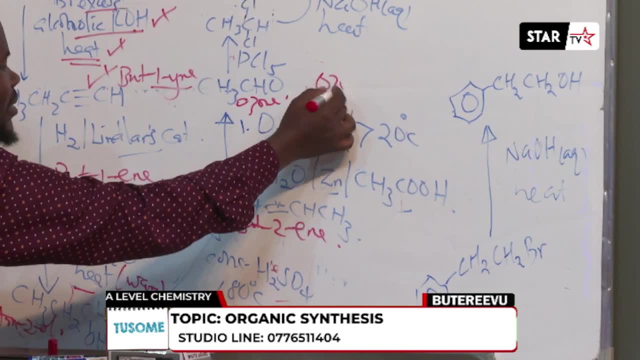 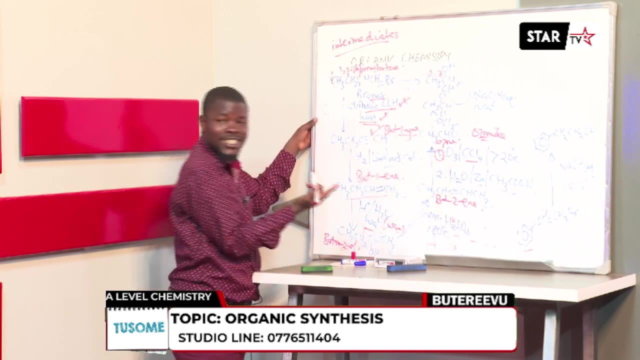 compounds called ozone in presence of carbon tetrachloride at a temperature less than 20 degrees Celsius to form an ozonide. You don't know the name of that ozonide. The intermediate after step one is an ozonide, Which ozonide is then hydrolyzed using zinc and ethanoic. 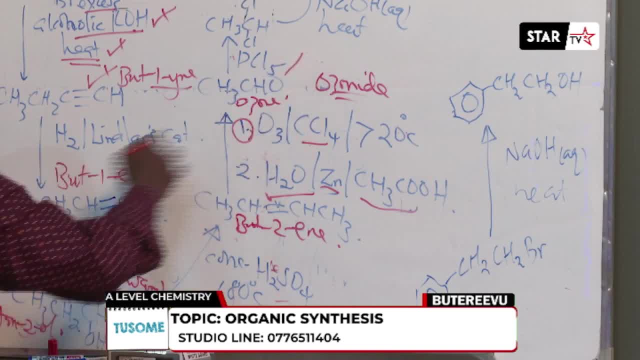 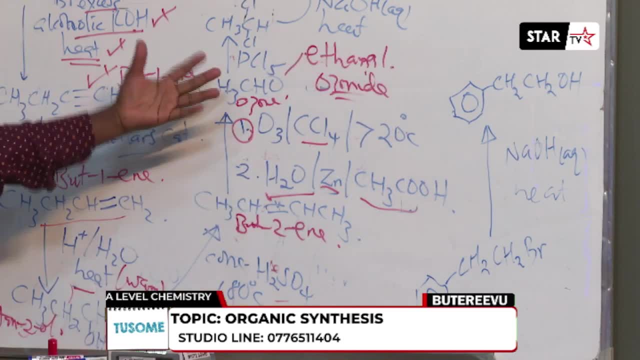 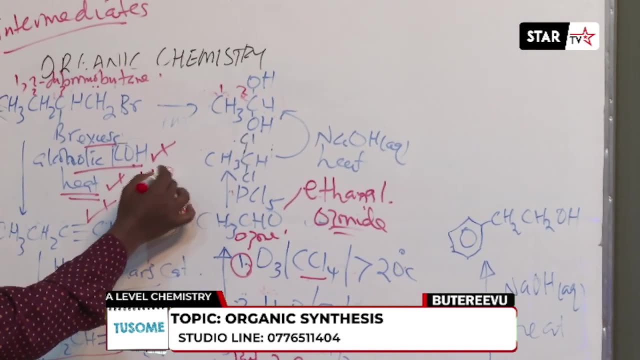 acid to form this compound here is called ethanol. It's an aldehyde. Ethanol is then reacted with the phosphorous pentachloride- don't heat at this point- to form 1,1-dichloroethane, which is then heated with sodium. 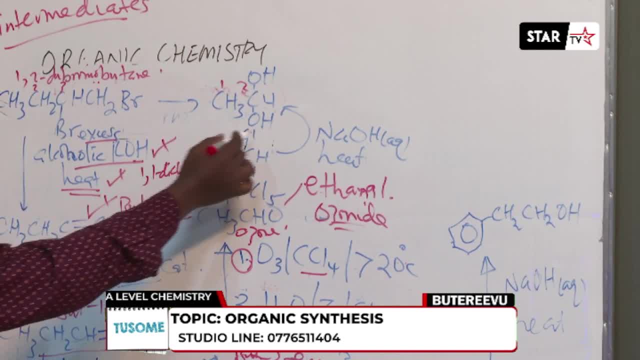 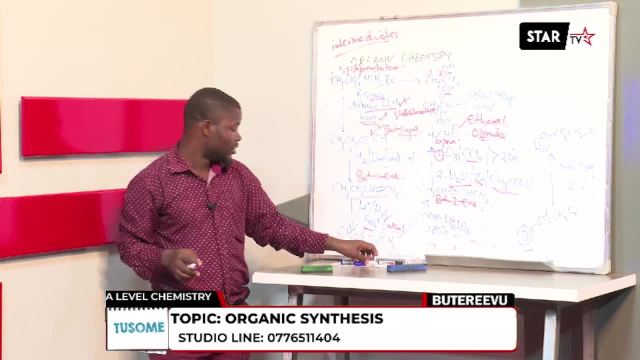 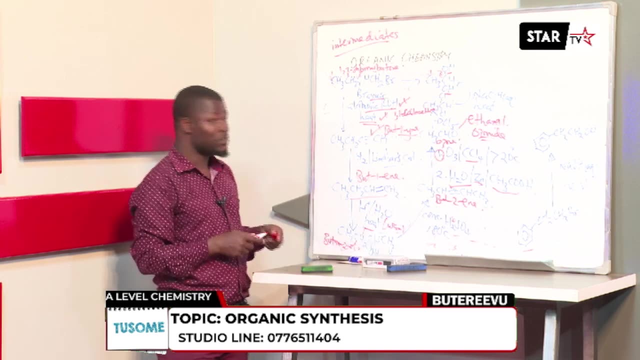 hydroxide solution to form ethan-1,1-diol. Hope that is perfect. Chemistry is simply fun. So whenever I'm doing these things, I'm just enjoying, And I know all of you seated at your home, perhaps taking 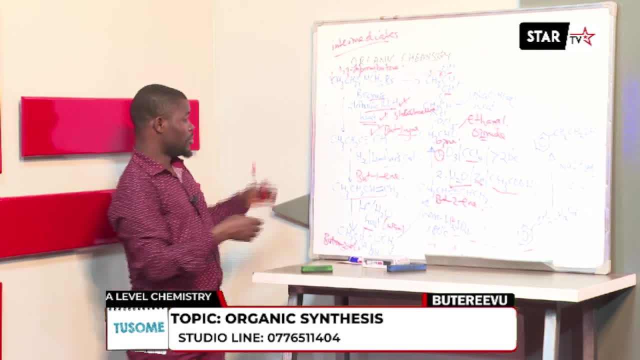 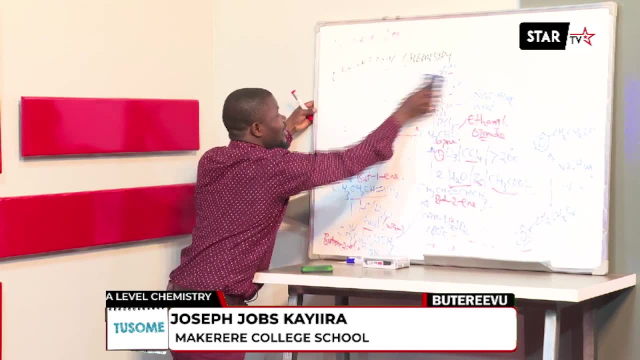 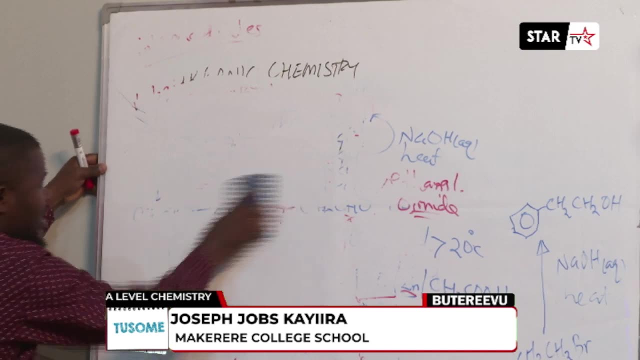 a cup of tea and water. you're enjoying this, People from Masakasa Secondary School. I know you're enjoying- I'm your OB there. So let's proceed to the next slide and see what happens after this. When you look at your screen, you see what the next slide is suggesting. 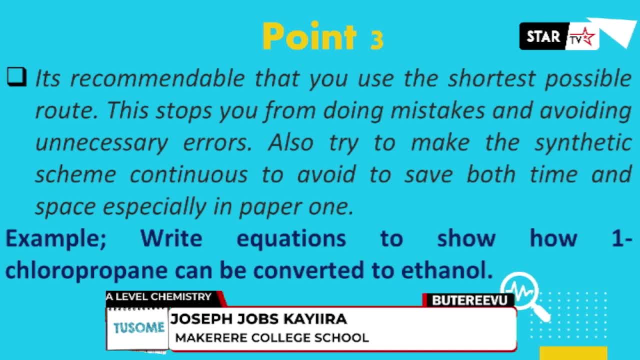 The next slide is saying we have Point Three. Point Three says it's recommendable that use the shortest possible route. This stops you from doing mistakes and avoiding unnecessary errors. Also, try to make the synthetic steam continuous to save both time and space, especially in paper 1, where space is usually a bit. 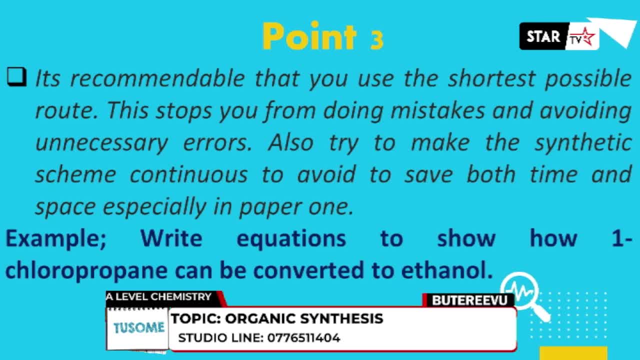 inappropriate. The right equation is to show how: 1- chloropropane can be converted to ethanoic acid. So this is an example of how to get a. This time they have taken us back to our old method, where we should write equations to show how 1-chloropropane can be converted to ethanol. 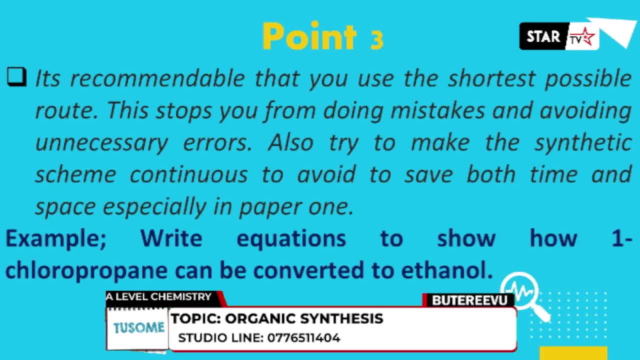 How do we convert 1-chloropropane to ethanol? 1-chloropropane to ethanol? This is 1-chloropropane. We are converting it to ethanol. There are very many routes that can do that. These are three carbon atoms. 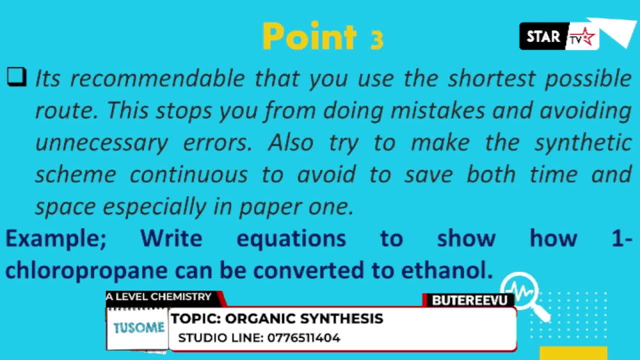 We are reducing them to two, But you should always think of the shortest route to save your time and space. What shall I do to do this? What shall I do to do this conversion? To do this conversion? this is what I'm going to do. 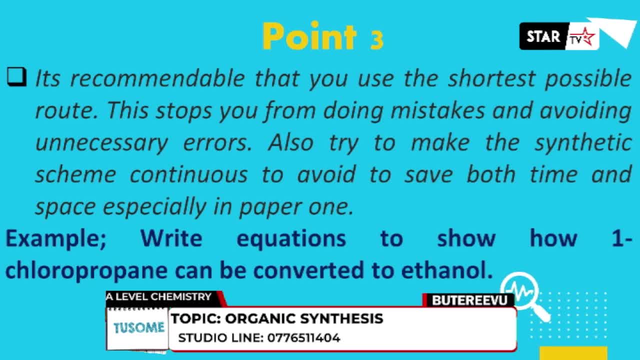 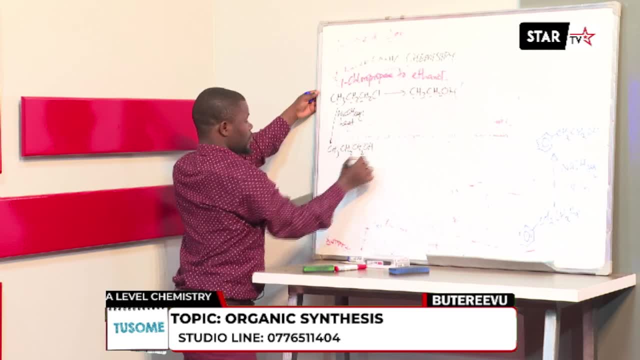 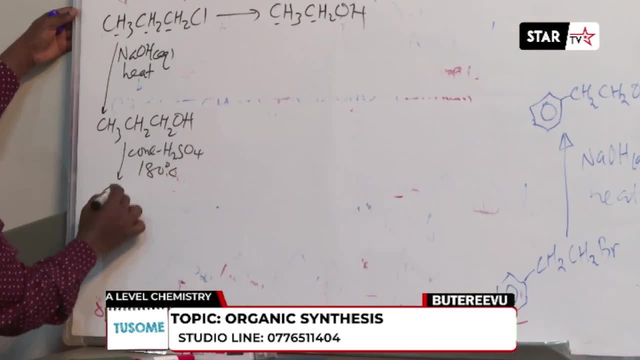 I'm going to first of all use sodium hydroxide and heat. I'm now going to be a bit faster- To give me propano, which is then dehydrated To give me propene. That's my propene. 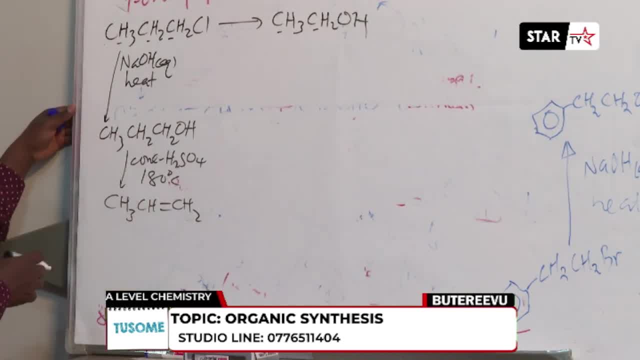 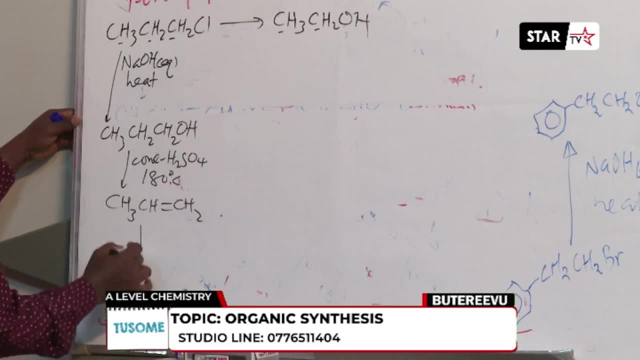 I don't prefer zoonosis at this step, Because this is An unsymmetrical alkene. To simplify my work, I'll go through a symmetrical alkene. How do I get a symmetrical alkene from this? I first of all convert it to an alkine. 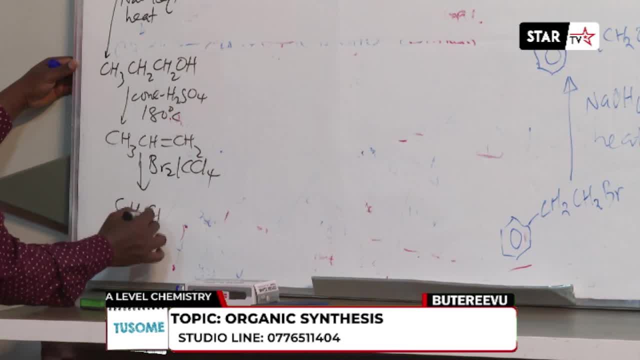 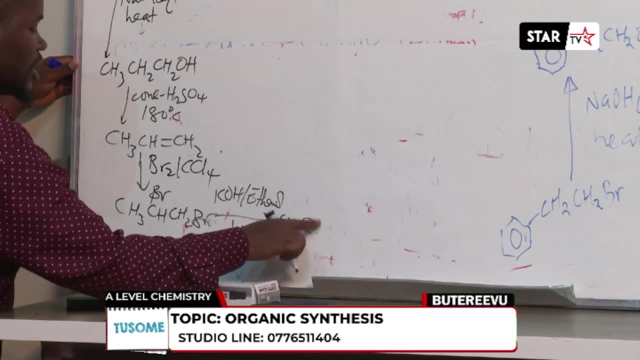 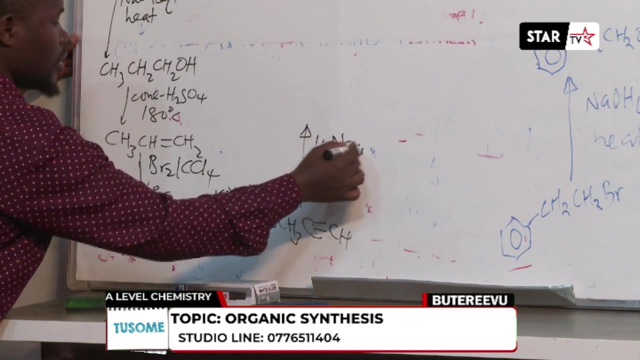 Bromine, carbon tetrachloride, CH3, CH. bromine, CH2, bromine. Potassium hydroxide, ethanol, heat, CH3, CH. C, triple bond, CH, Step one. sodium solid liquid ammonia- Step two. that one gives you. 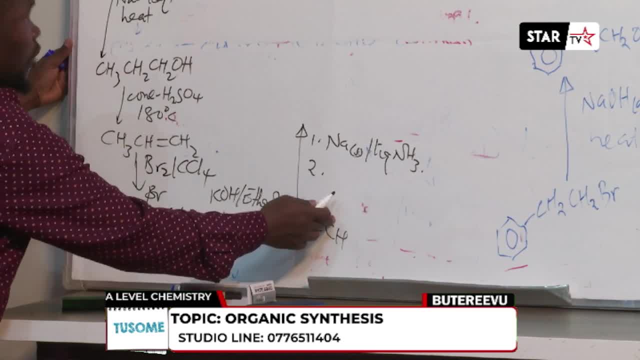 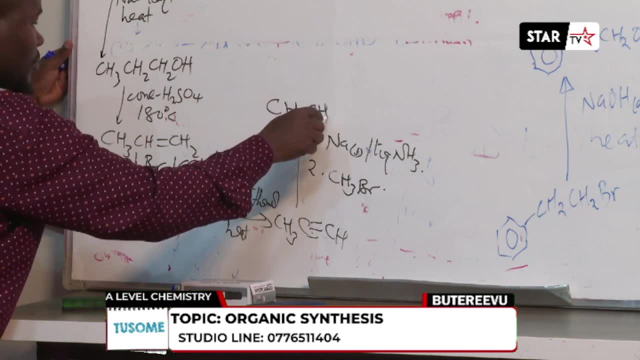 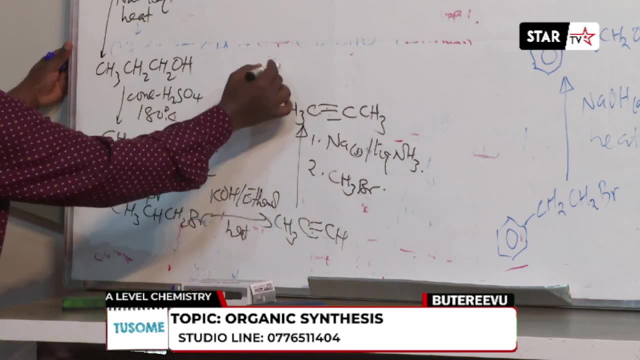 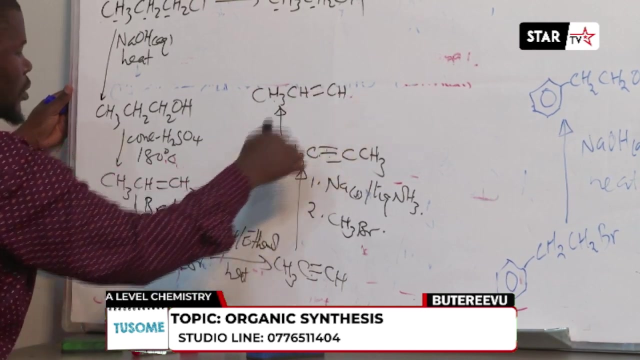 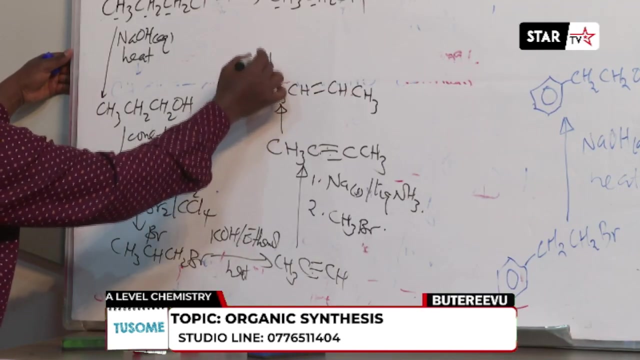 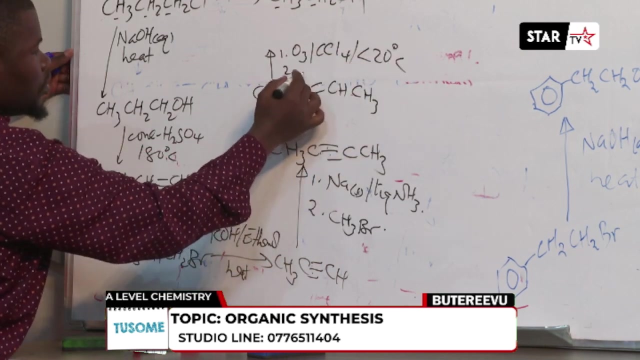 an acetylide. Step two: you add one carbon atom here And that will give you this kind of alkyne. That kind of alkyne can be converted to an alkene, to an alkene of this kind. And then you ozonolize. Step one: ozone, carbon tetrachloride less than 20.. Step two: you 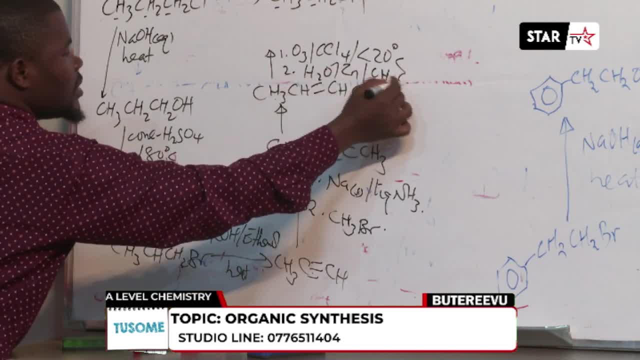 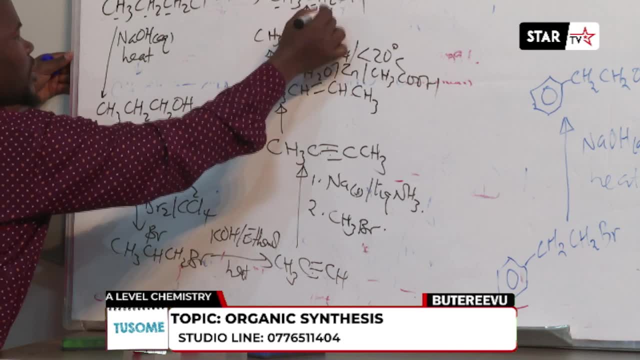 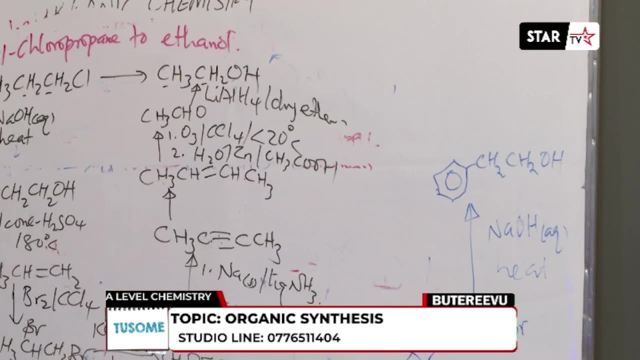 add water, zinc, ethanoic acid, That one gives you ethanol, which ethanol can then be reduced using a reducing agent. to give you that. These are how many steps? One, two, three, four, five, six, seven, eight steps, Probably. why am I doing this? I want you. 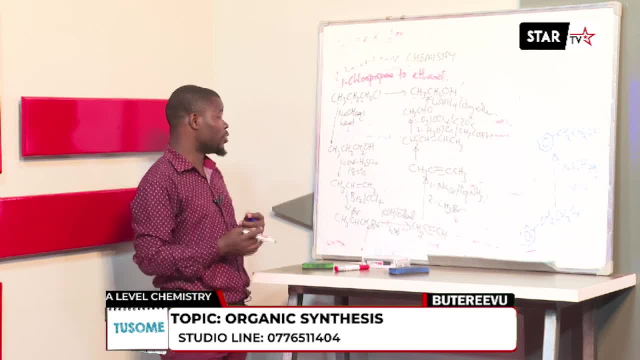 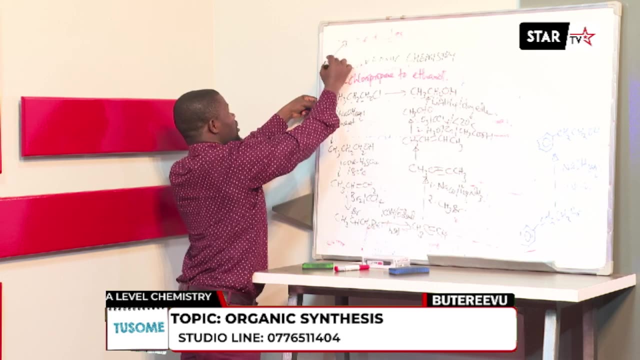 to stay at home and think of the shortest route possible that can take you there. You may probably be thinking of very many other routes that can take you here. Somebody could use this step. I have seen students always using this Potassium hydroxide ethanol. 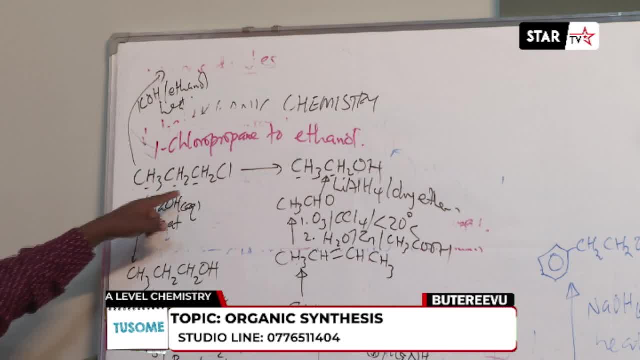 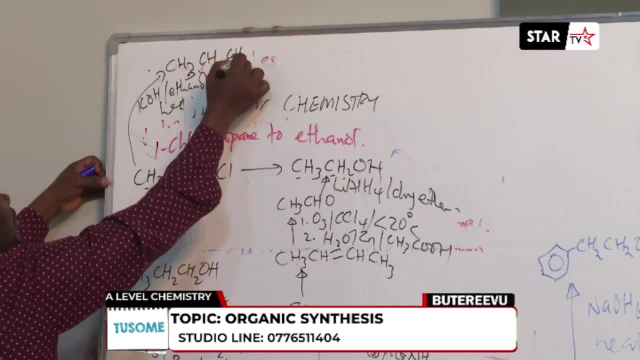 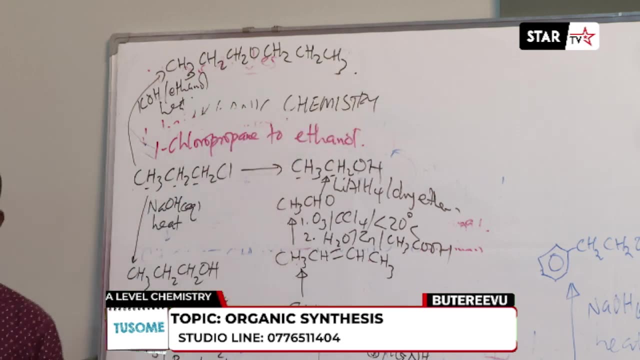 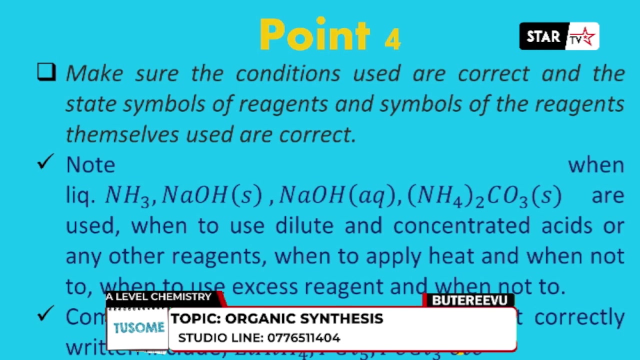 heat And such a reaction is likely to give you an ether. It's not appropriate for the synthesis, This being a primary, So you should avoid that. Let's proceed to the next slide. In our next slide we are seeing point four, which says: make sure the conditions used are correct And the state. 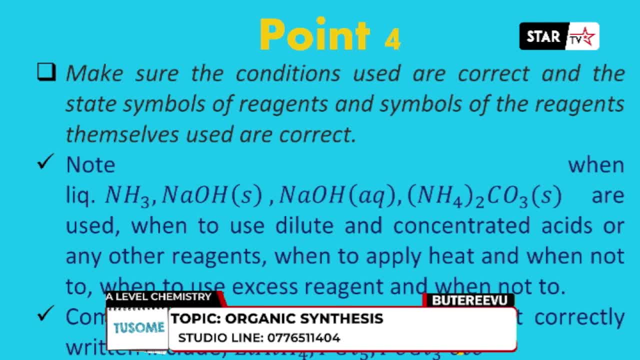 symbols of reagents and symbols of the reagents themselves are correct. For example, you have the carbon dioxide. This was included in equation two, So you take the carbon dioxide for the nitrogen oxide and clear the carbon dioxide. 부수부터, 부수부터, 부수부터. 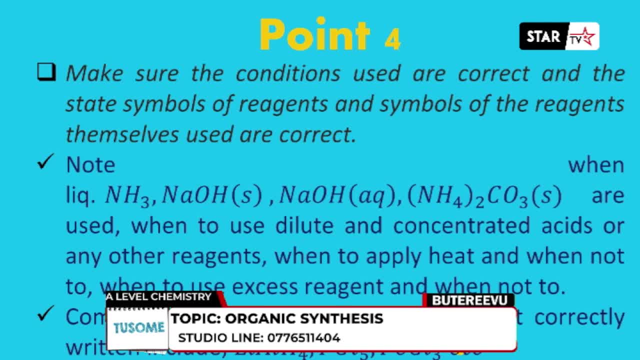 because하고 helping you to reduce using liquid ammonia in my conversions is here. It should be strictly liquid Because ammonia can be a solution. Know when to use sodium dioxide. the plotted on when to use acquiesce sodium. I drop now went to use solid ammonium. 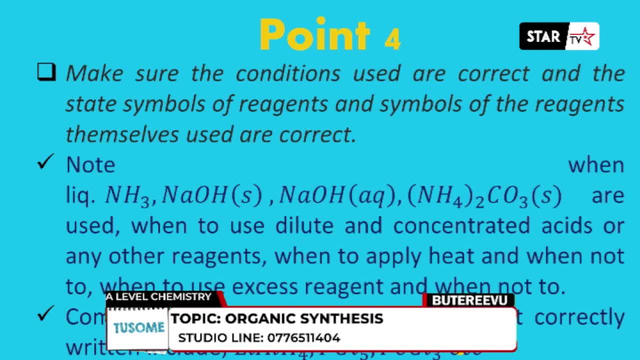 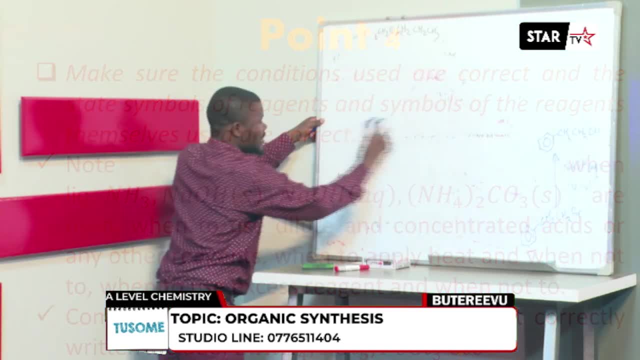 carbonate, For example, you have the carboxylic acid. I want to report it to a number, eight lower commissioning Asit and one to convert it to an amount. This is my carbazillic acid, This is my carbon dioxide acid And you can see this city. This isvoorcom, All right. 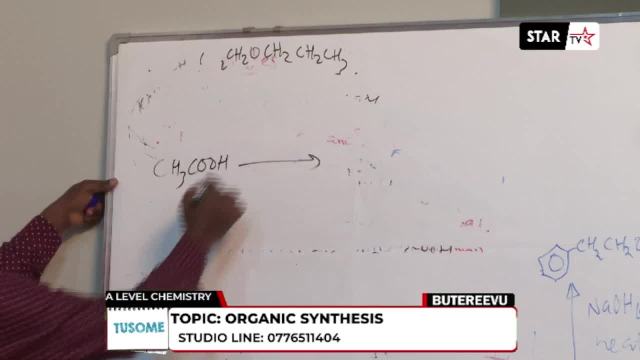 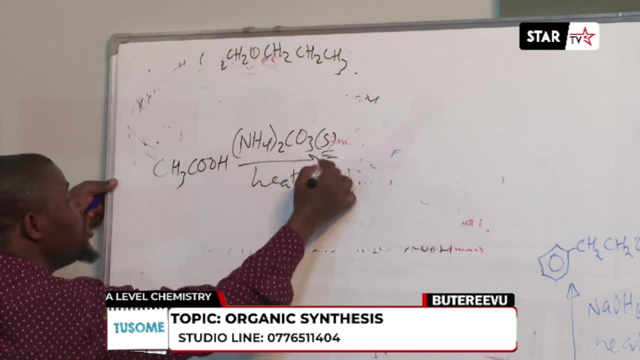 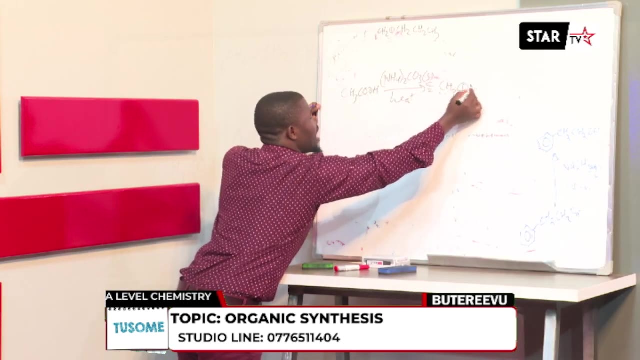 oxylic acid, ethanoic acid. If I want to convert it to anamide, I usually use ammonium carbonate and heat. This ammonium carbonate should be strictly less solid. Students usually mess up for such a case. This gives you ethanamide. 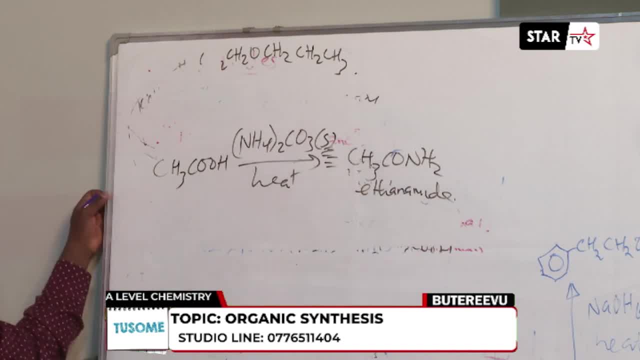 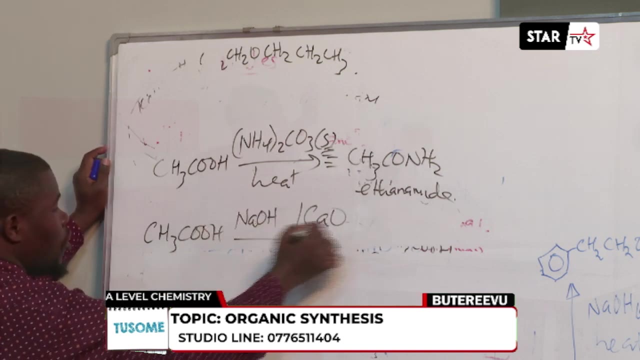 I'm emphasizing state symbols wherever they are required. Okay, You're using, you're doing a decarboxylation- Same carboxylic acid and using sodium hydroxide, calcium hydroxide, and then you're heating. This should be strictly. 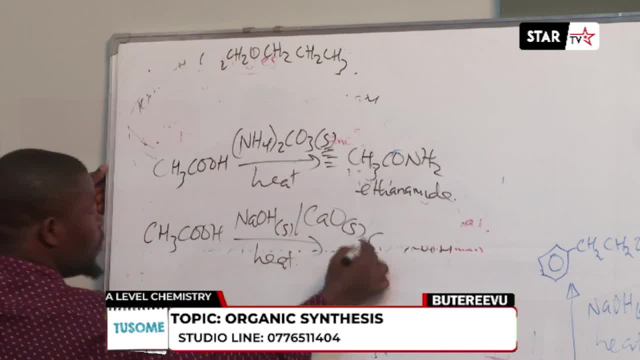 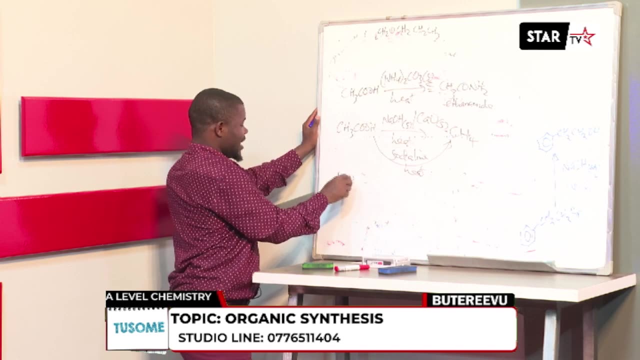 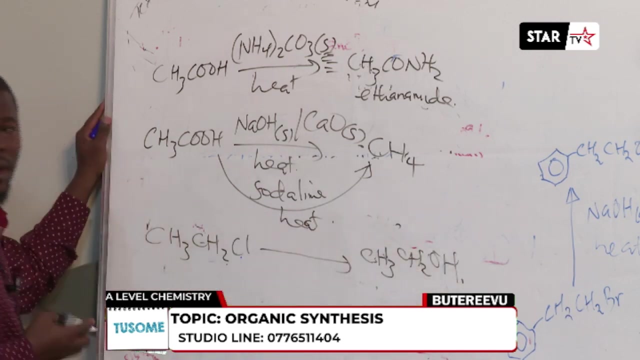 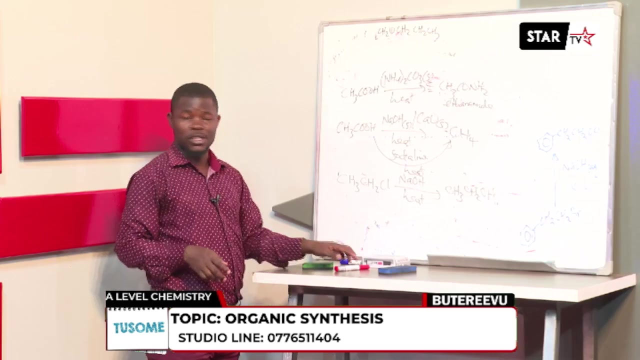 less solid to give you methane. But why do you go this way? Yet you can simply write the word sodaline and heat. Okay, You're converting an alkyl halide to an alcohol. Use sodium hydroxide, heat. Now, when you do that, you're not specific. The sodium hydroxide is it solid or liquid? 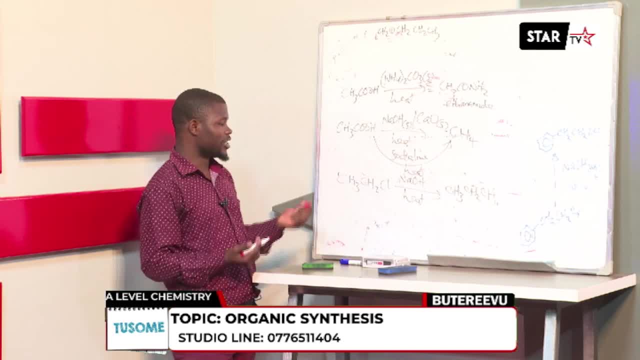 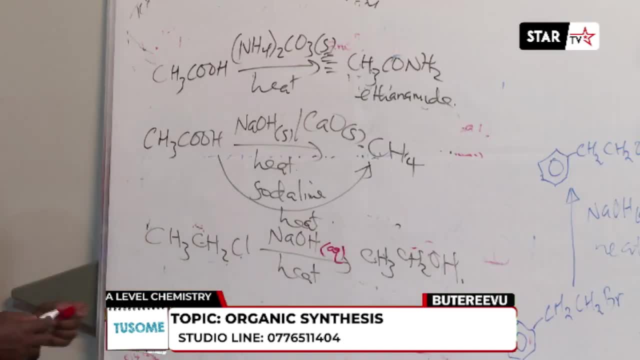 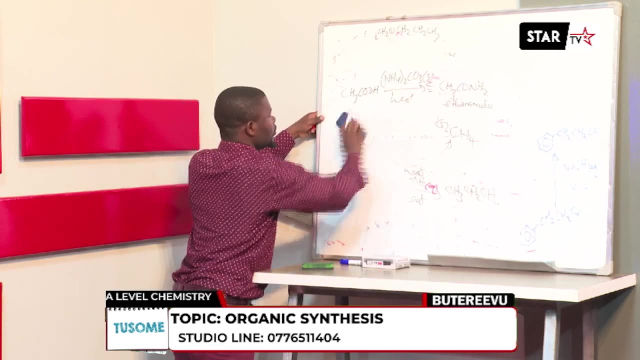 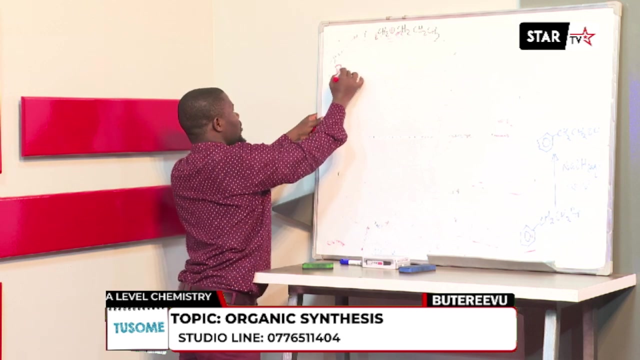 Sodium hydroxide can be a liquid. when heated to melt, It can be a solution. It can be a solid in pellet form. So please specify that this is aqueous. You have seen a conversion of this kind. Somebody can tell you to convert benzene sulfonic acid, Benzene sulfonic acid to. 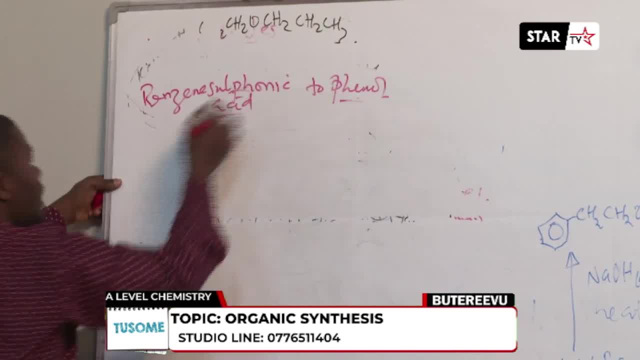 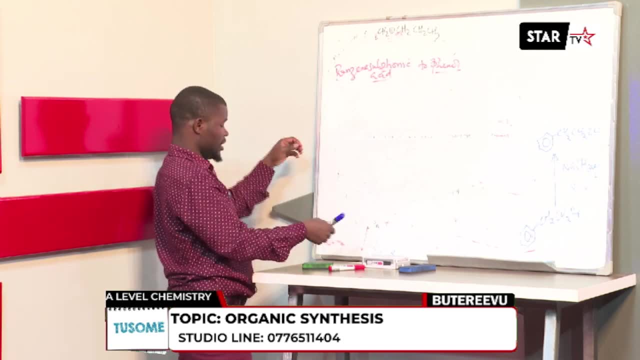 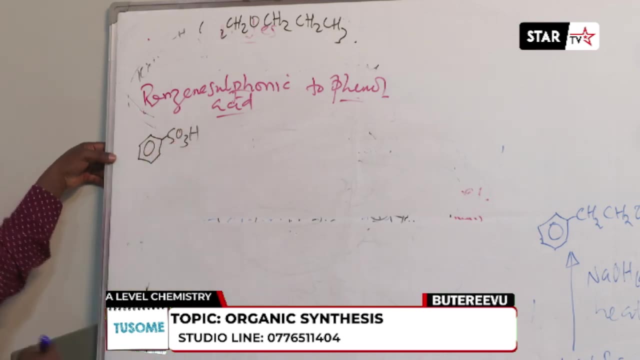 phenol. This is where most students mess up with their state symbols. What do you usually do in this synthesis? What you should always do is this: Get the benzene sulfonic acid- It is that compound- Sodium hydroxide aqueous at first. When you use aqueous sodium hydroxide at this step, you will. 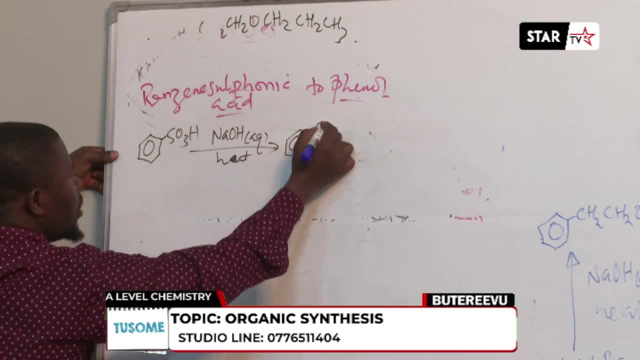 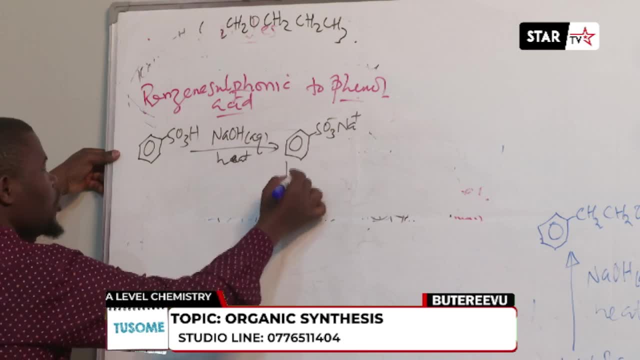 get a sodium salt of the acid and then, in the second step, what we usually use is a sodium salt of the acid, And then in the second step, what we usually use is a solid sodium hydroxide. I'm emphasizing states and their 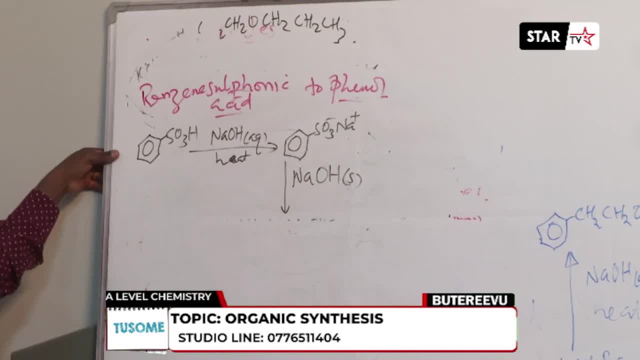 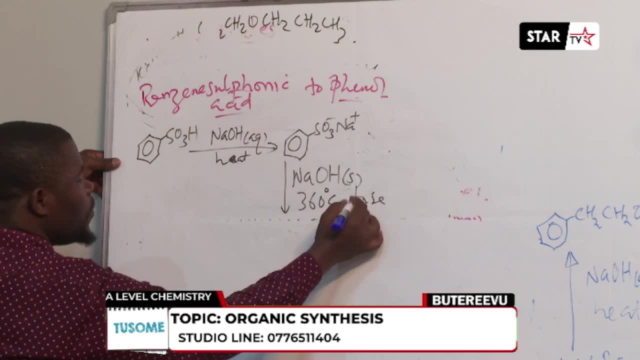 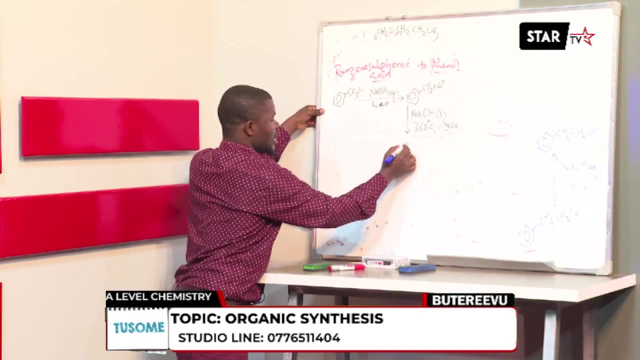 importance. In the case you don't specify which sodium hydroxide you're using, then you have challenges. This occurs at a temperature of 360 degrees Celsius and we fuse Fusing means we are using solid sodium hydroxide. At that point we 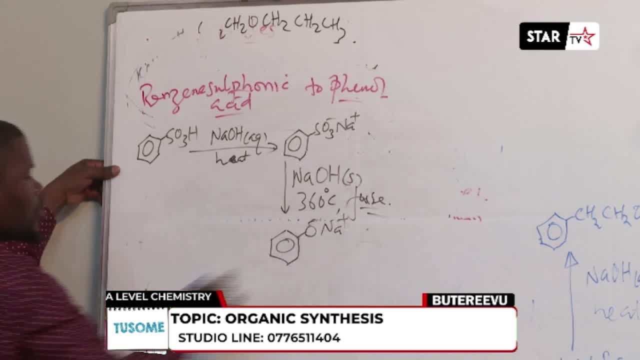 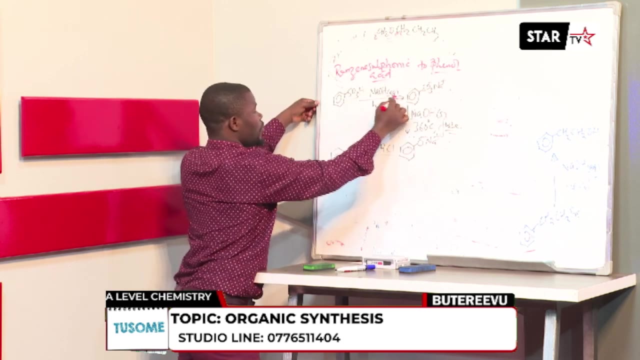 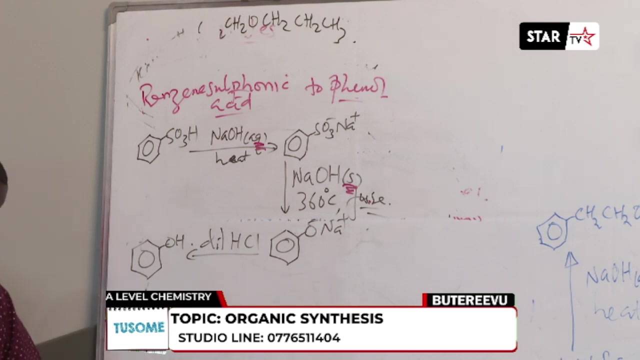 get a sodium salt of phenol, sodium phenoxide, which you can simply dilute with hydrochloric acid to finally come up with your phenol. Why have I done this? I'm emphasizing the importance of steady symbols, my dears. Next slide, When you 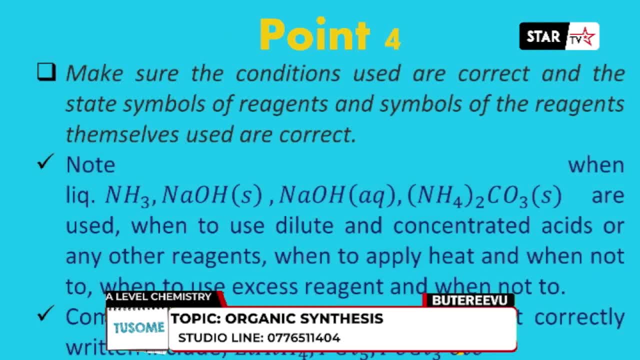 look at that slide on your screen. you're seeing point. that is point four. next slide: You should know when to apply heat and when not to. You should know the common reagents whose symbols are not written correctly. People usually write symbols. 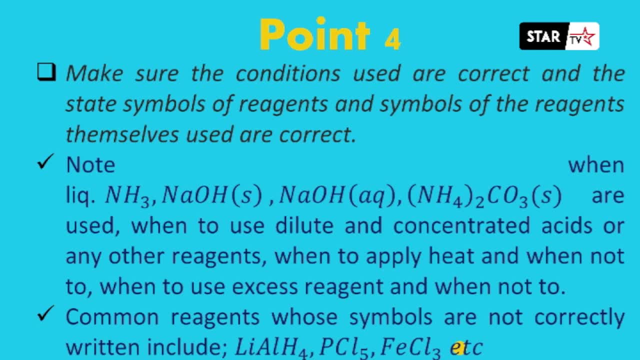 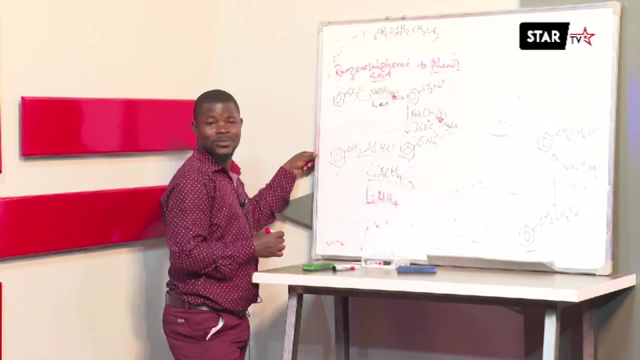 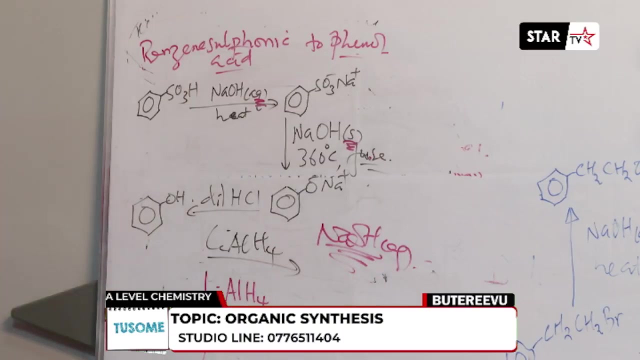 wrongly. Somebody is writing lithium, aluminium tetrahydrate and it does this. Who are you chasing? This is not letter L, and in chemistry we are always tricked with chemical symbols. Write letter L very well, You're not chasing anybody. Sodium hydroxide: I've seen people do writing these things. You're not chasing anybody. 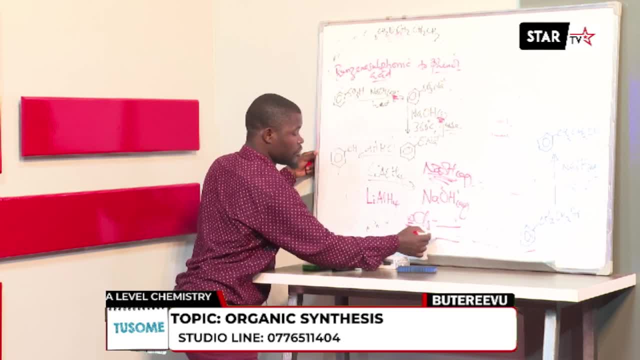 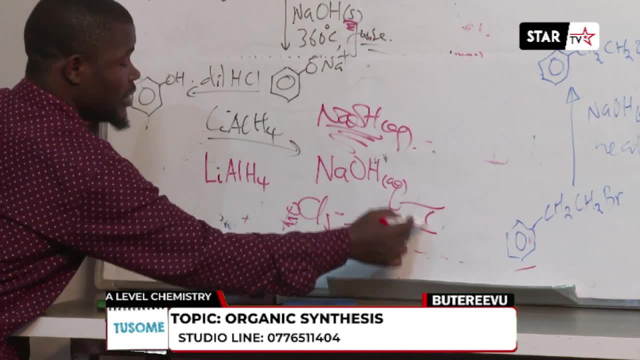 1. P, P, P. 1., 2., 3., 4., 5., 6., 7., 8., 8. write p like this. this is a small, a lowercase letter p, and for us here we're always interested. 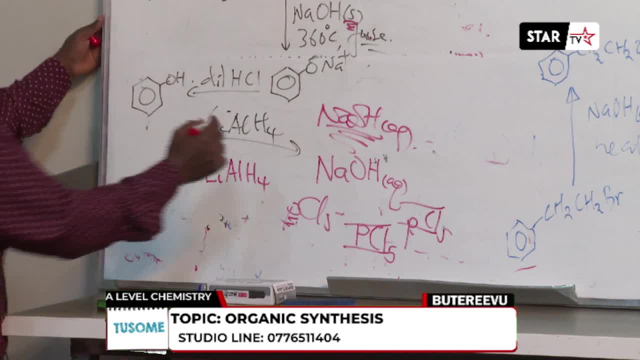 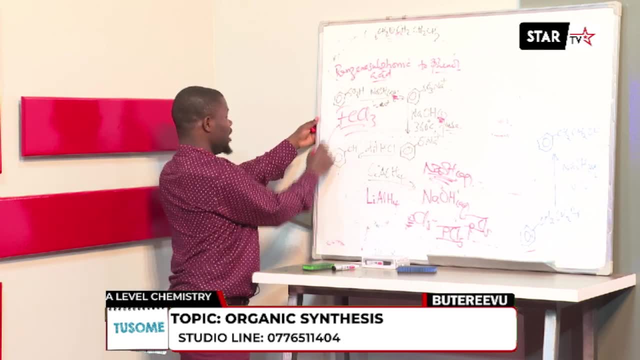 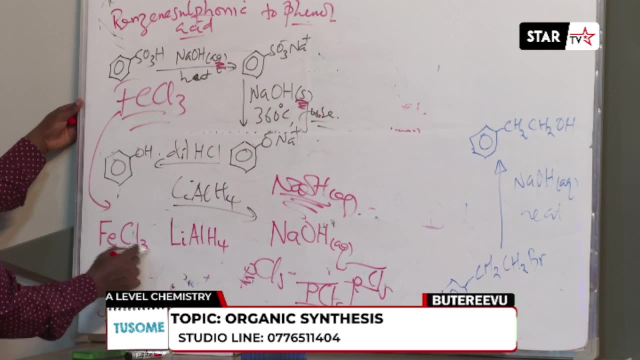 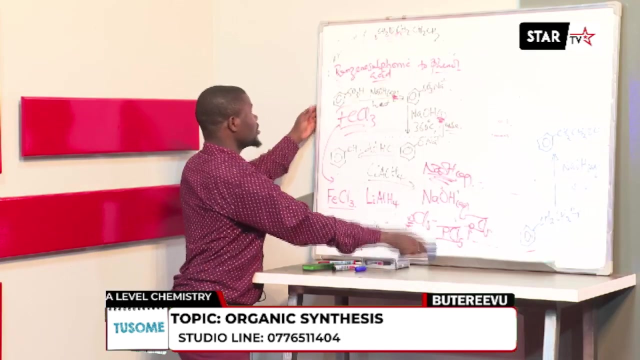 in symbols. please make sure you write correct symbols. somebody's writing any three chloride. let's be careful, my dear students. okay, write iron. very well, iron three chloride. you're not chasing any person. okay, we can move to the next slide. you can move to the next slide. 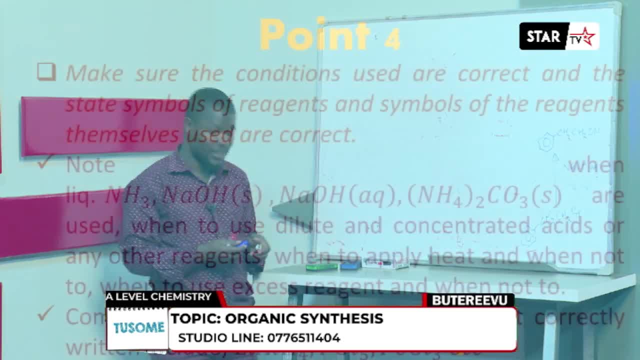 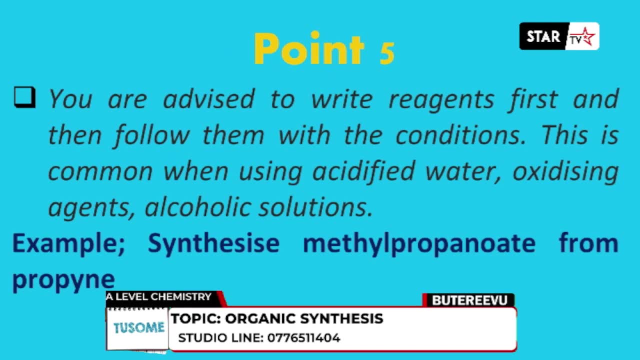 in our next slide we are seeing another point in organic synthesis, point five. let's proceed. point five said you are advised to write reagents first and then follow them with the conditions. this is common when using acidified water, oxidizing agents and alcoholic solutions. okay, don't write. 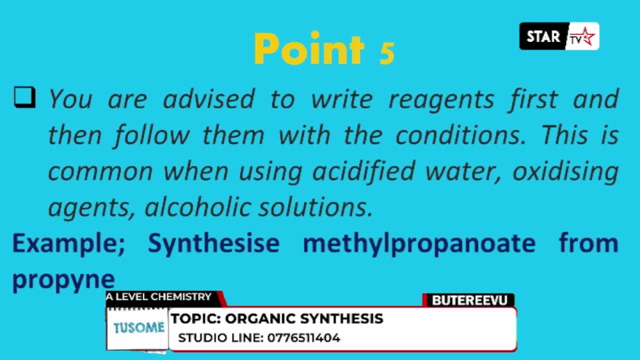 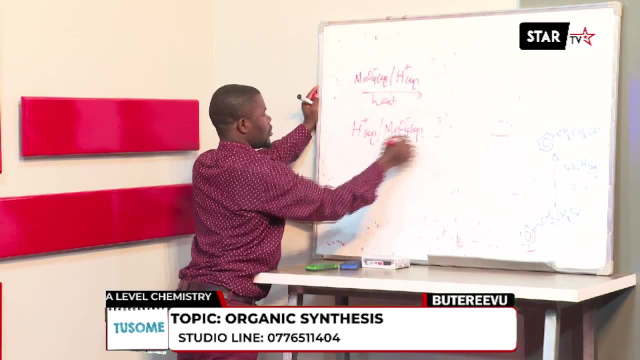 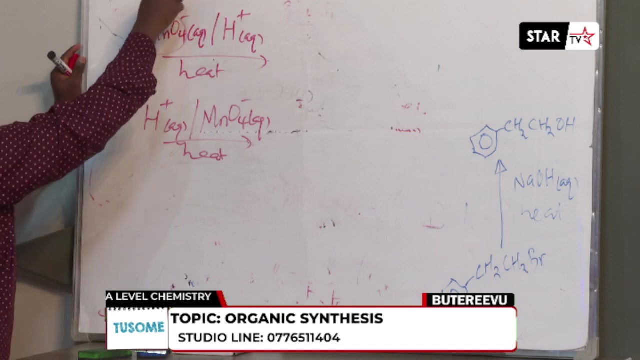 for example, using acidified potassium permanganate. you're writing that reagent and using it in synthesis. i've seen people writing it this way. i always advise students to write the first. this is the reagent. the potassium permanganate is the reagent. the acid is just. 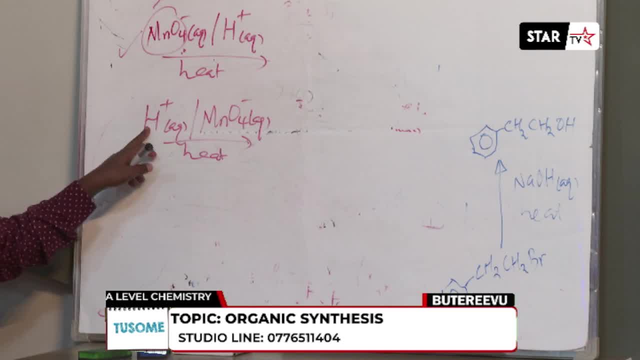 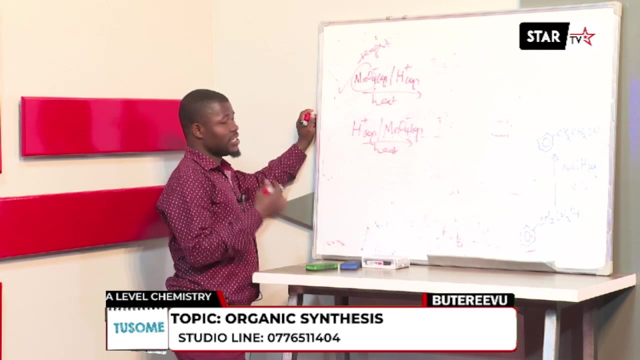 a condition to acidify it. don't begin with the acid and then write the. don't begin with the condition and then write the acid. for example, you are using a um alcoholic potassium hydroxide solution. okay, you should write the reagent first. the reagent is potassium hydroxide. 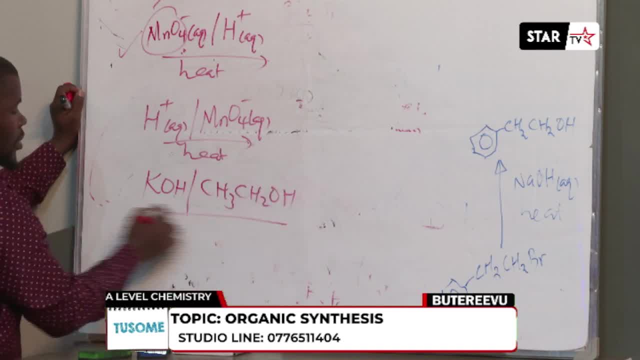 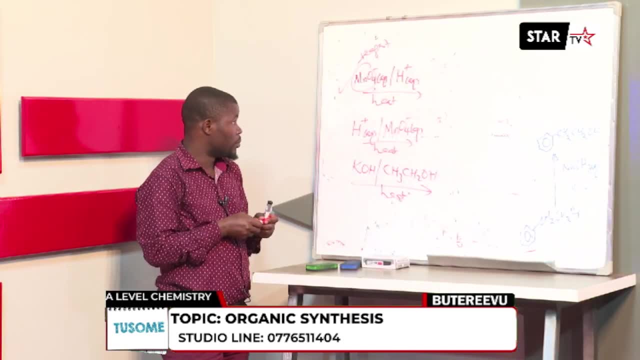 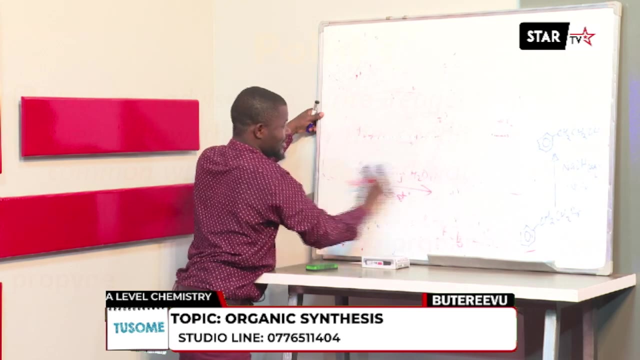 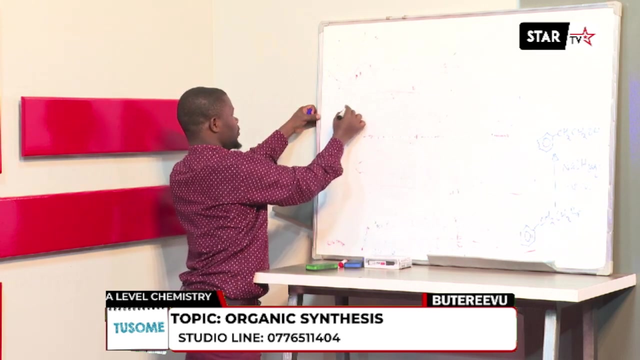 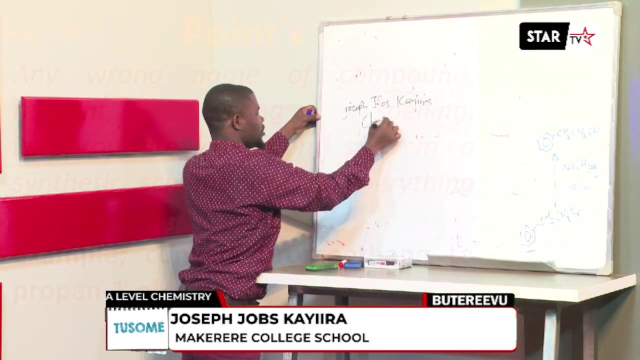 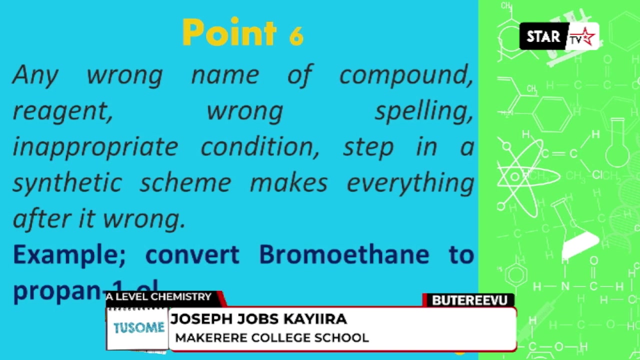 and then ethanol is just a condition. then you hit in a synthesis. let's proceed to the next slide, point six. thank you for viewing us members. you can get more on my youtube channel, which is joseph jobs kaira chemistry channel. there are very many lessons about chemistry. uh, we are synthesizing. let's rewind. there is a synthesis we are doing. 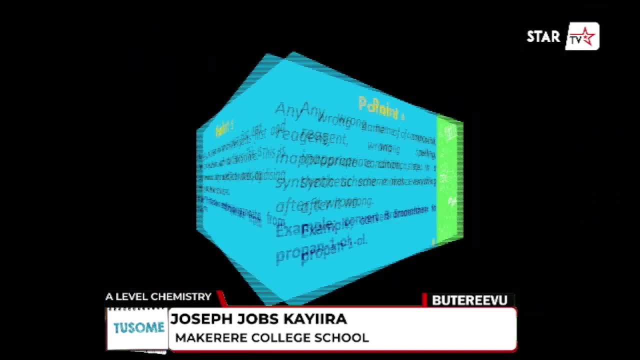 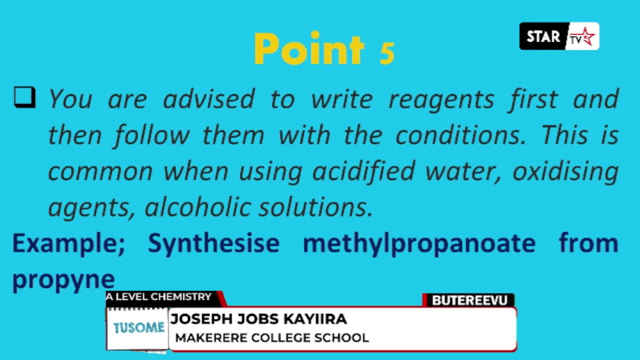 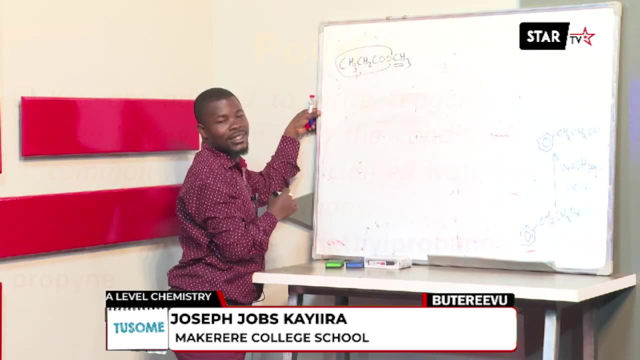 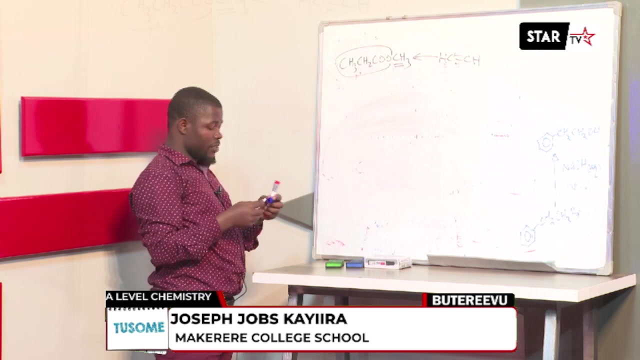 point five. there is a synthesis there. uh, that synthesis is methyl propanoate from propane. methyl propanoate- this is methyl propanoate. we are getting it from a time. How do you convert methyl propanoate from ethylene? Look at these two carbon atoms. 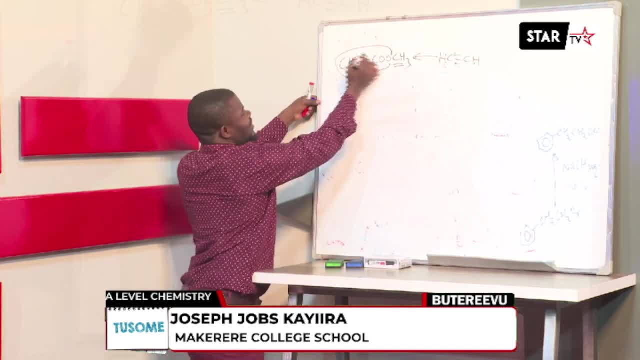 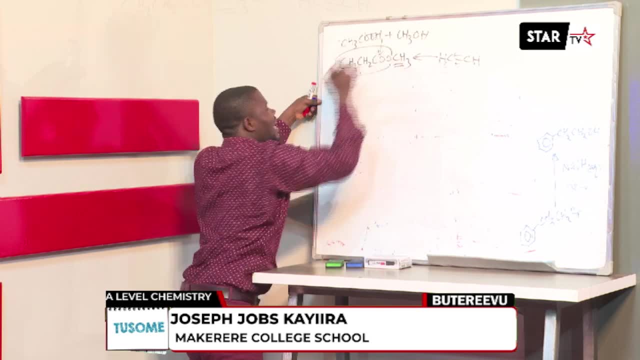 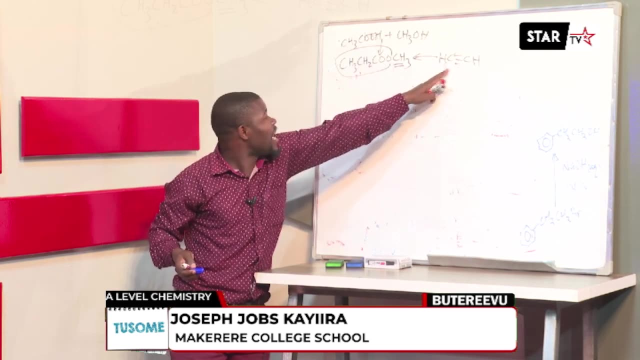 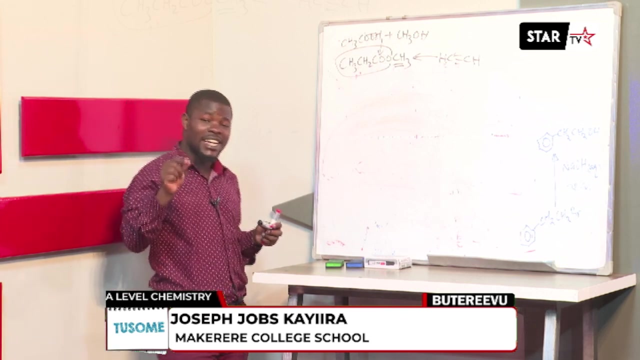 You must of all get ethanoic acid, Which ethanoic acid you will esterify with methanol to get this ester. You see how chemistry is interesting. So you must think of how do I get from ethylene to ethanoic acid. To get ethanoic acid from ethylene I must get ethano first. 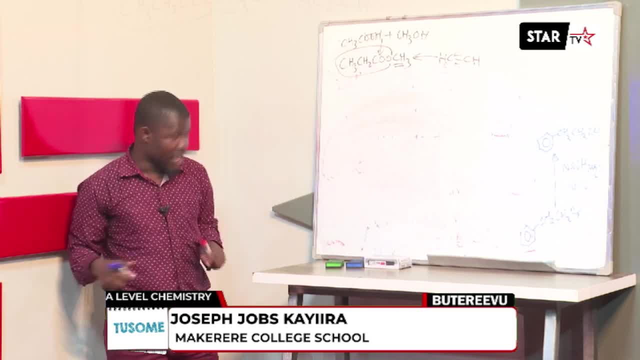 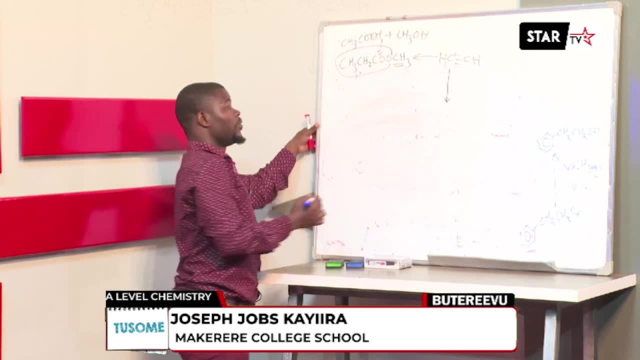 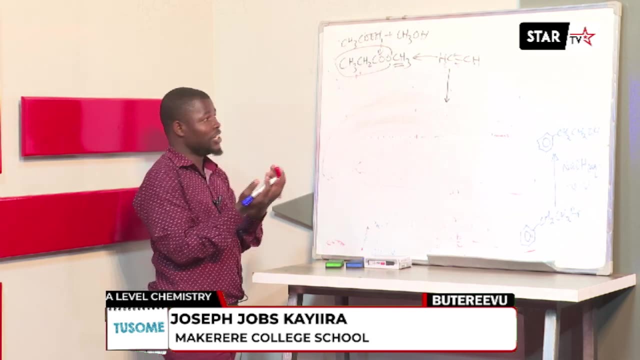 Which ethano I will oxidize. Dear viewers, what do we do? Convert the ethylene to ethano. To convert ethylene to ethano, you first of all convert it to ethene. How do you get ethene from ethylene? 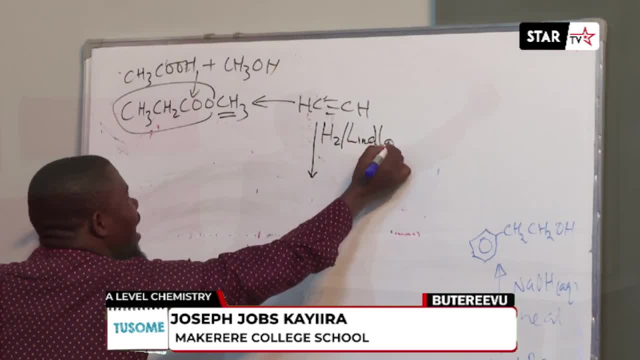 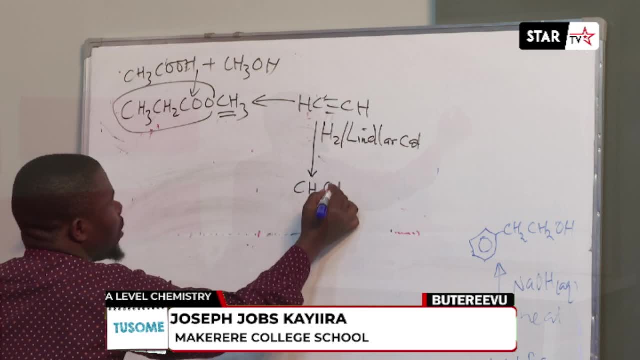 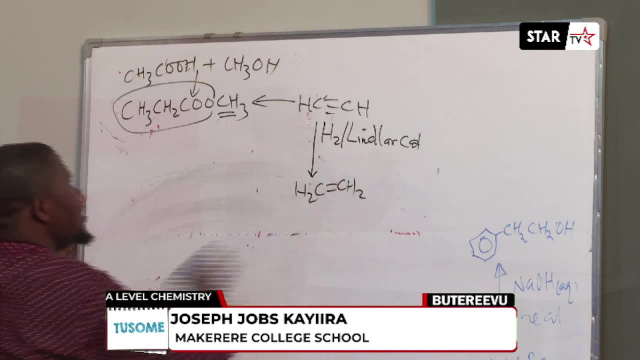 You first of all convert it to ethene. How do you get ethene from ethylene hydrogen? in the presence of lindelar catalyst, that will give you CH2, CH. it gives you an alkene which is H2C, CH2. that is a thin. some people I have seen 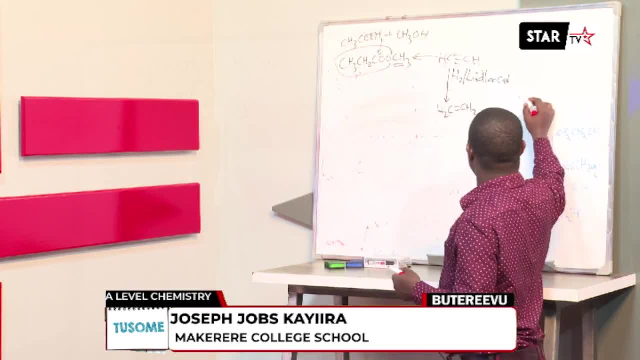 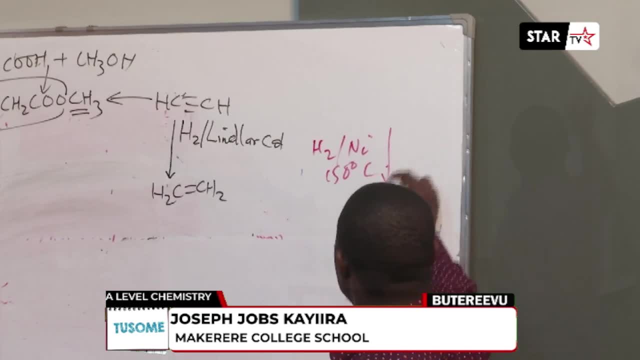 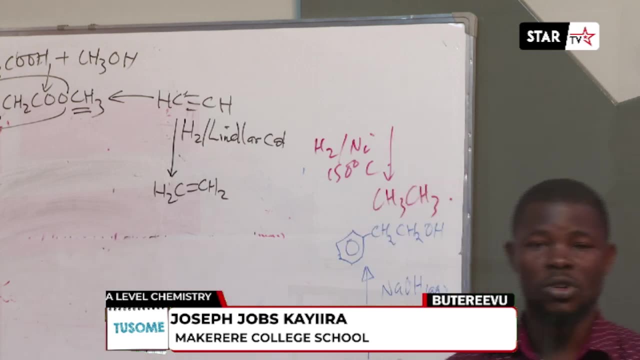 them using this. they use hydrogen in presence of nickel 150 to do that conversion. when you do that you're likely to get an alkane. it will be very hard to for you to isolate the alkene, so you may not easily isolate the alkene from the mixture. to avoid that, we poison the hydrogen with what I told you. 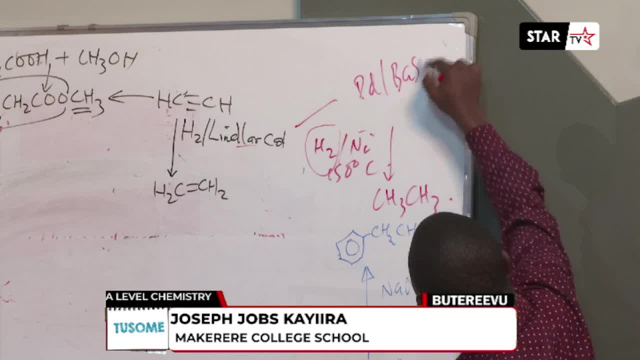 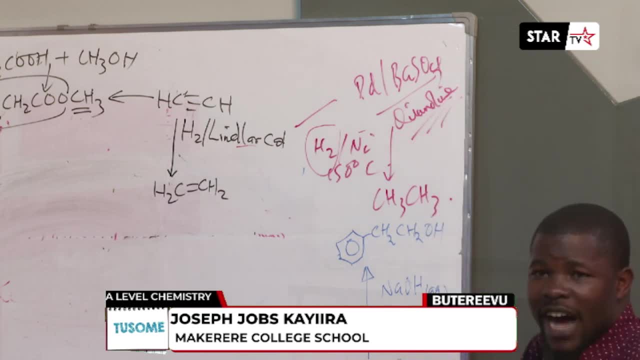 lindelar's catalyst is palladium supported on barium sulfate and quinoline is the poison. why do we poison the catalyst? to slow down the conversion of the hydrogen. and to slow down the conversion of the lindelar's catalyst is palladium supported on the mixture. to avoid that, we poison the hydrogen. 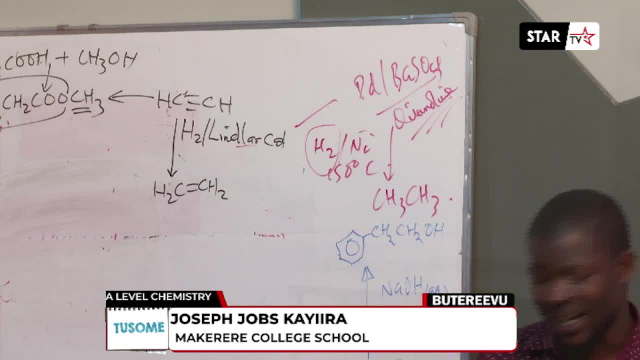 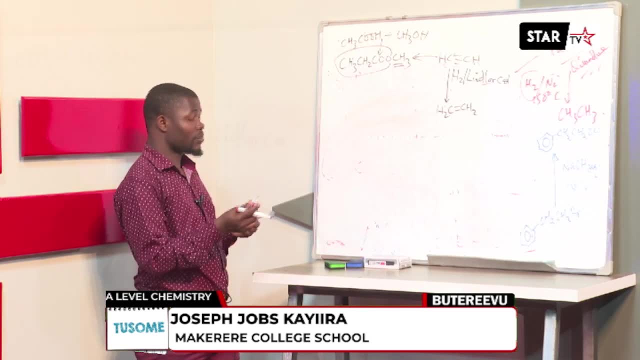 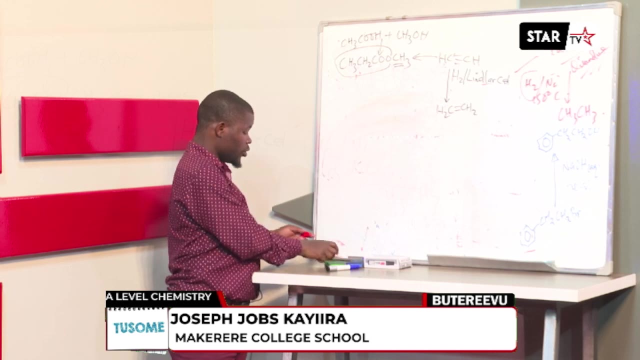 down the conversion of the alkane to the alkene. so when you do that, you'll get the alkene instead of the alkane. now that is, the lindelar catalyst is simply that mixture there. so what do we do after getting a thiol? I know you can now. 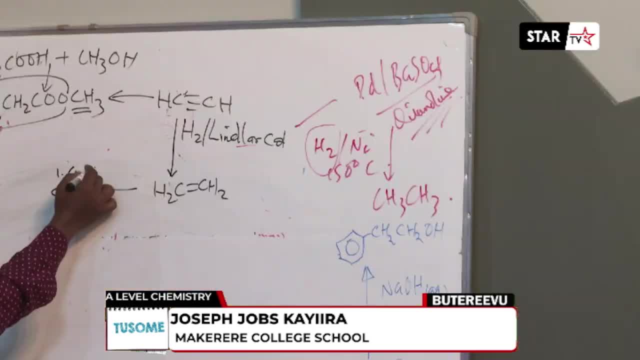 proceed by using step one co-onco sulfylic acid to water, uh salt to bind to the isethyl in order to kill this methylation. so they are taking a thin process to form a thin, a thin profile. so all the valentine that we can do is to put it in water. I know you can now proceed by using step one co-onco sulfylic acid to water. 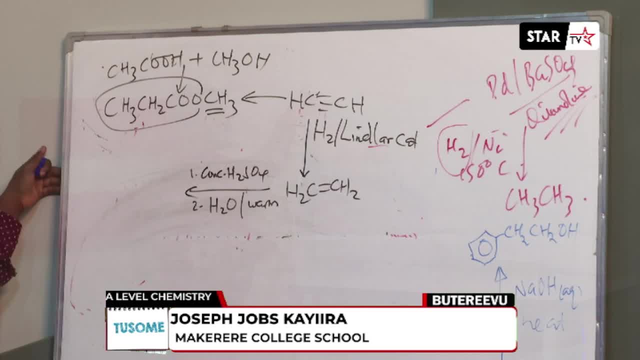 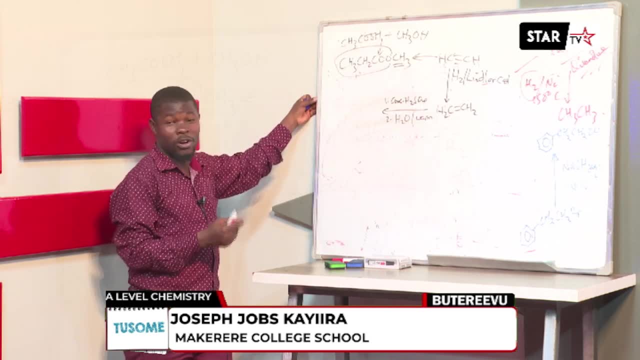 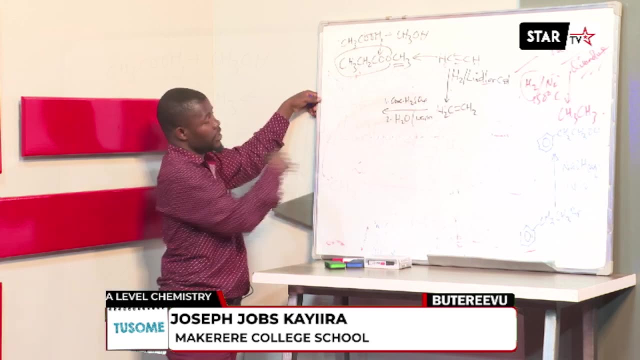 and then warm. now people are getting confused. what does that mean? this is what you have always been calling acidified water. you write acidified water, but it usually occurs in two steps, doesn't occur in one step, so I've liked to separate it this time. but even if you use acidified water and warm, that's fine. 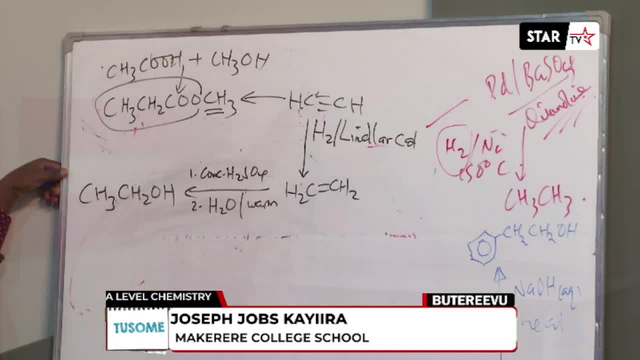 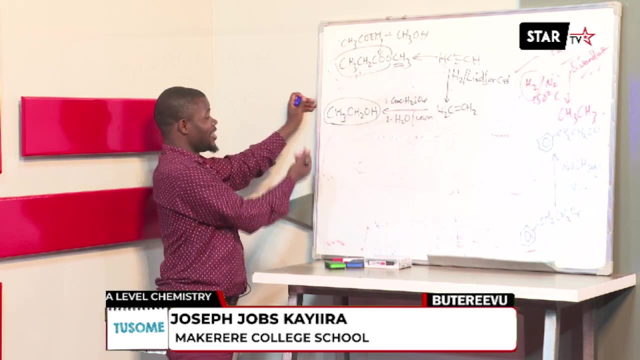 this gives you ethanol. this gives you that enjoyable drink that probably some people are taking this morning. people are working, people are on business, then people are sanitizing their throats. people say the ethanol sanitizes their throats and I stops COVID. I don't know the proof. I'm still in the lab trying to. 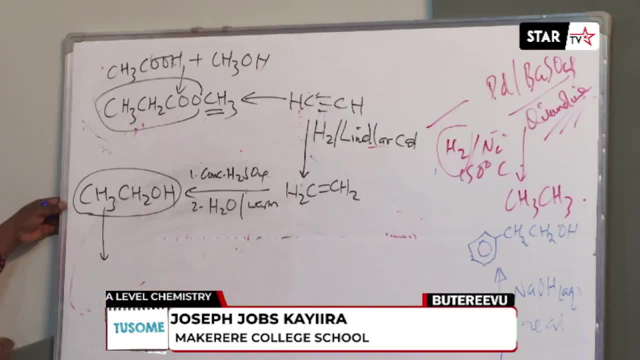 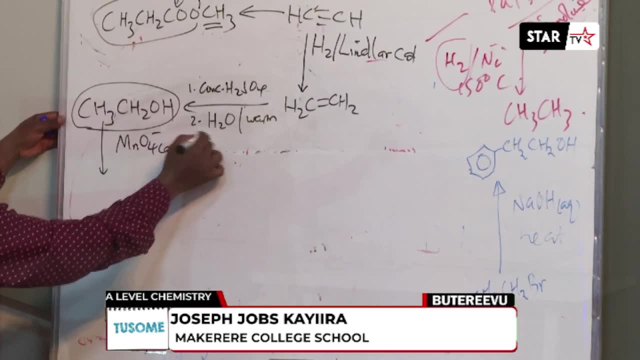 to prove that now, after getting ethanol, you can oxidize the ethanol using an oxidizing agent, potassium permanganate. in the presence of the condition now, the acid, you must heat. when you heat this drink, you will get a lot of oxygen and you will get a lot of oxygen in the 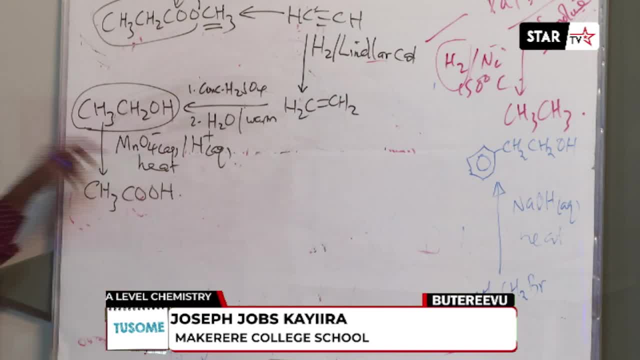 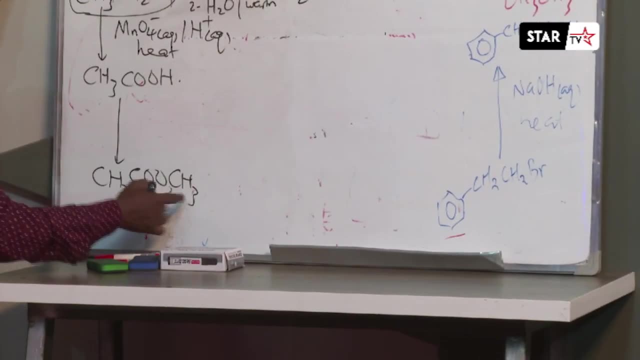 tea. so when you're boiling the tea, the standardized, you will get a lot of water. therefore you must prepare when you operate the oestrogen and other substances. take us, for example, I have na up it as much is very high in thisiguainer. so this hospital, to get water from tea at the pH 100, at 1000, you only have to. 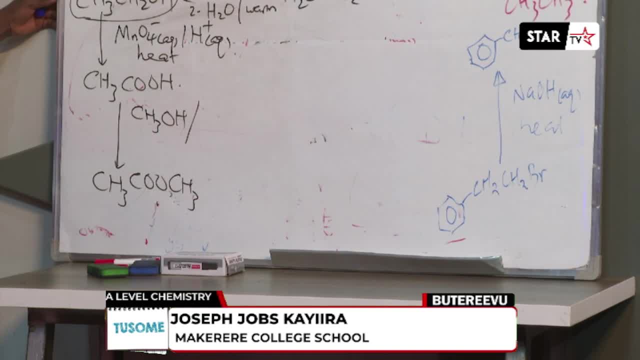 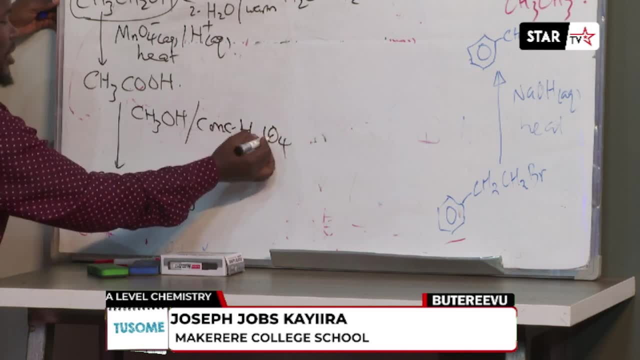 chance and also instant 발 상태 meantime, which will take less time to chill- about half an hour. so after you are cold you want to cool down if you are buying something both in hot or cold. I said today I brought the cast orders sulfuric acid and please, this reaction is very slow, so make sure you heat to. 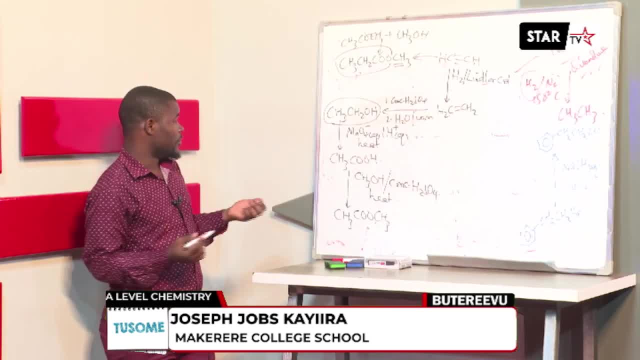 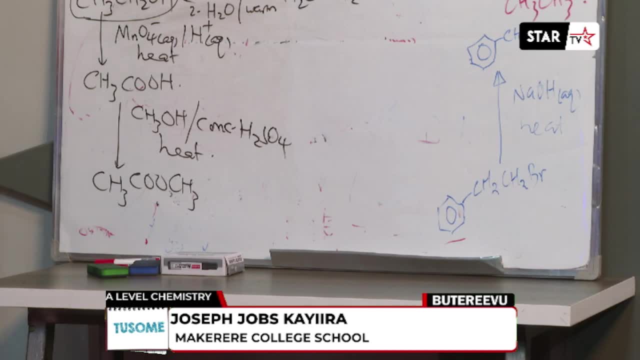 make it occur faster. what have I been emphasizing here? reagent first condition. reagent first condition, next slide. oh sorry, this is not yet. we are saying methyl propanoate. we are saying methyl propanoate, we must have three carbon atoms. I think I need to correct. 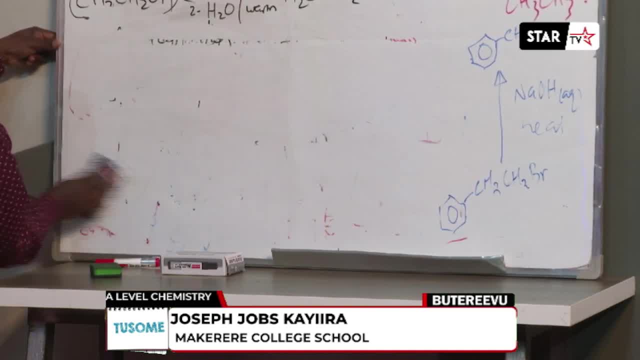 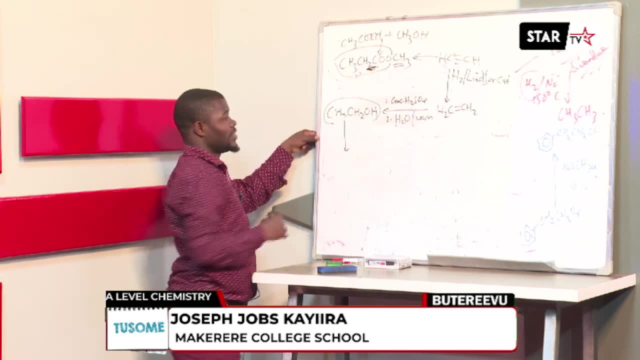 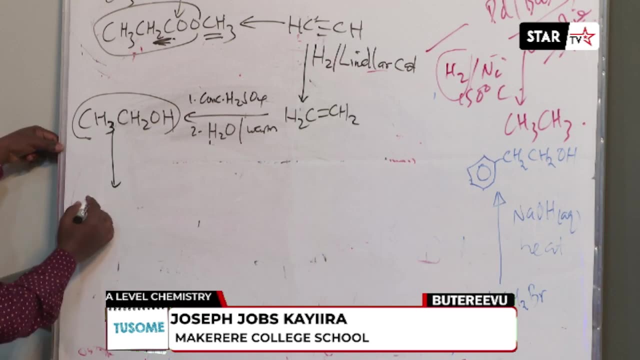 this. I'd seen methyl ethanoate. so how do I get methyl propanoate from this? we must add one carbon atom here. we must add one carbon atom. I didn't see this. sorry for for that error. so what do we do? we get the alcohol and convert it to. 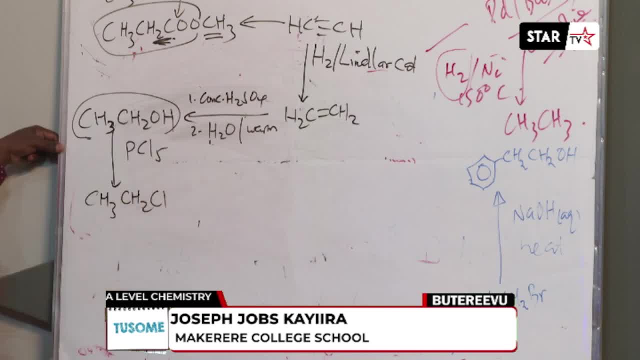 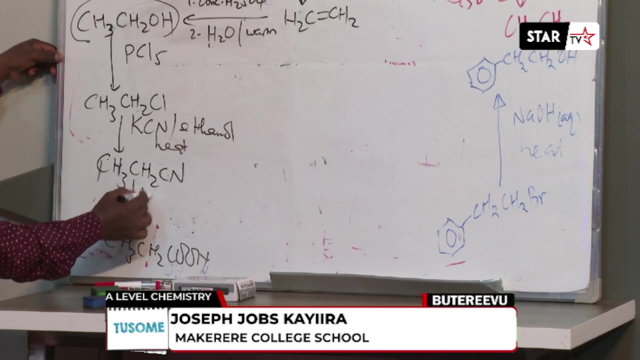 an alkyl halide using phosphorus pentachloride and then you use potassium cyanide to give you this. use potassium cyanide in the presence of ethanol and then heat. it gives you that. then you can go to propanoic acid. the propanoic acid is got by using acidified water at this step. 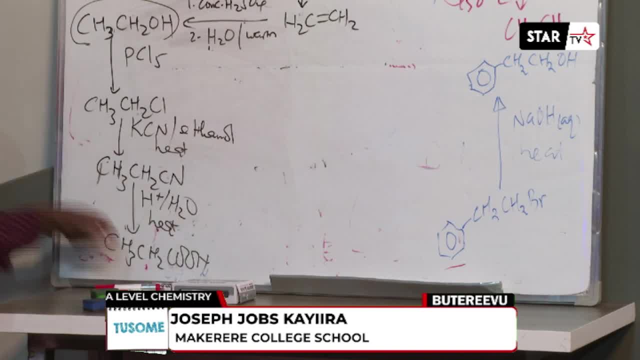 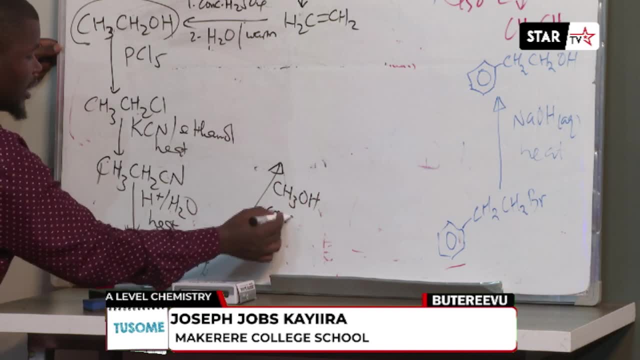 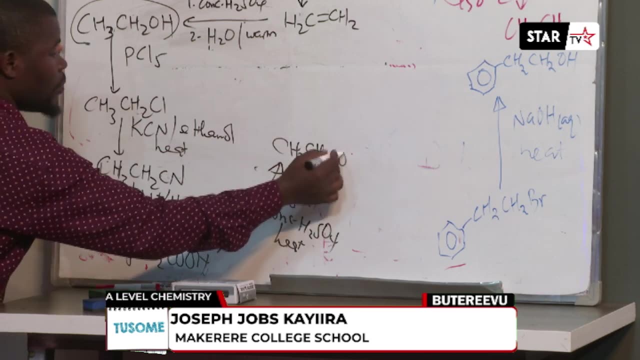 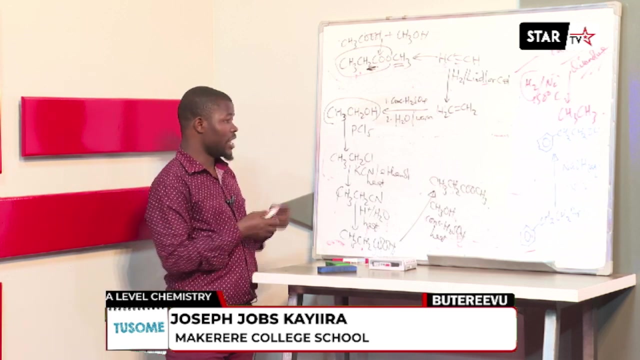 and then we heat. so after getting the propanoic acid, then we do our last step, which is methanol, quarks sulfuric acid, heat that gives you methyl propanoate. thanks for viewing and learning. we are in our program to some, once again remind you, and we 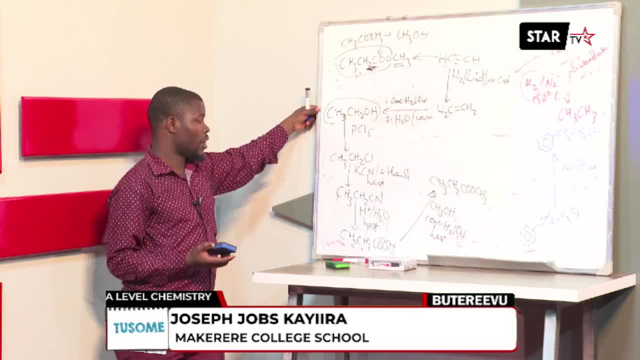 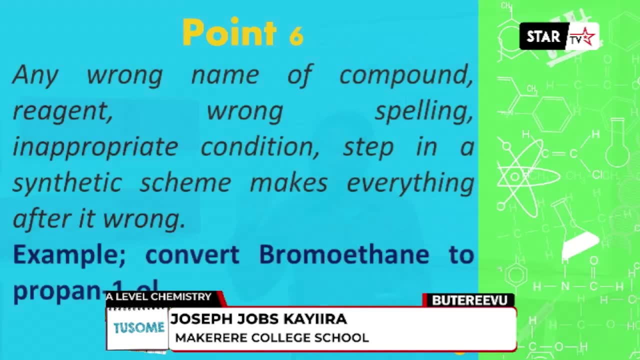 shall always be doing these enjoyable lessons. okay, so we proceed to our next slide, which is a point six. any wrong name of the compound reagent, wrong spelling, inappropriate condition, any wrong step in a synthetic steam scheme makes everything after it wrong. let me give you an example. we are converting bromothane to propane. one all. 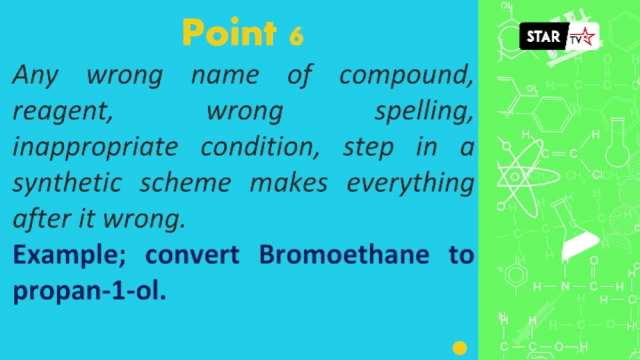 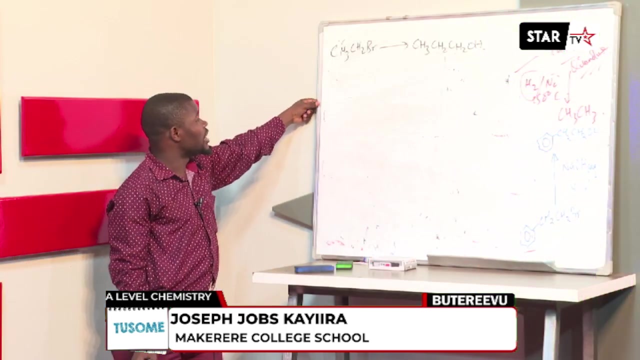 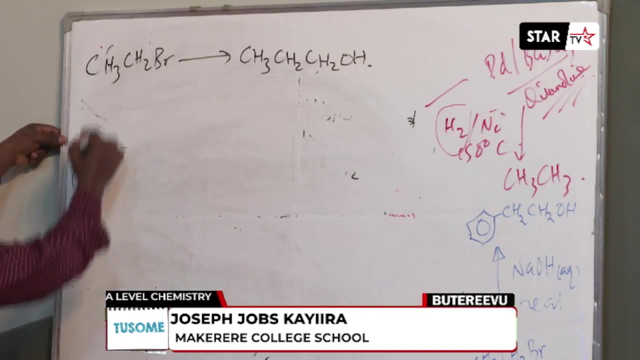 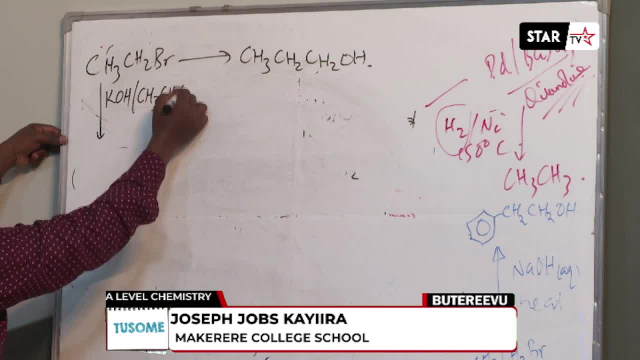 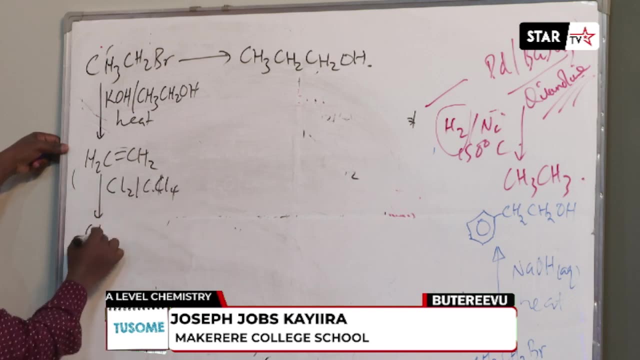 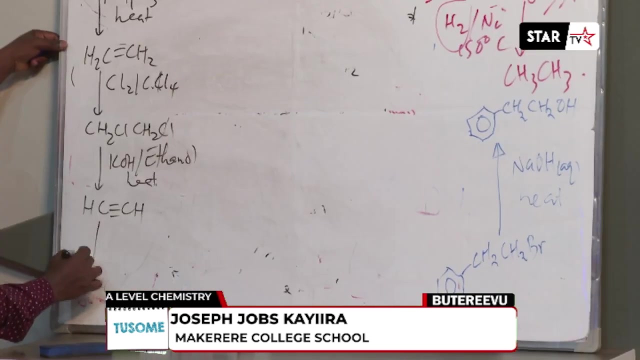 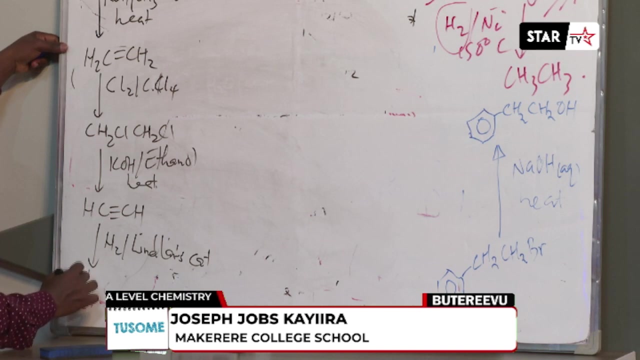 student one is there and he's thinking of this. somebody is seeing that. student two: the student is getting a thin and then he proceeds using uh chlorine, carbon tetra chloride, CH2 chlorine atom, then uses potassium hydroxide ethanol again and the student is heating to get a thiene. That student is using hydrogen lindela to get a. 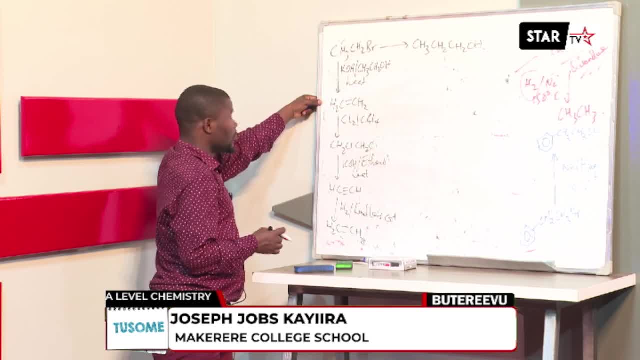 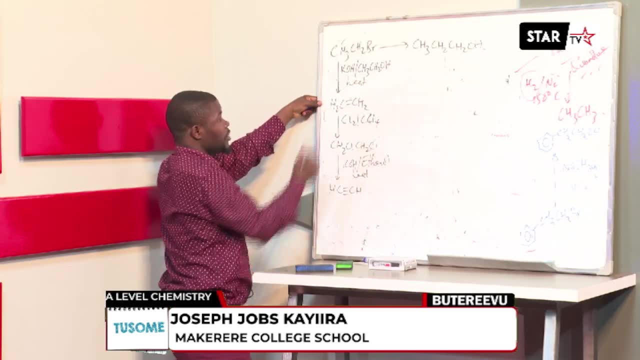 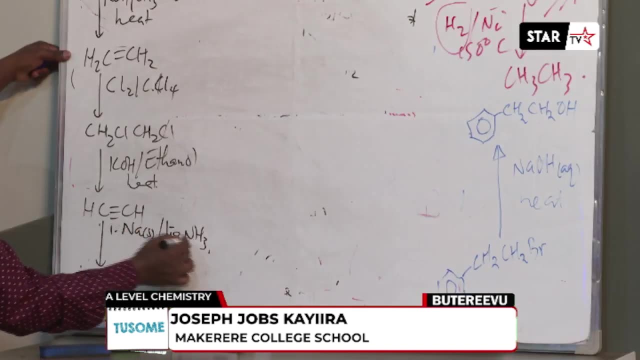 thiene to get a thiene, Or the student may prefer to elongate the chain at this point to get the three carbon atoms by using step one, sodium, liquidy ammonia. The same student is now adding one carbon atom, because those are three. 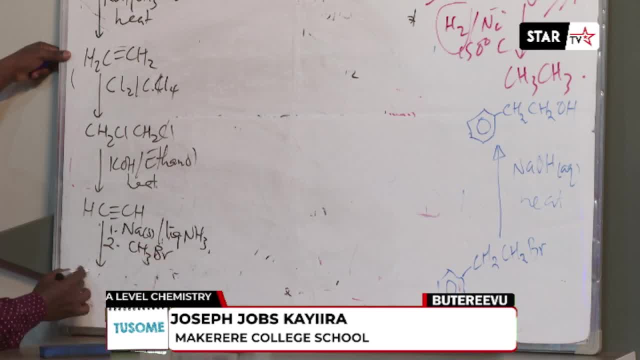 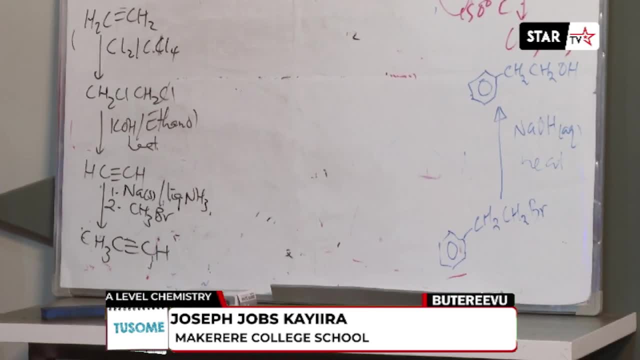 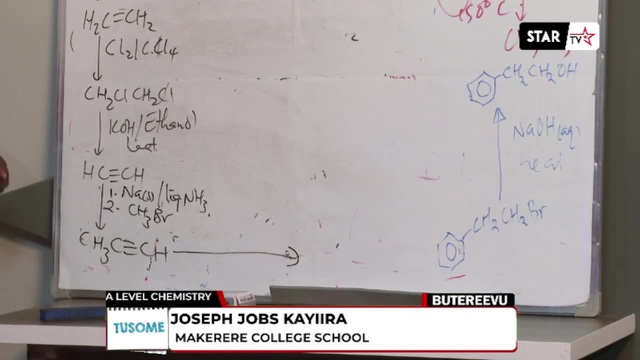 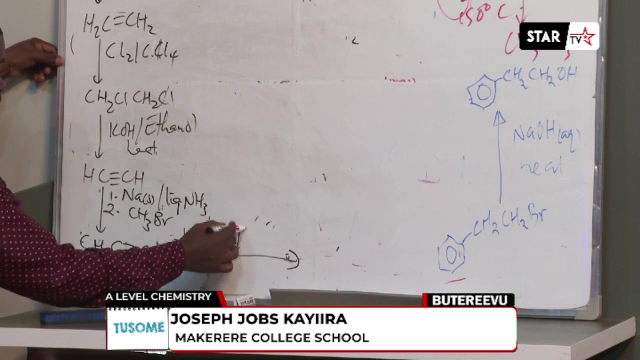 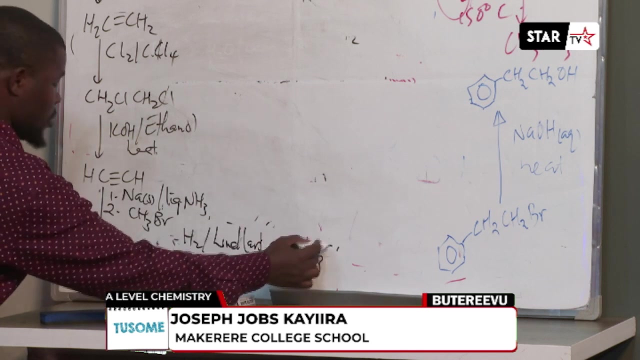 CH3Br, That student now gets CH3CH3.. This should be a terminal alkyne to do that conversion. The student continues enjoying the synthesis. Okay, So the student continues enjoying the synthesis, then uses hydrogen- again lindela catalyst- to get the alkyne. 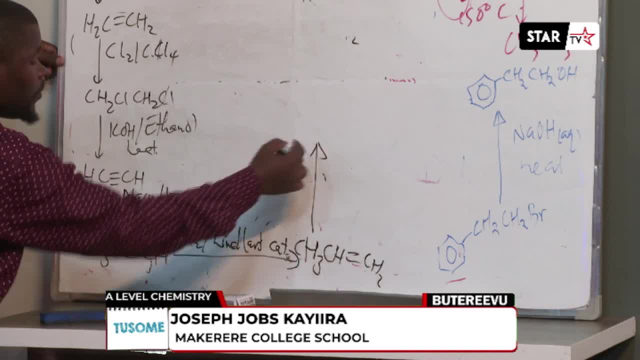 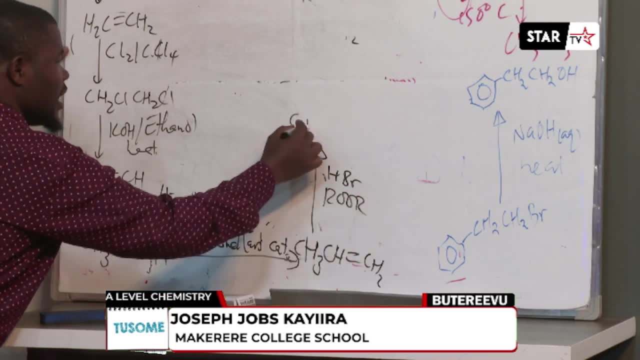 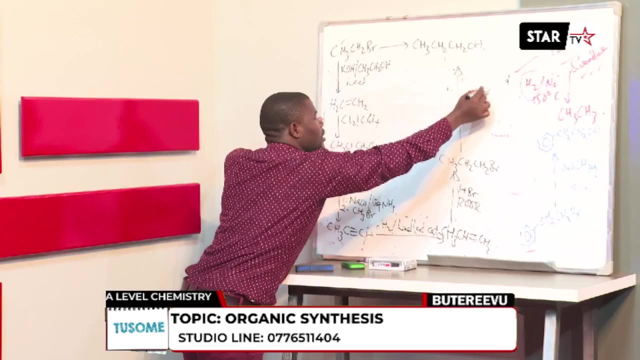 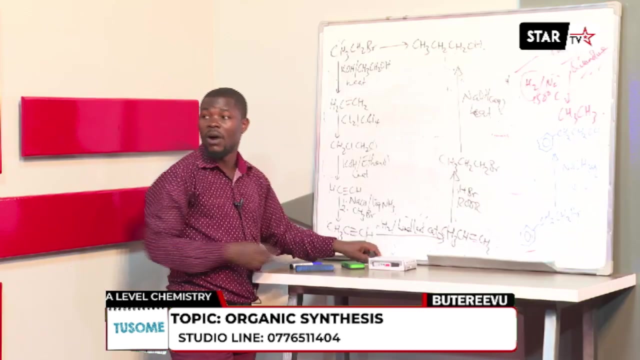 And then uses antimaconic off. If you want to the bromine here, use antimaconic off. That student is getting CH3CH2, CH2 bromine And then uses sodium hydroxide and the student heats. That student is very wrong because he's violating our point. that I've been 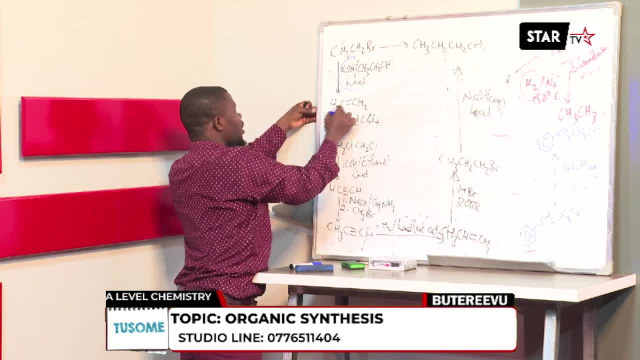 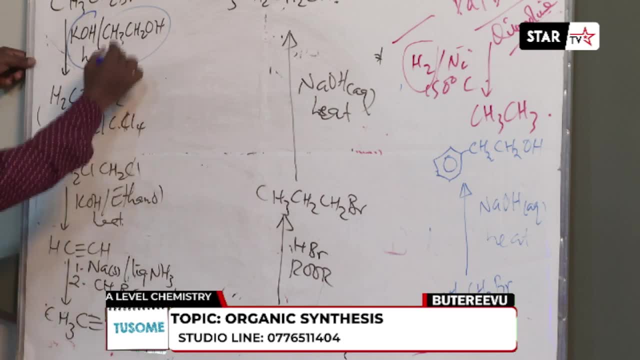 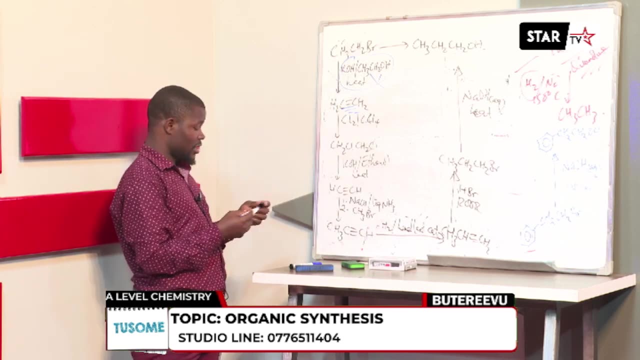 talking about why This step here will never give you a thiene as the major product. The rest of the steps are very fine, but the first step is wrong. so we look at your work and make you lose marks. yet you've done good work afterwards, so 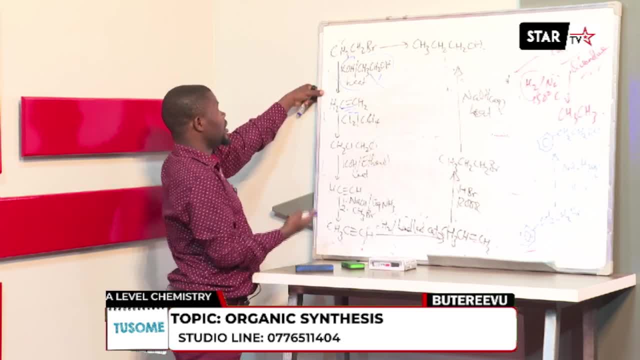 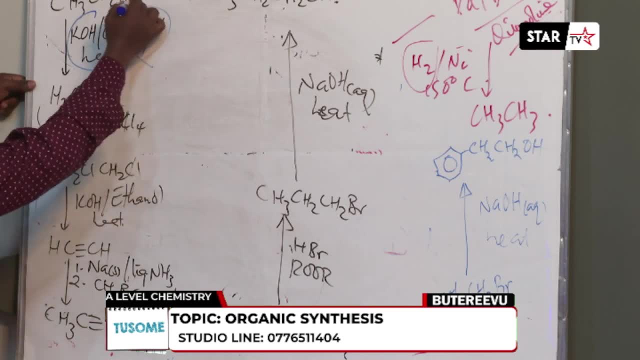 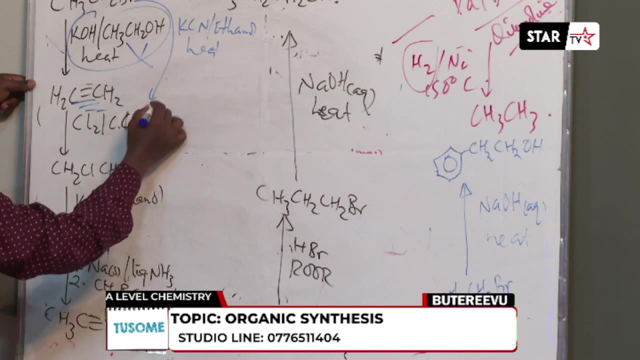 how do you avoid that primary color lights give ethers on reacting the alcoholic, potassium dioxide and heating. so to avoid this, you could go through this route: use potassium, cyanide, ethanol and heat. this will give you, uh, this kind of compound, a nitrile. we call this a nitrile. 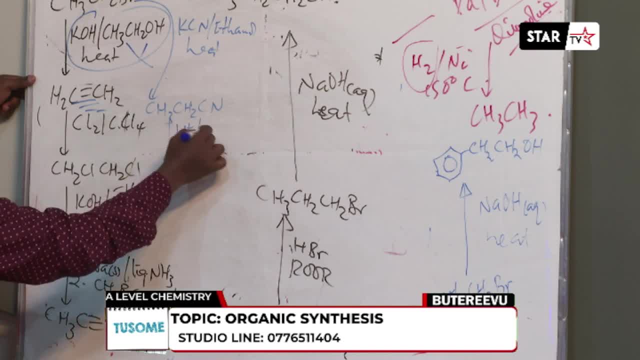 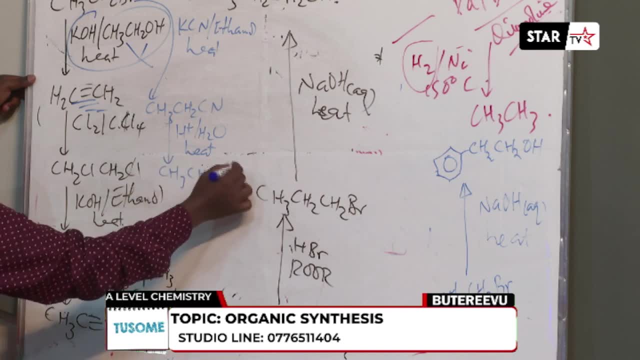 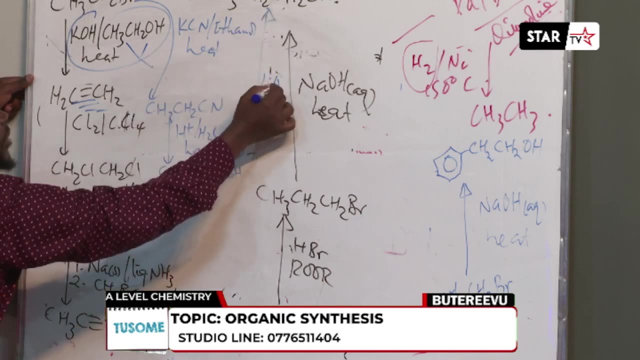 oxidize the nitrile using acidified water and heat. this will give you a carboxylic acid, which is propanoic acid, which you can now reduce using lithium tetrahydridoaluminate in place of dry ether. that gives you 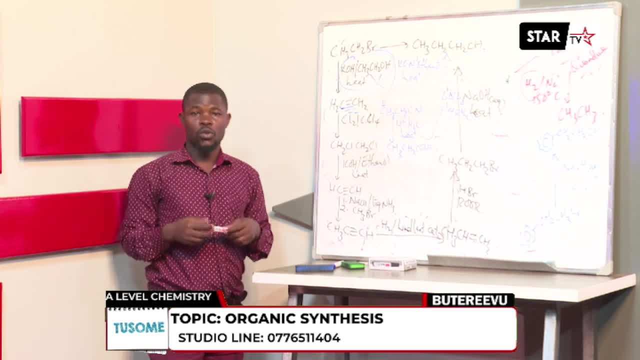 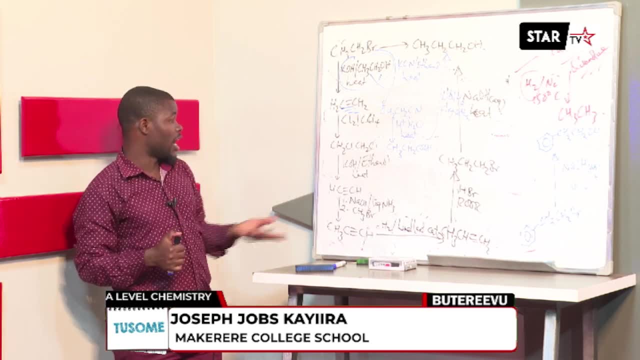 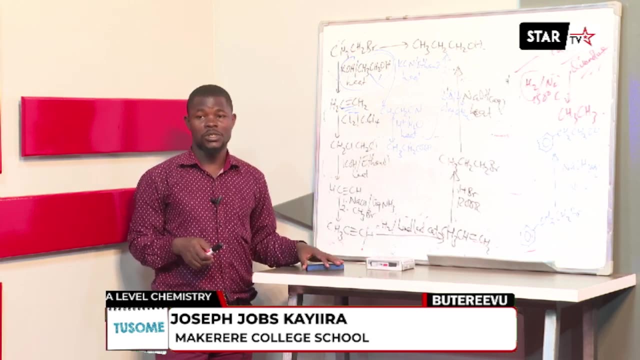 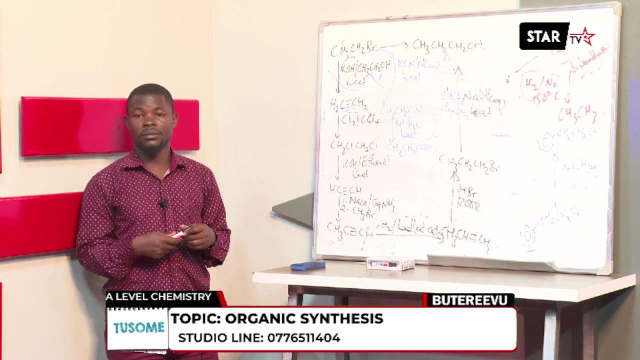 the propano, so that's the best way we could do that. thank you, viewers, for attending this session. we can now welcome questions. for those of you viewing from home, if you have any questions, you can call in the studio line and then present your questions. i'll be answering them. 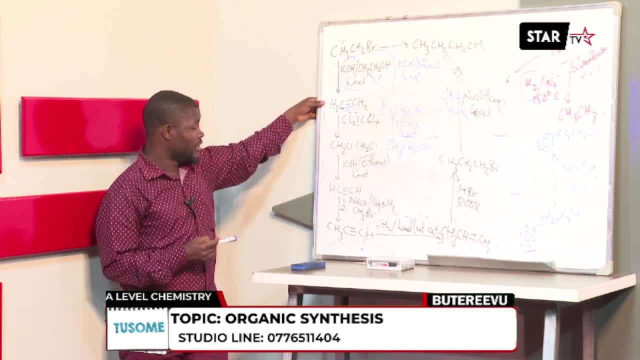 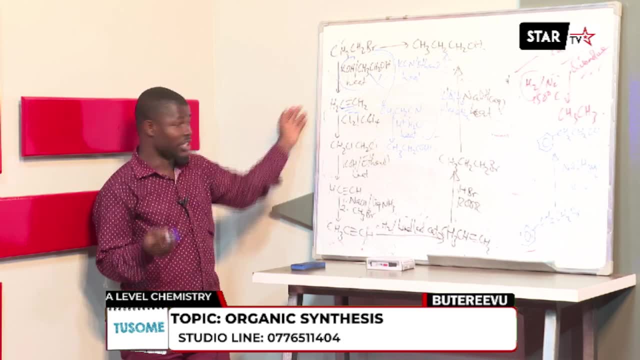 you can call in as you're listening to the program and you can also think of other issues. we shall do more of the synthesis in our proceeding lessons. after this shall always be doing some synthesis. i'll give you the do's and don'ts. when we complete it, then we shall be. 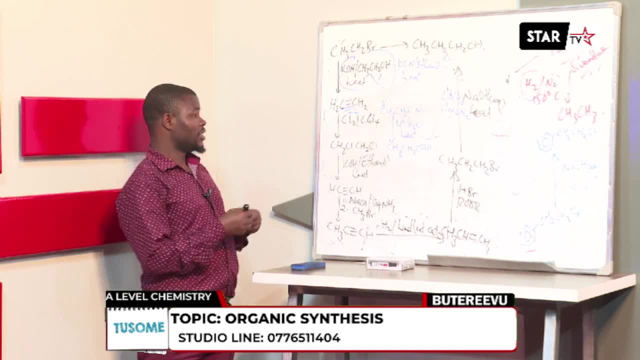 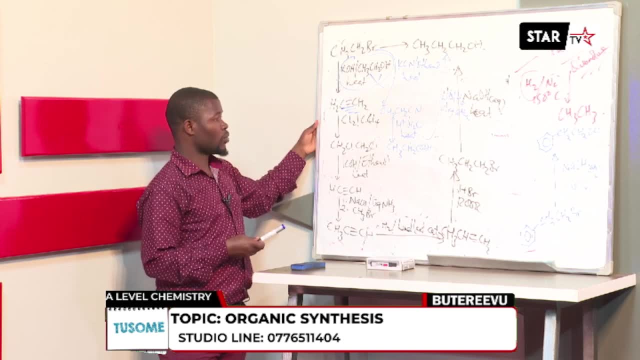 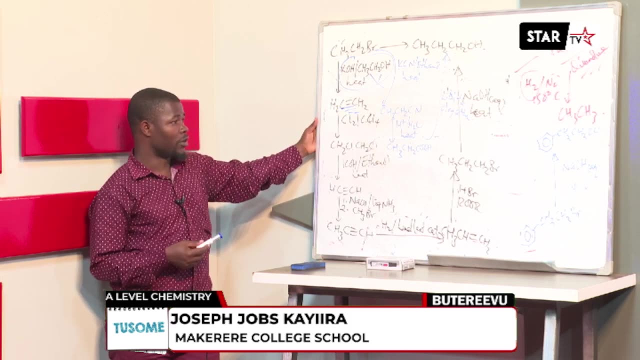 able to see what next we can do. okay, very much. thank you very much for viewing um. you can inbox me the questions on our whatsapp group or you can contact me via my email. Well, thank you for viewing our program this summer. We once again meet next week.